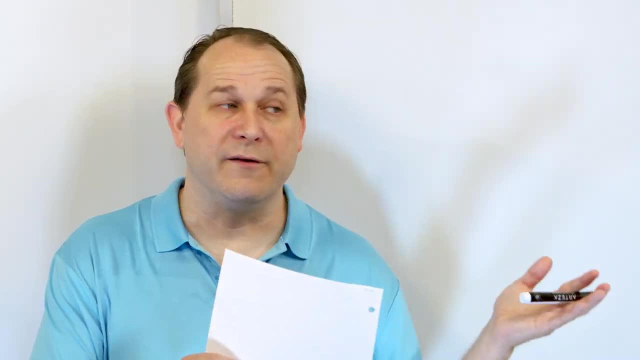 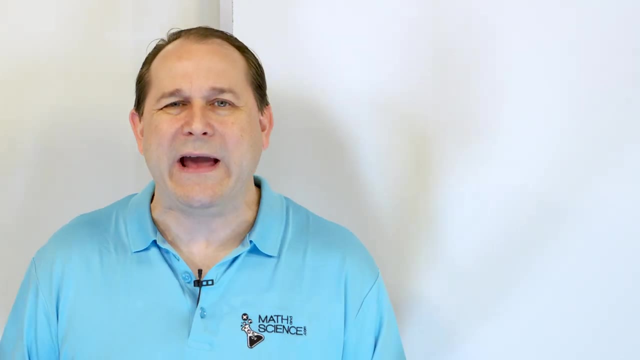 anything wireless and then also physical theories of gravity in many cases, and also in theories of matter, electrons, protons, photons of light hitting you, they're all wave theories. So when you get into higher level stuff you start talking about sines and cosines, And I am 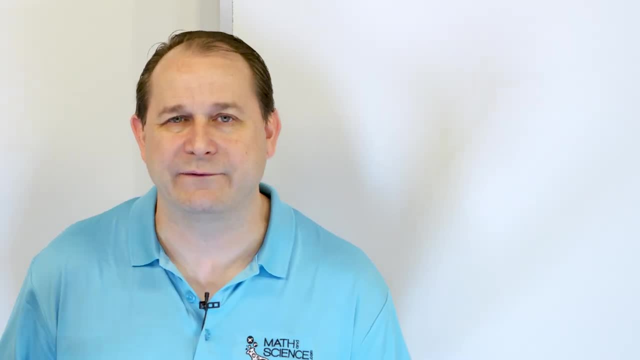 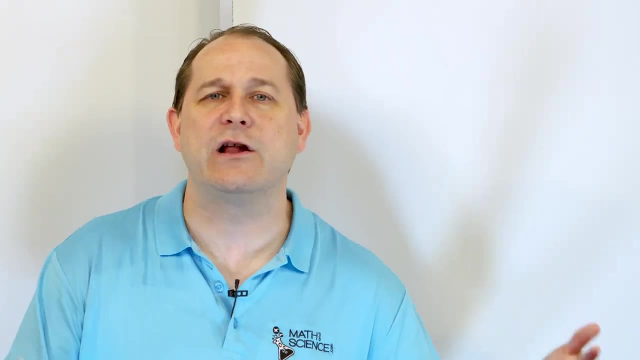 simplifying it, It's not just sines and cosines. There are other aspects that we have to talk about later, But fundamentally this wave- shape, sine and cosine- comes back over and over again in quantum mechanics and technology and so on. 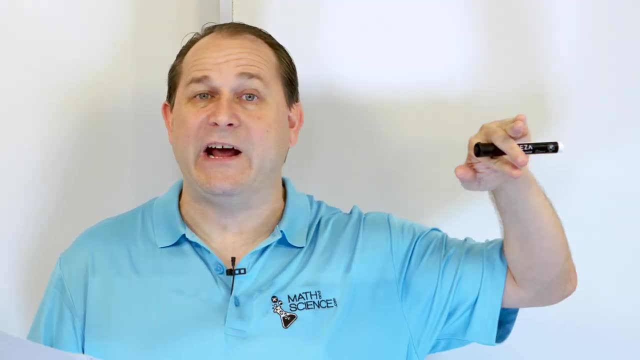 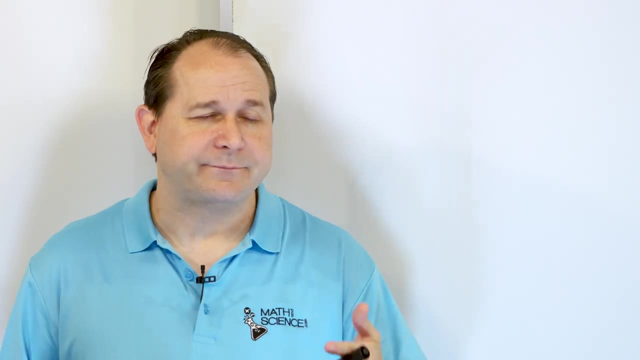 So what we have to do, though, is learn how to take that basic shape of a sine and a cosine function and change it or shift it around, make it look a little different, Because in real life, you have waves of all different shapes and sizes, so to speak. So what we're going to do is a 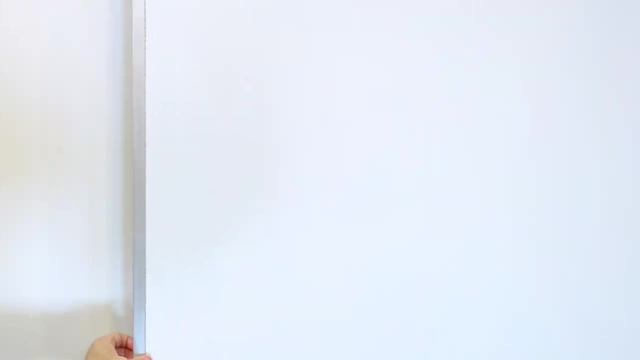 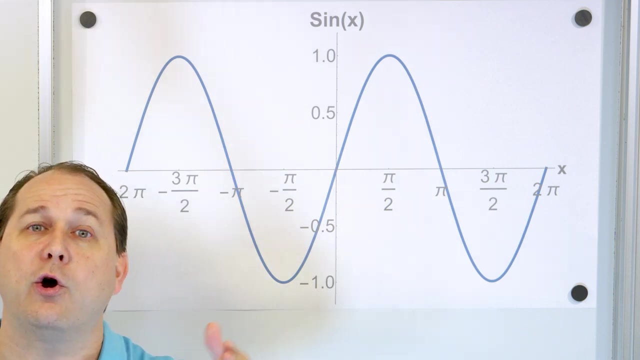 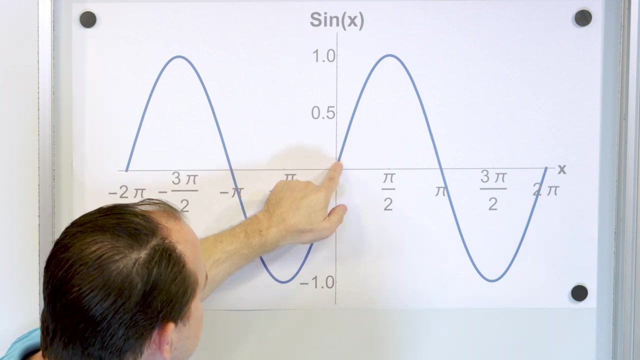 computer demo to show you graphically how that works. But before you do that I want to jump into a little bit of math. So if you don't already know this, if this doesn't look familiar, then go back to my graphing lesson on sine and cosine. So the sine function is a wave that starts at zero. 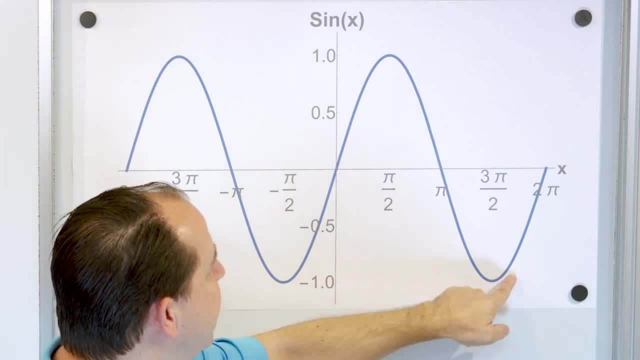 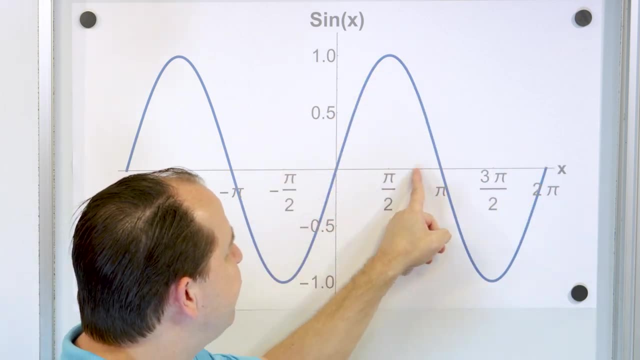 the origin. it goes up to a maximum of one, down to a minimum of negative one and then it goes back to the starting point. So this is called one period, And you can see, the period when it begins to repeat itself is two pi. So that means when x gets to two pi, the wave begins to start over again. 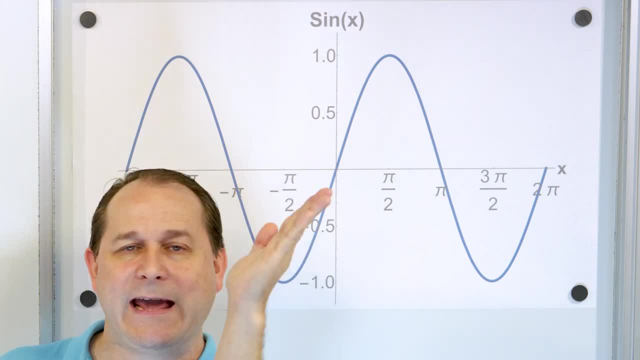 And the reason that happens is because x is the radian angle And so when it goes to two pi it means it completes one whole circle in the unit circle. If you go a little past two pi, then you're just retracing the same angles over and 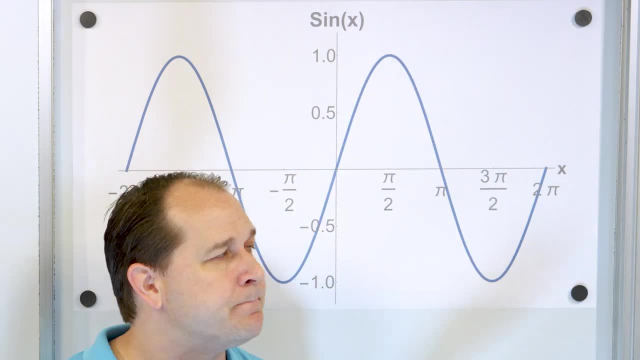 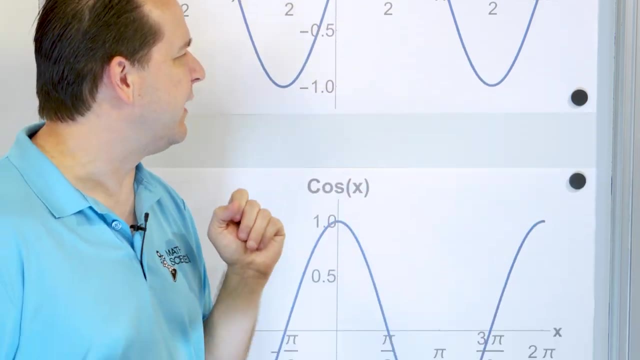 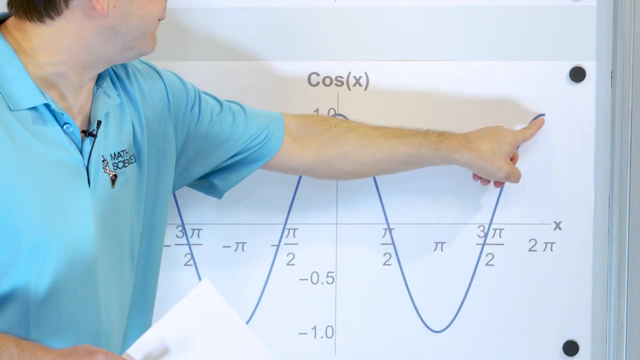 over again. So the thing continues to go up and down, up and down forever. But the thing to remember is that sine starts at zero and then up, down, up. Maximum minimum plus minus one. Cosine starts at a maximum and it goes down to a minimum again of negative one, and then back up. 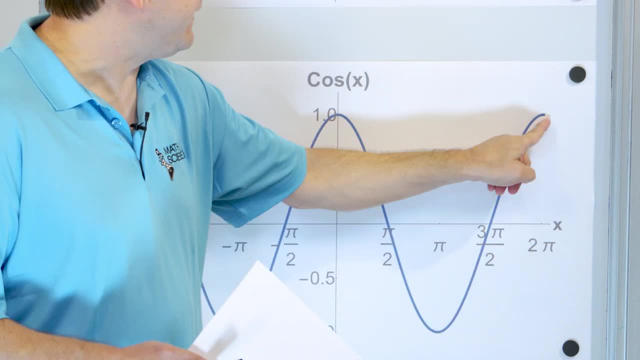 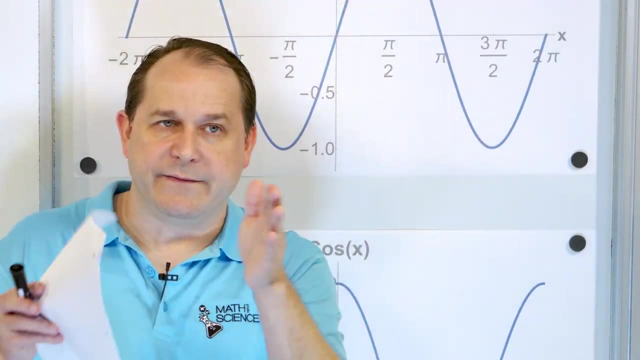 to its maximum of positive one. So it starts here and again, it begins to repeat, or it will begin to repeat right here. Notice that it also has a period. Period is the kind of like when the thing begins to repeat again of two pi. 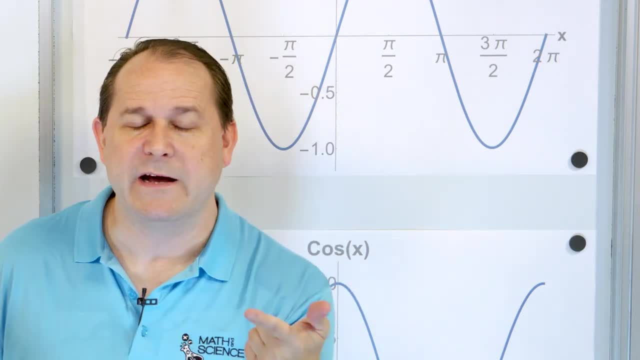 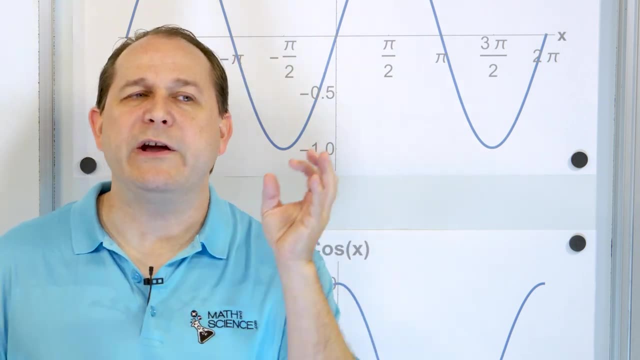 All right. So sine and cosine have the same shape, They have the same period, They have the same maximum and they have the same minimum, plus or minus one. Now, the reason I'm reminding you of this is because when we graph these functions, we're going to start changing their shape a little. 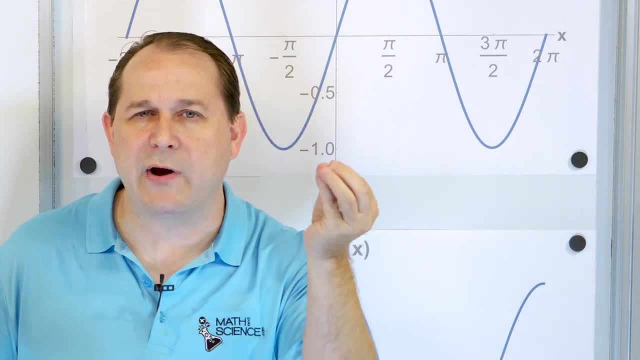 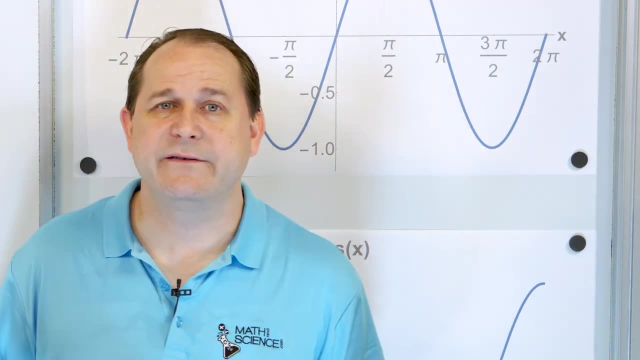 bit. It's important for you to have a baseline function in your brain of what it looks like And you need to be able to draw it. You need to be able to draw it and put it down on paper and commit it to memory. Okay, So starts at zero, goes up to positive one here at pi over two down. 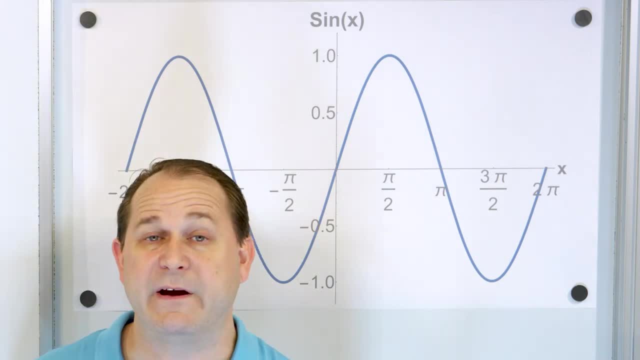 through pi and then up to two pi. That is very important for you to have in your brain, because as we alter the graph, as we change it a little bit, it's going to be always in reference to what we started with. All right, So what are we going to do? First of all, we said: this is one period when 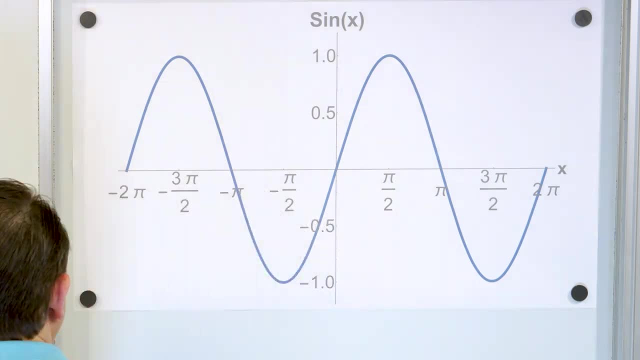 it begins to repeat itself. We need to define the number of times that it repeats itself. So we need to define the number of times that it repeats itself. So we need to define the number of times that it repeats itself. So we need to define some additional terms, This distance from here, all the way. 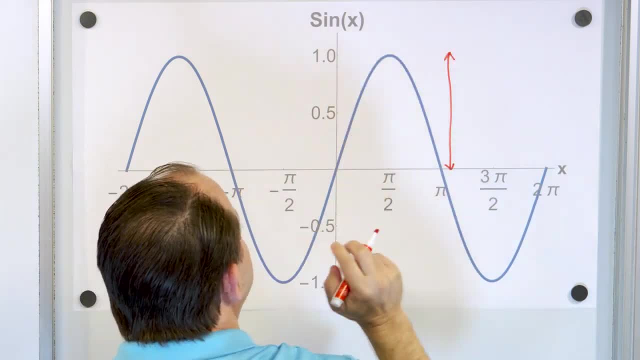 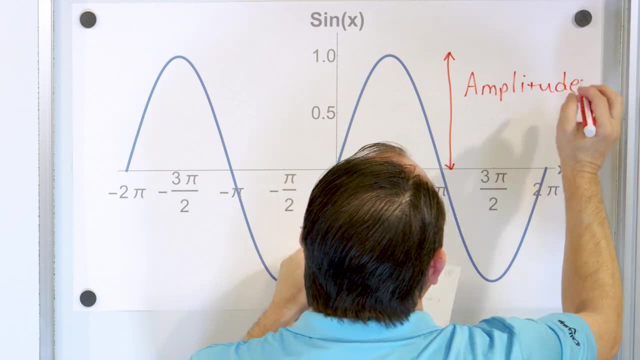 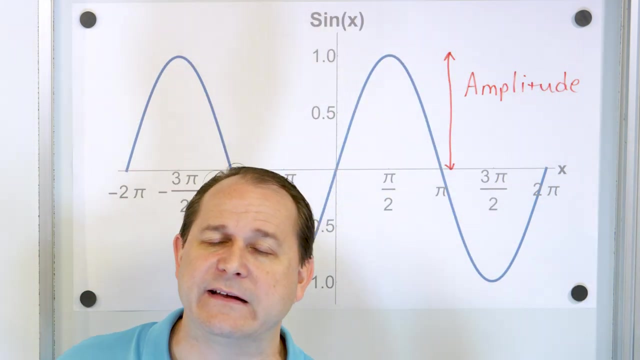 down to the x-axis, from the x-axis all the way up to the maximum of the curve. it's called the amplitude. The amplitude- You may have heard the word amplitude- Amplitude- is the height of the wave. If you're at the beach, you're watching the waves roll in. If you have a very high wave, we 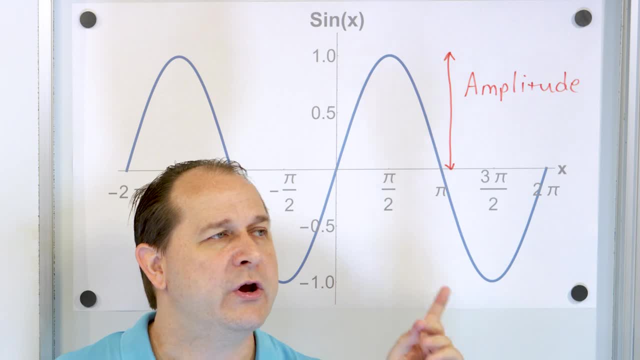 say it's a higher amplitude, A low wave is a lower amplitude. So one thing we're going to learn how to do is how to change this sine function to make it a higher amplitude. So we're going to learn how to do is how to change this sine function to make it a higher amplitude, A taller wave or a smaller? 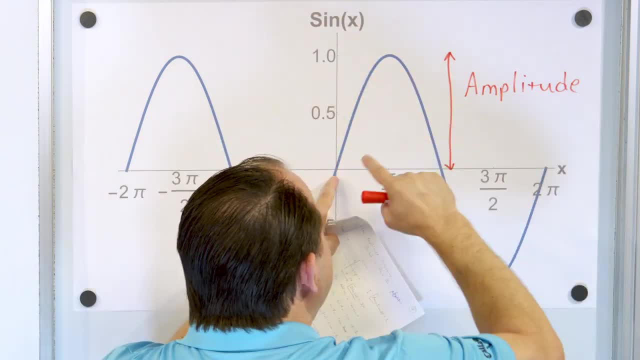 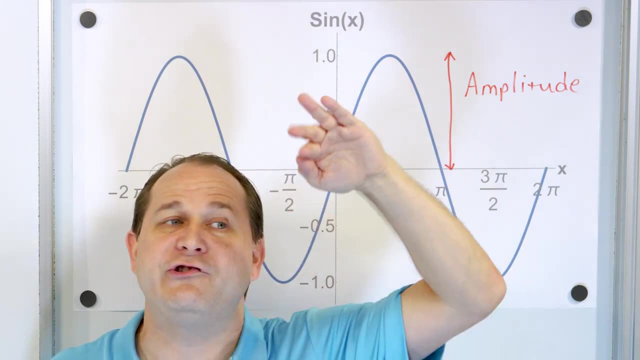 wave. We're also going to learn how to make it wiggle faster. Right now, the period's 2 pi, but what if I put a bunch of wiggles in here? Then the period of that function is going to be different than 2 pi, So we're going to learn how to change its period, which is the same thing as changing. 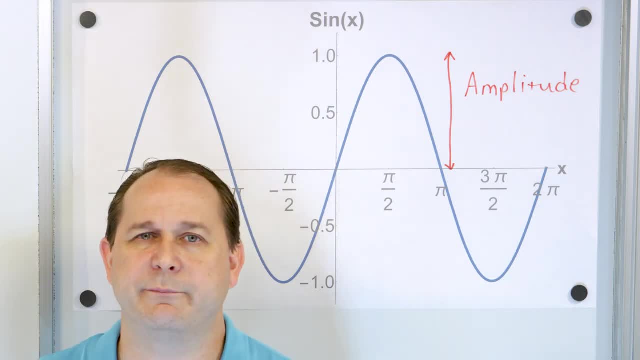 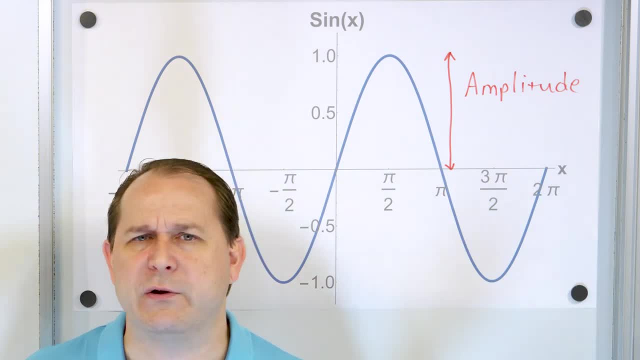 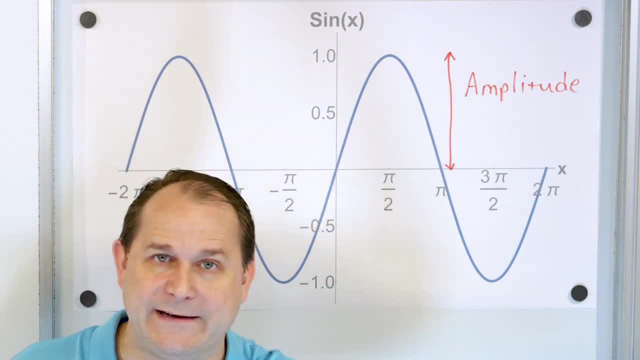 So in a wave, if it has a high frequency it wiggles a lot. okay, Higher frequency, higher wiggles. right Right now there's only one wiggle up down up over here on the right side, but I. 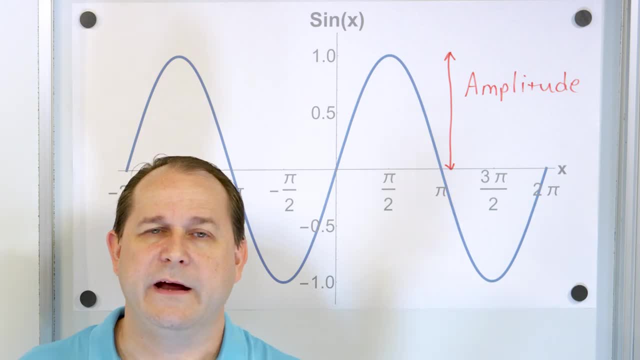 can put a thousand wiggles in there if I want to, and so they would have a higher frequency. So the amplitude is the height of the wave from the x-axis up to the top, and the frequency and the period. both can measure how much wiggling is going on here. essentially right, And what else are we? 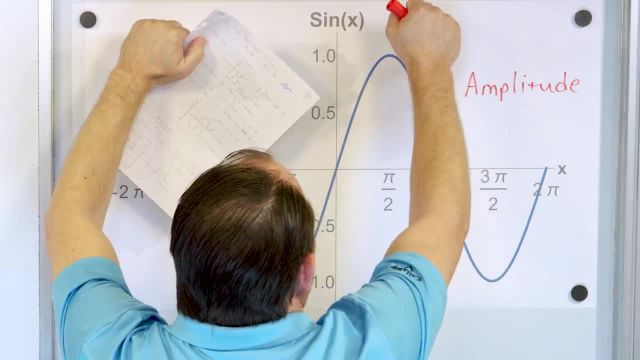 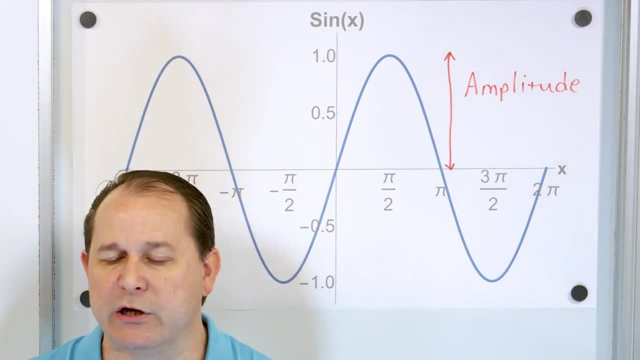 going to learn how to do. We're going to learn how to take this graph and shift it up and down on the y-axis, and then later, in another lesson, we're going to learn how to take the graph and shift it left and right along the x-axis, But right now we're going to learn how to change. 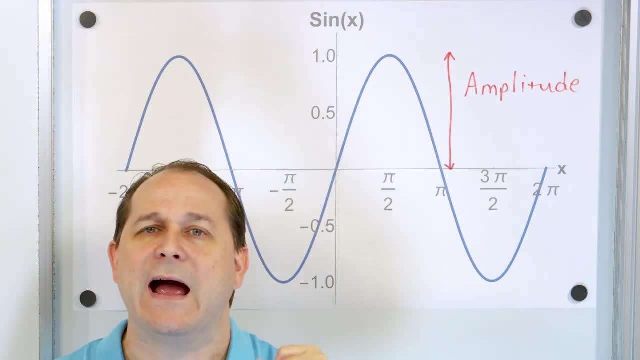 the wave's period, which means change how many wiggles we got in there, how to change its amplitude and then also how to shift it up and down as well. So before getting into the theory on the board, let's do the computer demo with a few things. Let's do the computer demo with a few. 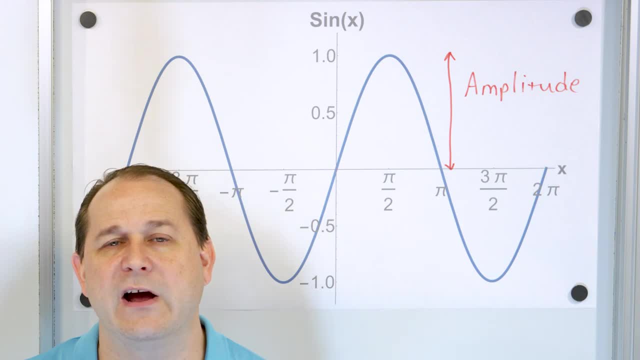 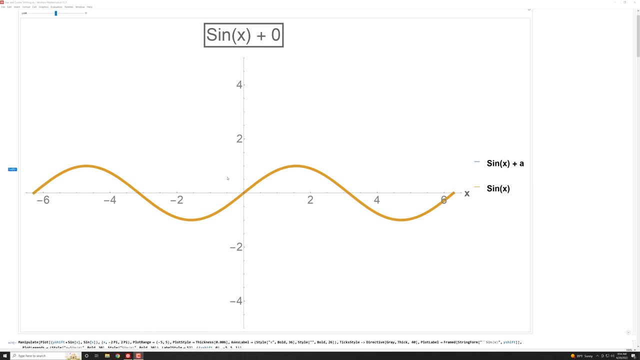 minutes, You'll understand brilliantly how this works. It's very much worth your time, so let's go ahead and do that right now. Hello, welcome back. So here we are at the computer demo. Here we have a sine wave. We're going to do the same thing with cosine, in just. 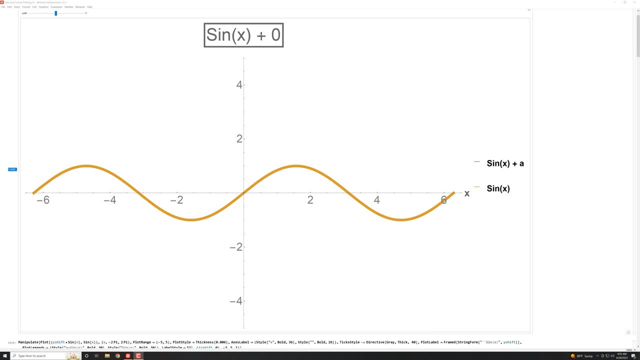 a minute, but here is a sine wave. Notice what I've done is it's sine of x, but I'm going to add to it a number, and right now this number is zero. So since I'm adding nothing to it, then all. 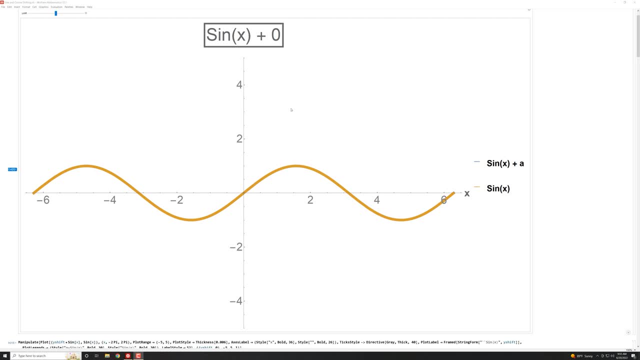 I have here is a sine wave. So what's going to happen is, if I want to shift this thing up or down along the y-axis, what do I do? Well, if I add a 1 to it. so now I have sine of x plus the number. 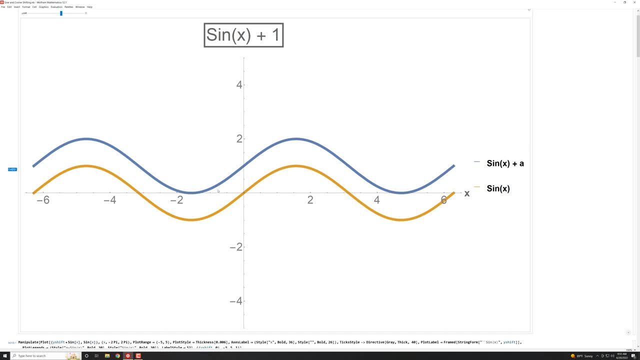 1, then I have a blue curve which looks exactly to be the same shape as the curve below it. It's just shifted up one unit. Notice that the original orange curve only goes up to a maximum amplitude of 1, but the blue one goes up to a maximum amplitude of 2, and the minimum is now at zero. 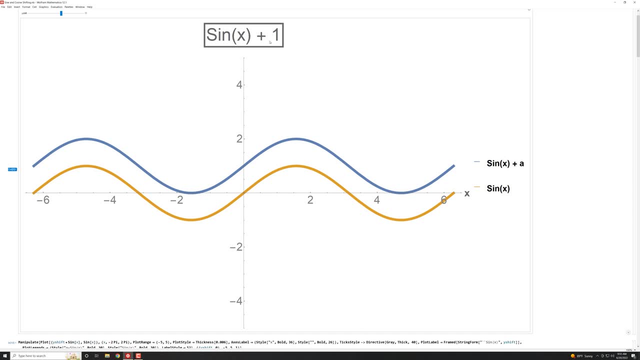 So it's the same height, The wave is the same height, It's just that the entire thing is shifted up by 1.. So what you do is you compute the value of the sine, at whatever angle you're, at, Whatever number you get back for the sine, you just add the number 1 to it, and that's what you. 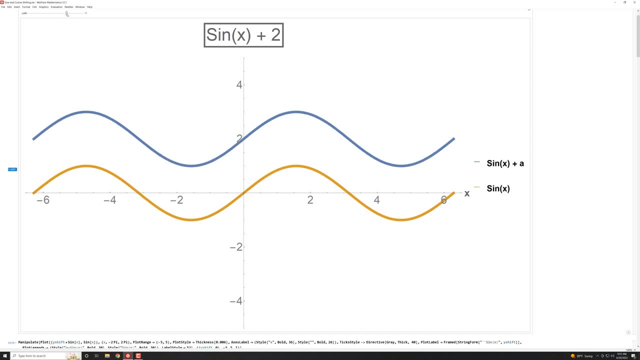 plot on the graph. So if I change that number 1 to a number 2, then I shift the entire graph all points up two units. So the maximum goes up, and the minimum goes up, and the baseline here also goes up, So they all go up like this. So you can see what happens if I shift it up 3 or even 4. 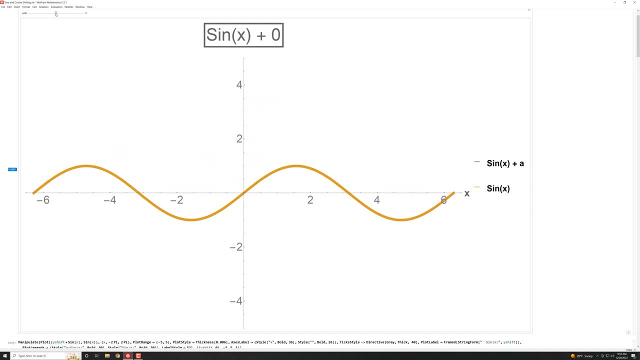 units. okay, So let me go back down to zero. What do you think is going to happen if I change that constant over here to negative 1?? So you can think of it as a plus minus, or you can think of it as sine of x. 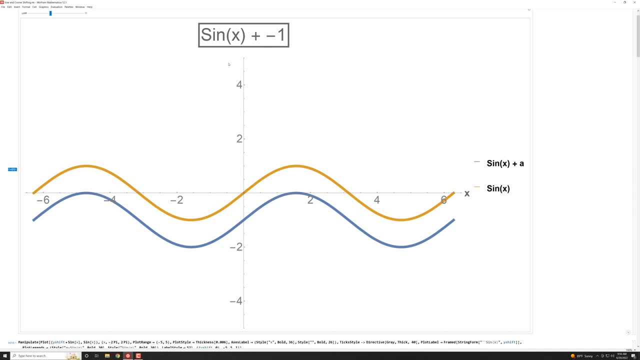 minus 1, and that's going to shift everything down. You compute the value of sine, of the angle, and whenever you get back you subtract 1.. And you do that for every point. So the shape is the same, but the thing is shifted down. So to answer the question, how do I shift a sine or cosine up or 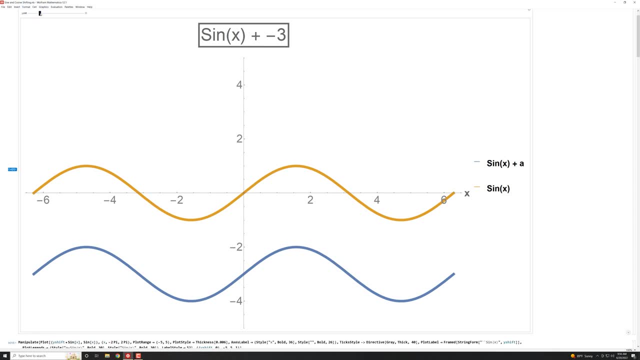 down on the y-axis, But changing nothing else. I just add a number on the outside. Notice, adding this number is on the outside of the sine function. Just add or subtract it and that's going to shift the thing up or down. All right, that's how to shift it up or down. The next thing we need to 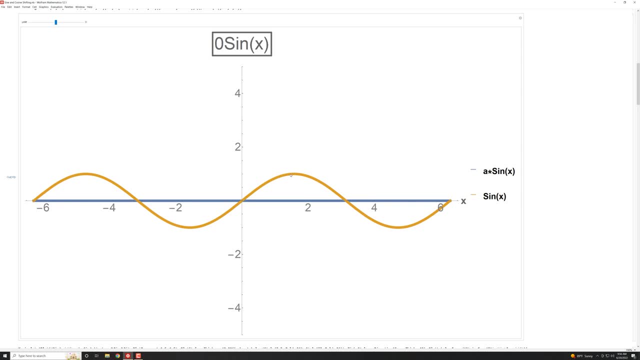 talk about is how to make the wave taller, In other words have a higher amplitude. So notice the gold graph here. This is number 2, so this is 1.. It has an amplitude of 1.. The basic sine function and cosine function has a maximum of 1.. Notice I have 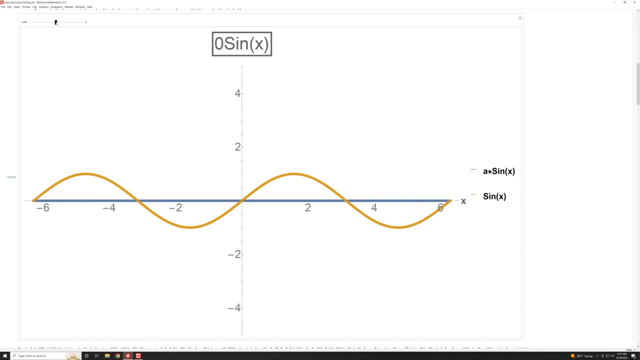 a 0 here on the front of the sine. What if I change that to 1?? So 1 times the sine of x, that's the same thing as sine. So we have exactly the same curve here. But what if I change it to 2? 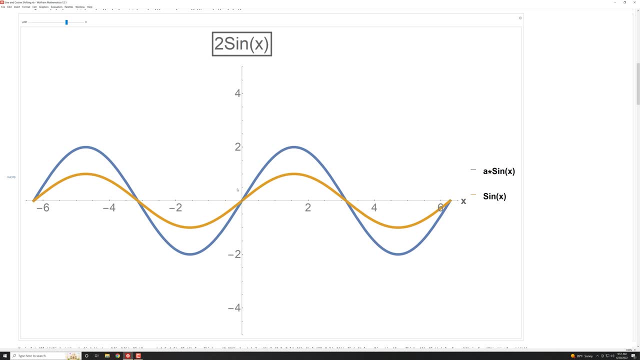 times the sine of x. This is what you get. You see how the blue curve is the altered curve. here It's 2 times the sine of x. Notice that the crossing points are the same. We cross through 0 at the same place. Here is the maximum of both of these functions, and they both occur at the same. 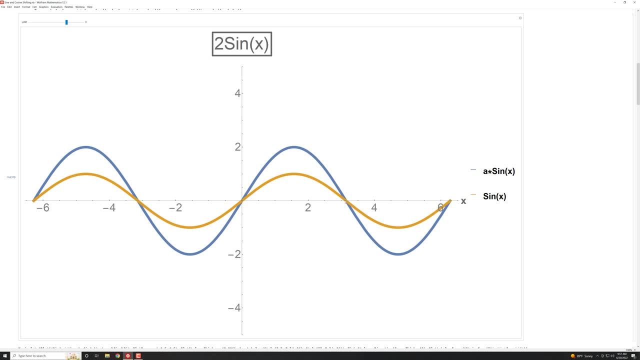 spot, They cross down through the axis, again at the same spot, They have a minimum here at the same spot and they go back up at the same spot. So these have the same period and all the same crossing points. The only difference is this blue curve goes up to maximum of 2 and minimum of minus 2.. 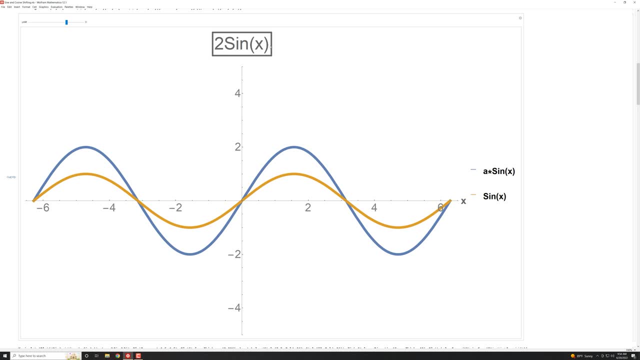 Why do you think that is? Because if you look at the function sine of x, it's only going to give you numbers back between plus or minus 1, because the unit circle can only go between plus or minus 1.. So the sine is going to give you a maximum of 1 and a minimum of 1.. 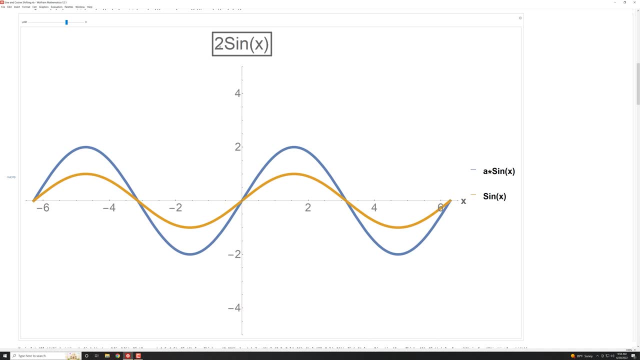 So the sine is going to give you a maximum of 2 and a minimum of minus 1.. So, whatever I get back from the sine calculation, I just multiply it by 2.. So the maximum it can go would be positive 2 or. 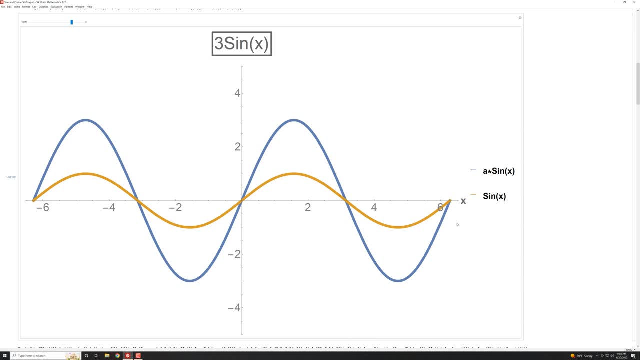 negative 2.. What's going to happen if I change this to 3 times the sine of x? It's exactly the same crossing points, but now the maximum goes up to 3 and the minimum to minus 3.. And, of course, 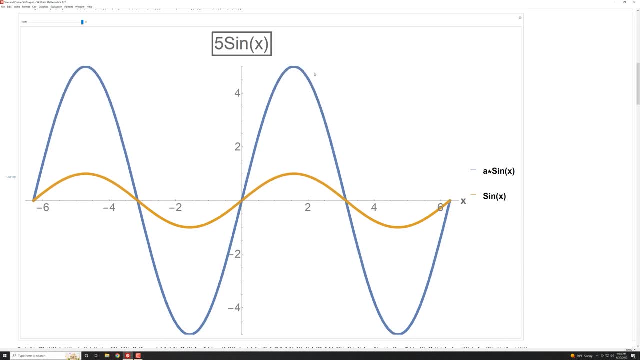 if it goes to 4, maximum of 4 and minimum minus 4.. And if it's 5, maximum 5 minus 5.. So you can play with this and see that to make the amplitude higher or lower, you just put changes in the. 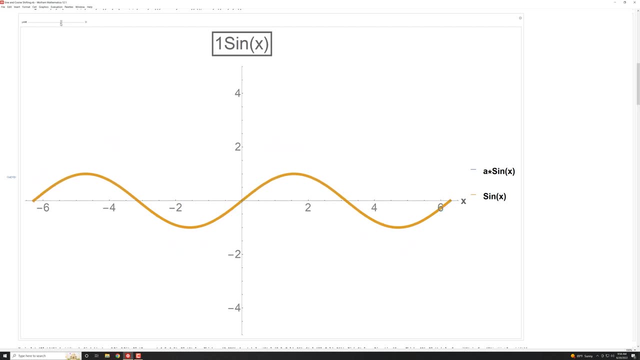 number that's out in front. Now what do you think is going to happen? Here is 1 times the sine of x. What if I make it negative? 1 times the sine of x? Look at what happens here. So now what's going on? 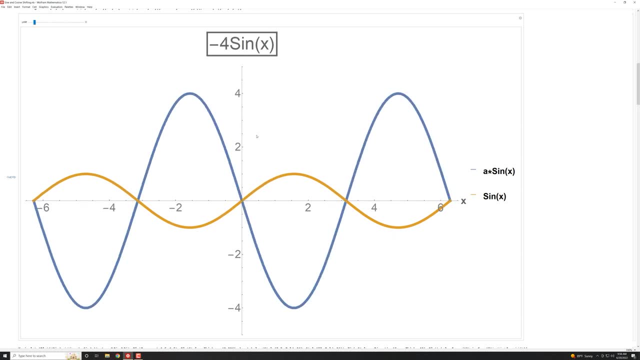 is, or if I change it to even negative 2 or negative 3 times the sine of x. Notice that the crossing points are the same, but now the maximum and minimum they're kind of like opposite of each other. Why? Because the sine function returns either a plus 1 or a minus 1.. Let's 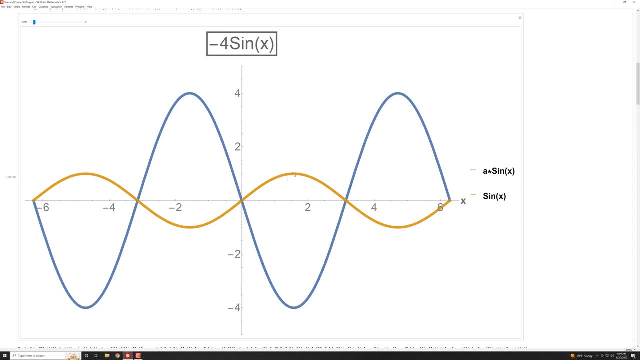 say that it's returning a plus 1. That means we're here on the graph returning a plus 1.. Well then I multiply by negative 4.. So at that moment or at that angle, I'm really getting an answer of negative 4, because it's negative 4 times 1.. That's why it flips it down. So when you see a 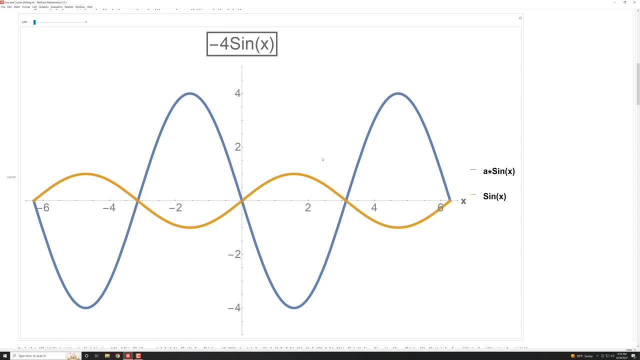 negative sign in front of a sine function. it's going to like: flip the graph over and all of the positive points become negative and all the negative points, like over here, become positive. So we're changing the amplitude and we're also flipping the thing upside down, so to speak. 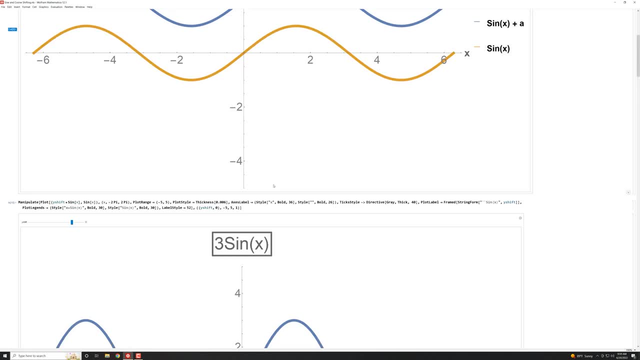 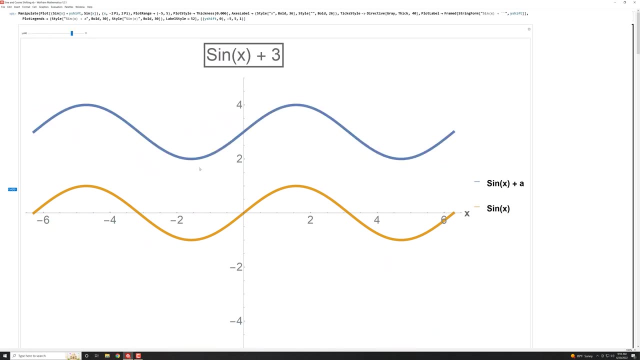 So that's how you change the amplitude: You change the number out in front. So just to recap so far: to shift a graph up and down, you just change the number that you're adding to the whole function, like this. And to change the amplitude or the height of a function, you just change the number. 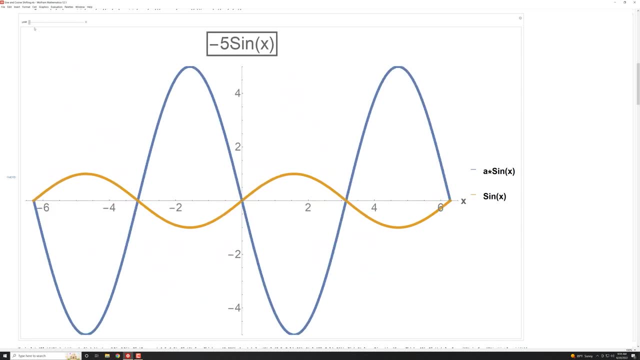 that's out in front, And if it slips negative, then it's going to. it's going to invert the thing, but it's still going to behave the same way. Now let's take a look at what happens. Everything so far this has been outside of the sine function. The 4 is on the outside, The 3 over here. 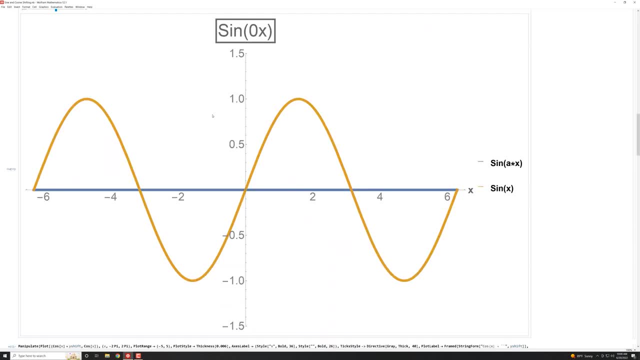 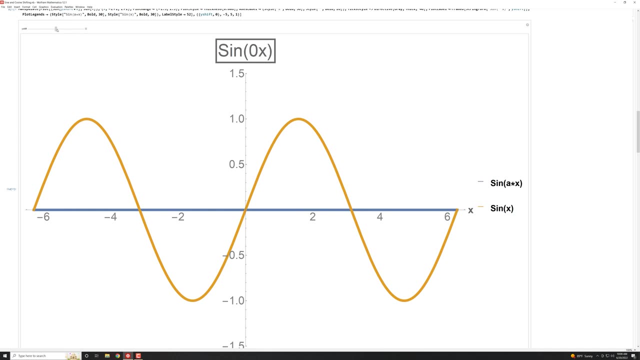 is on the outside of the sine function. Let's see what happens when we change a number that's on the side of the side. So I have 0 times x here. So what I can do is change this to 1 times x And 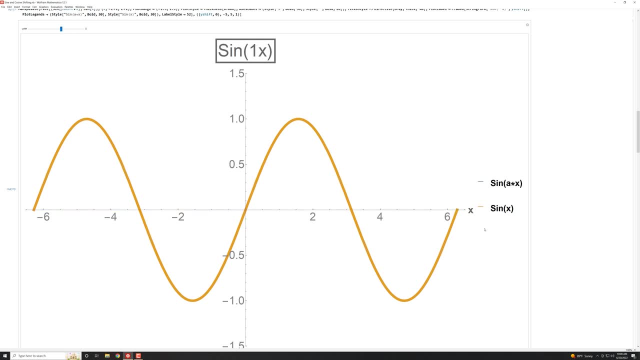 what are you going to get Sine of 1x right? So that's just sine of x. That's the same gold curve we always have. Everything is exactly the same as it is Now. what does it mean if I change that to? 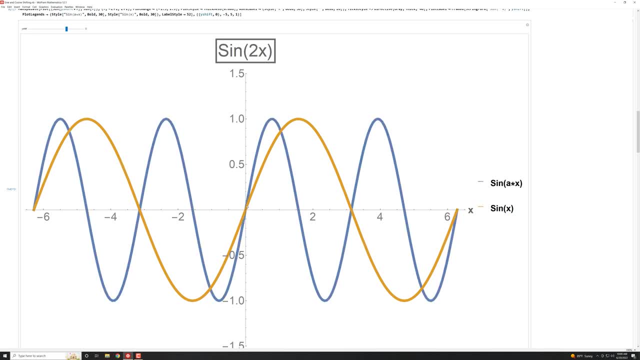 a 2?? Notice. what happens here is I have a blue line that now is wiggling twice as fast. That means it has a frequency. Frequency is how fast it's oscillating, essentially. So you can see, if I have a 2x, I have more wiggles in the blue curve. If I have a 3, sine of 3x, I have even. 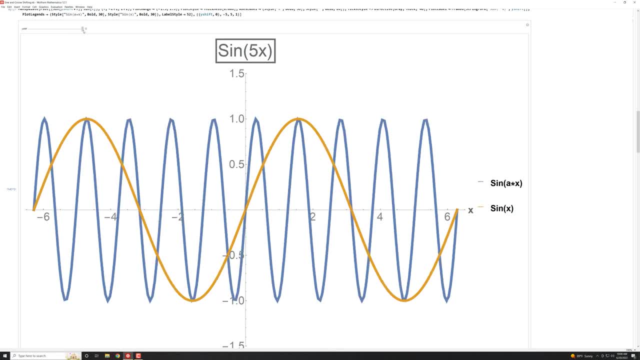 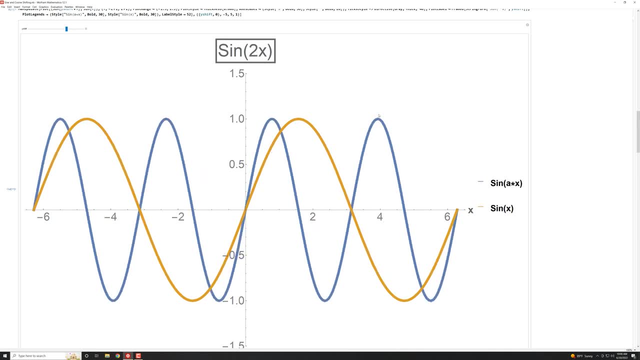 more wiggles, And if I have a 4 or even a 5x, I have even more wiggles in the blue graph. But notice the pattern of what's going on here. Let's go back down to 2 right here. Okay, Actually. 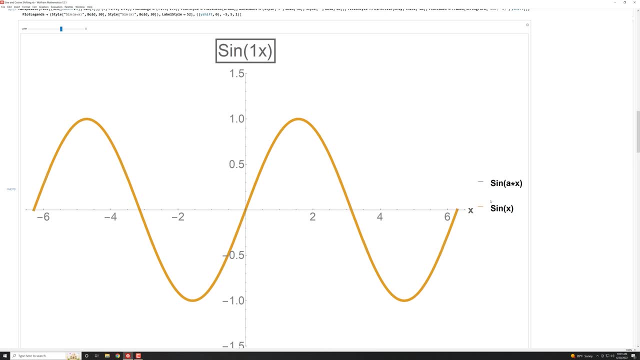 let's go to sine of x. What is the period of this sine function? This is 6,, this is 6.28.. So this is pi over here. So the period of the sine function is sorry: 2 pi, 2 pi radians. 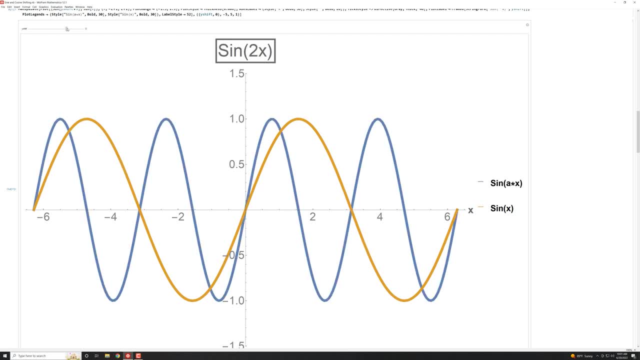 The period when it begins to repeat is 2 pi. If I change that number to 2x, what actually happens is notice the blue curve. I have one complete cycle here and then I have another complete cycle here, So I have two complete cycles that exist. 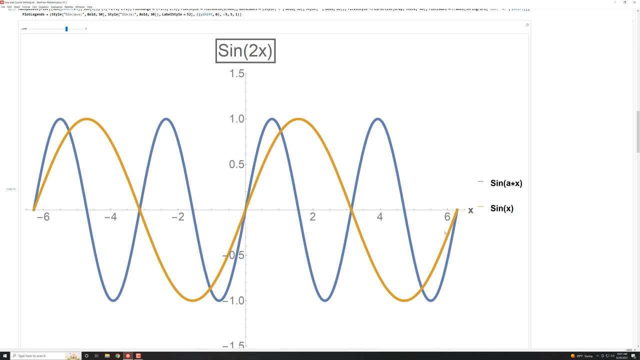 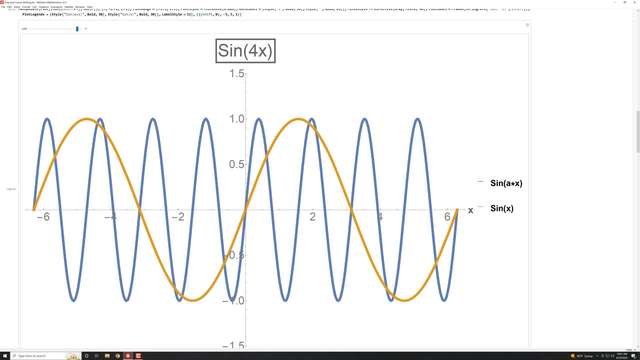 inside of the same period that the original function has, And if I make it sine of 3x, I now have three full oscillations. There's one, there's two and there's three of them exist in 2 in a 2 pi region. If I make it sine of 4x, I have here's one and then here's up and down two. 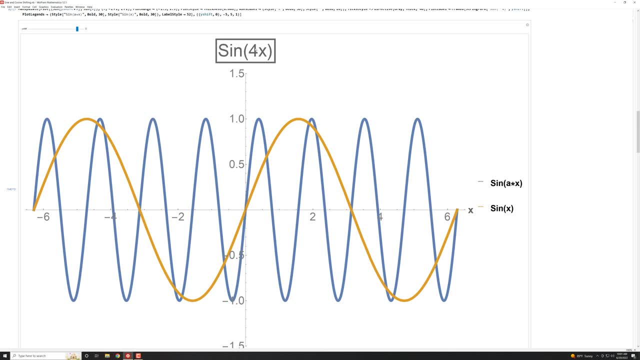 here's three, here's four periods. So the number that you have here. if you make this number bigger, then you're increasing the number of wiggles, so to speak. in the function We say that you're increasing the frequency. This blue curve is oscillating four times faster than the gold curve. 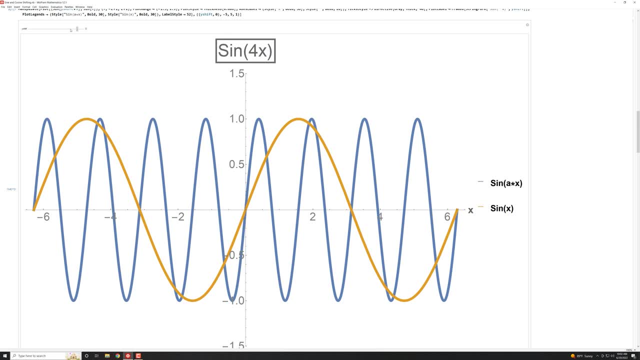 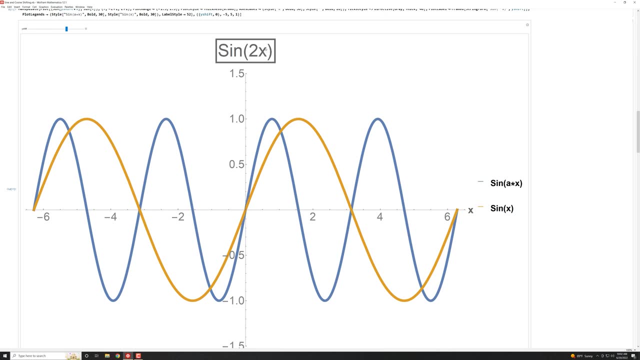 And we're going to talk on the board why. but I can just tell you briefly why in a second. If you put it to 2 right here- oh sorry, that's sine 1x to 2 here- then what's going on is: if you put a value for x here of pi, 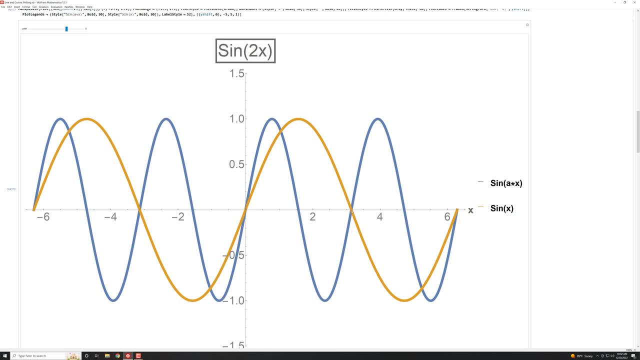 pi radians on the gold curve is right here, That's 3.14.. That's only half of a cycle. But if I put pi into this function then I'm taking the sine of 2 pi, And 2 pi means I've gone all the way around the unit circle. So for the blue curve, 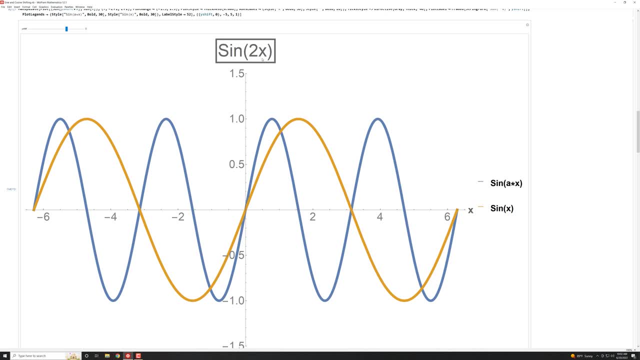 then I've already completed one cycle when I only have gone around half as far half the unit circle Pi radians. So the reason why you're going and oscillating faster is because when you put a number in front of here you kind of make you're kind of like changing the angles inside the unit circle. 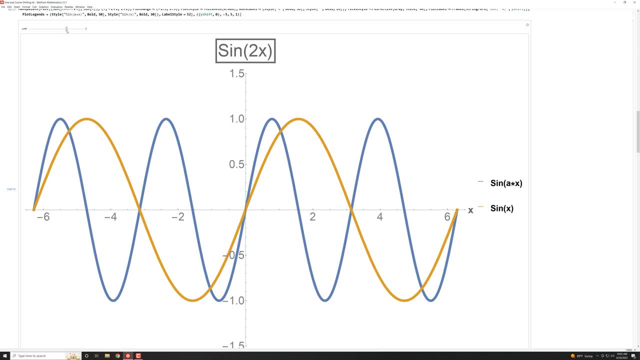 twice as fast as before, Because if the number here inside of here is sine of 1 times x, then of course x can go. you know, pi over 2,, 2, pi over 2, and so all the way around to 2, pi And. 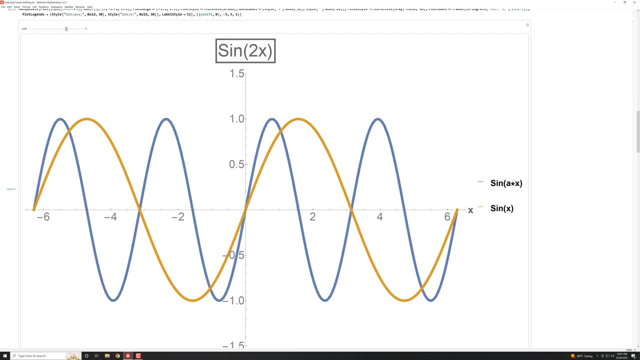 then you complete one cycle in 2 pi. But if I make that a 2, then x only needs to get to pi radians so that I take the sine of 2 pi. That means I must complete a complete cycle of this thing when x. 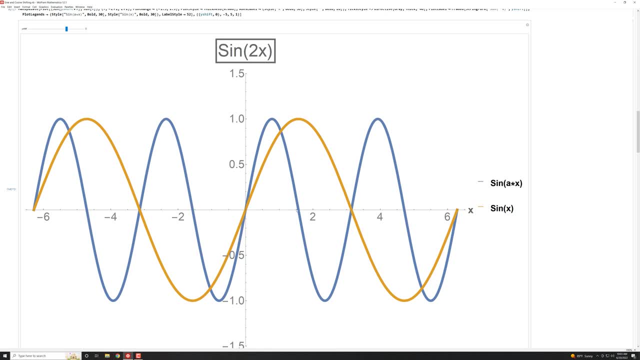 only goes half as far to 2 pi to pi radians, And so you can see that when I get to 2 pi I've completed one cycle. So the bottom line is, whenever you have a number in front of the variable that's inside of the sine function, the number here is telling you how many complete. 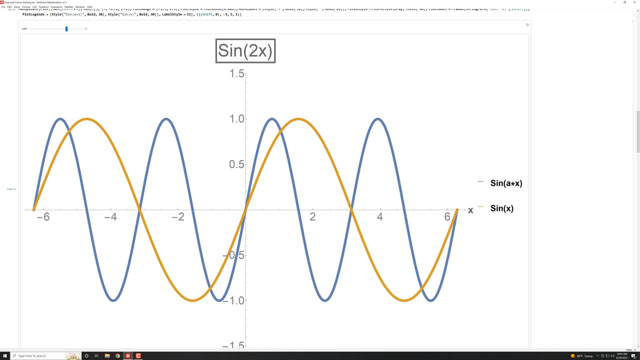 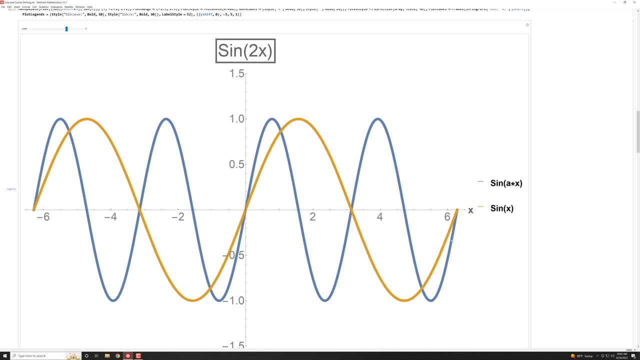 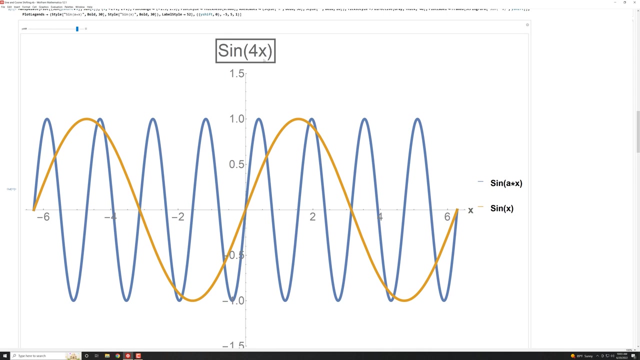 2 pi. So since there's a 2 here, this function has two cycles inside a regular sine function. This one has three cycles, three periods, inside of a normal sine function And this one has four complete cycles that live inside of here, because this thing is changing angles four times faster. 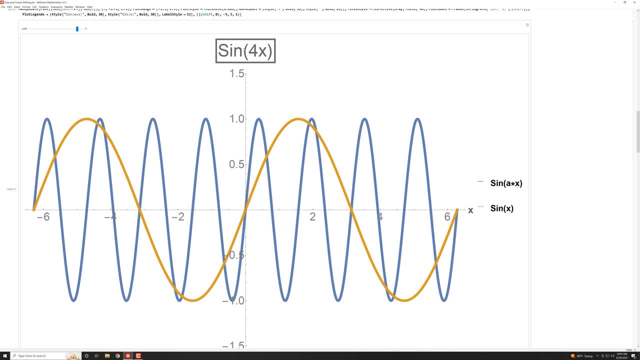 The x variable doesn't have to go up as much in order to make the inside of this thing go all the way around the unit circle very, very fast, And that's why you're getting all these cycles here, because of that. I mean, just think about it: If I put the value of 2 pi in for x 2 pi, then 2 times 4 is 8,. 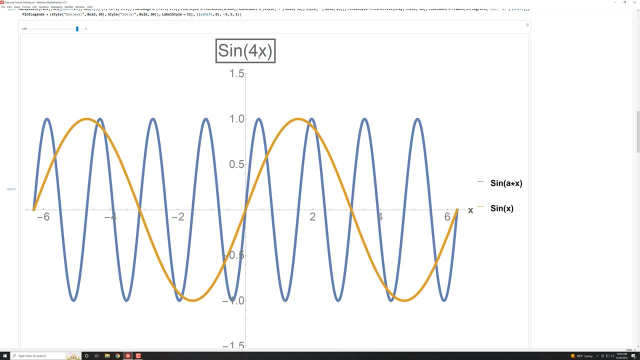 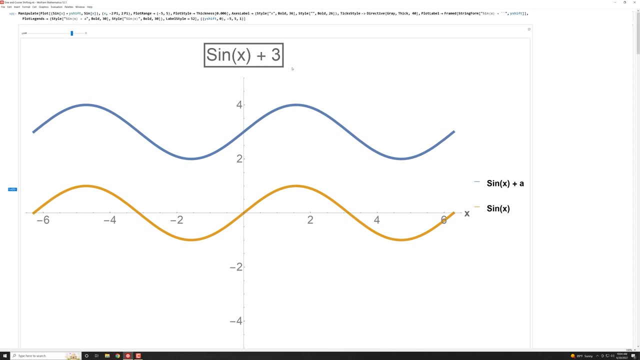 that sine of 8 pi. I've already gone around the unit circle, Remember 2 pi is one cycle. So if I go around 8 pi that's like four complete cycles around the unit circle, whenever the gold curve only goes one time by going around 2 pi. So let me just recap real quick: We have a baseline sine. 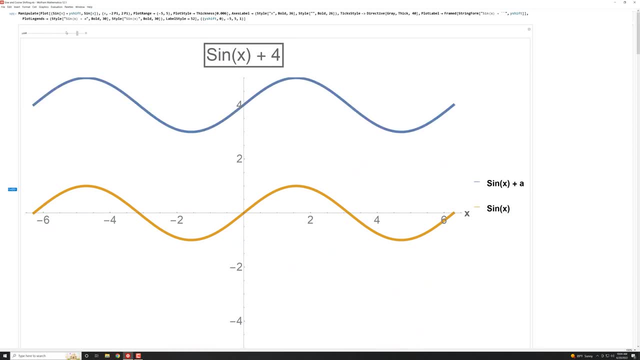 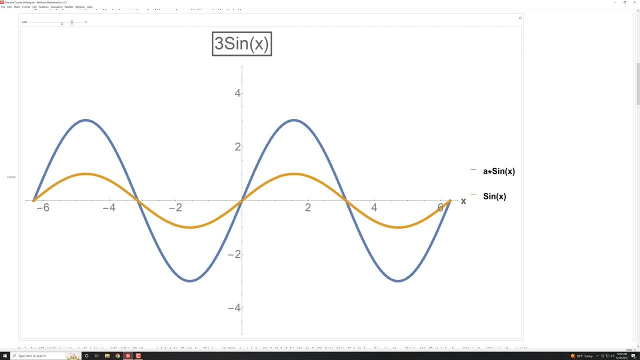 function. If you add or subtract a number on the outside, then all you do is shift the exact same curve up and down. If you have a number sitting out in front of a basic sine function, then it changes the amplitude- higher or bigger or smaller. And if you change the number on the inside, what? 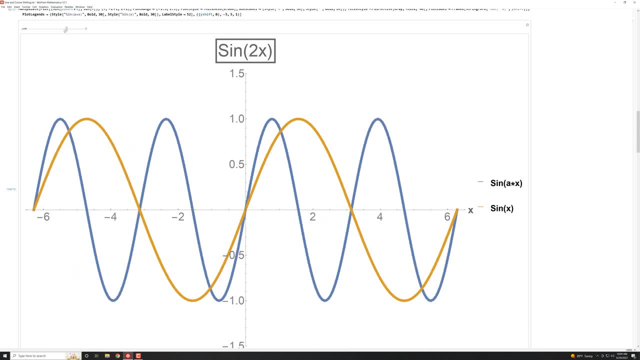 you're doing is changing the frequency, also doing the same thing as changing the period. When you have a higher number, that means there's that many is wiggling faster, which means there's that many complete periods inside of the baseline period of 2 pi. 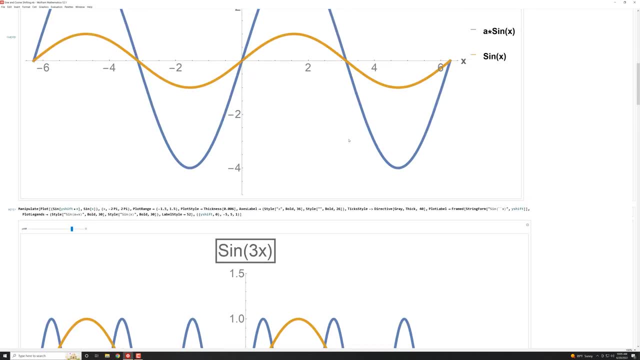 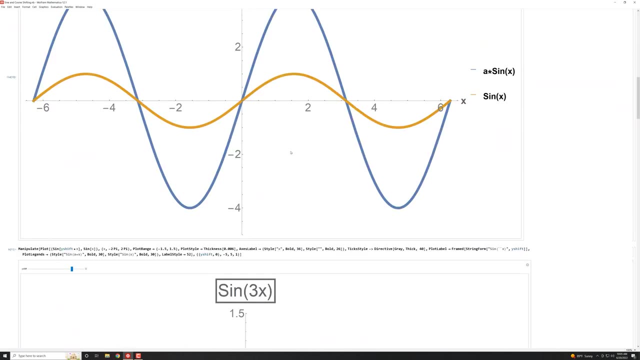 that we're familiar with Now. we're going to do this later- but you can combine all of these things together. You can add a number on the outside, you can at the same time change the number in front of the sine, and you can also change the number in front of the x and do all of these at the same. 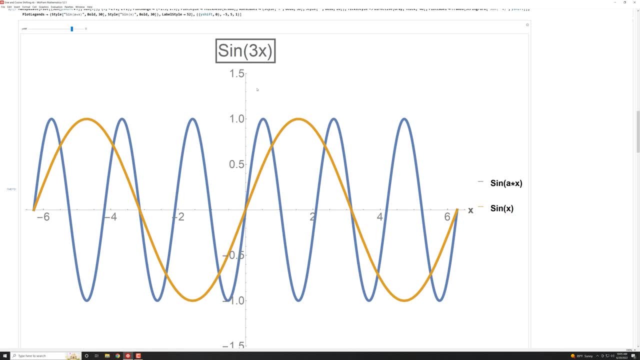 time. You can change the frequency, the period you know and the shifting all at once, and the thing will move accordingly to all three of those. Like they're separate knobs you can turn in order to change the way the thing looks. okay, Now everything applies to cosine, So this: 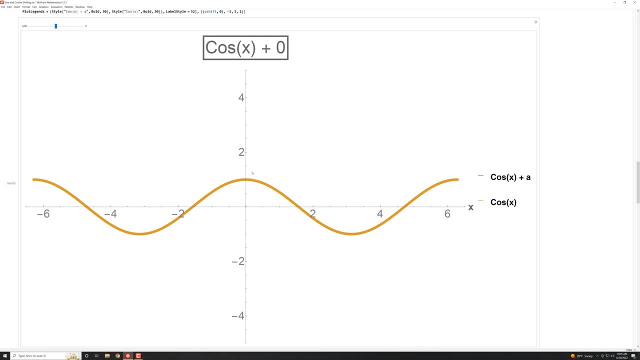 is going to be very simple, This is not going to take very long. Here we have the cosine function Differs, because it starts at a maximum, goes down and then back up to its starting point, And so it has one complete cycle again in 2 pi radians. So if I add a number on the outside of 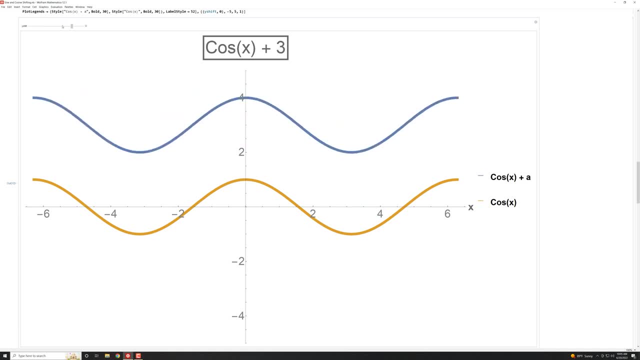 the cosine. then as I add positive numbers, the whole graph just shifts up, And if I make those numbers negative, which is like subtracting a constant, then I shift the thing down. That's very much the same thing as the sine function. If I put a number on the outside of 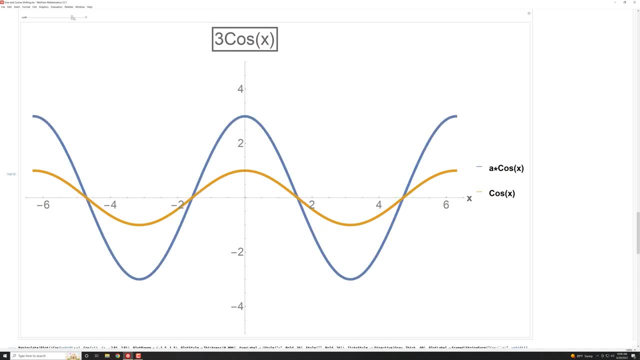 a cosine function like this, then all I'm going to do is I'm going to change the amplitude here. So notice: here the cosine goes up to three and then down the negative three and so on there. And of course, if I put a negative amplitude, the thing inverts. 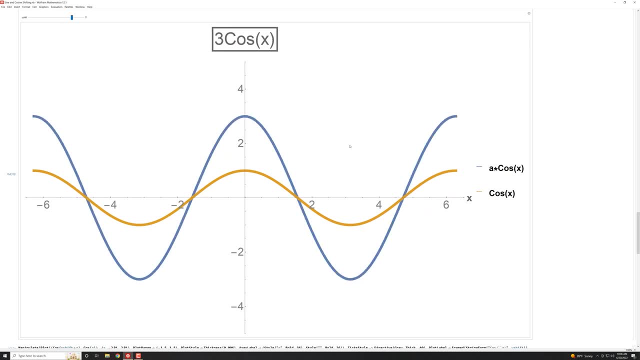 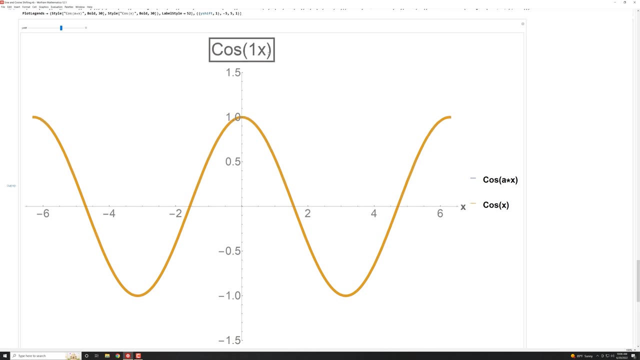 same as before. okay, So that's changing the amplitude of the cosine function. And then if I change the number that's on the inside of here, like this: right now it's cosine of 1x, which is cosine of x, which is the regular cosine function. 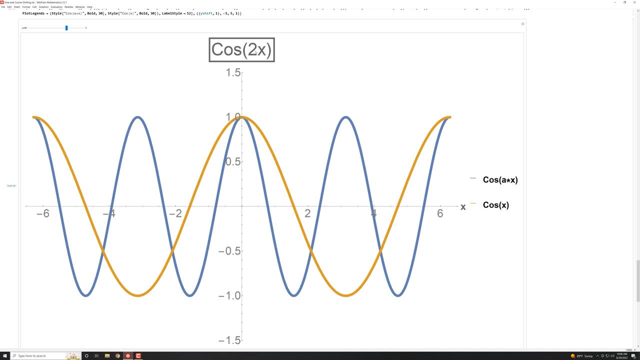 But if I make it 2x, notice what happens: The blue curve. I have now two complete cycles of the cosine And so if I put a 2x here, I have now two complete cycles of the cosine. So this gives me. 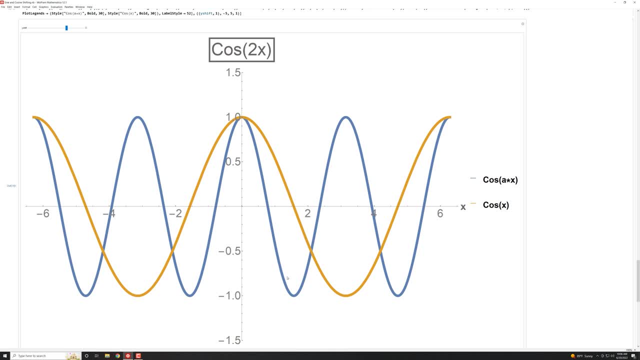 a cosine function in a normal 2pi baseline. The baseline function, the goal function, the period is 2pi. But when I put a 2 here, I have to have two complete cycles. There's 1, and then here is the second complete cycle in the same region. All right, if I make it a 3,. 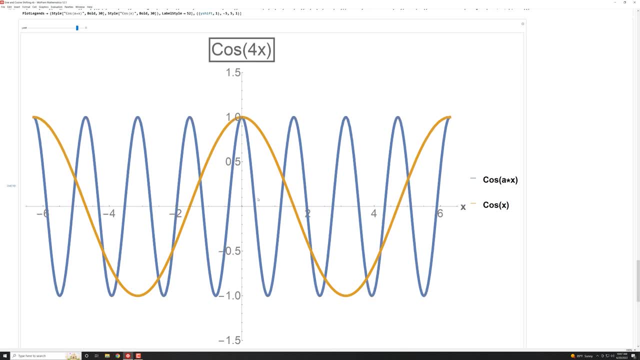 then now I have three complete cycles of the cosine: There's 1,, there's 2, and there's 3 in the same region. If I make it 4, I have now four complete cycles of the cosine. There's 1,. 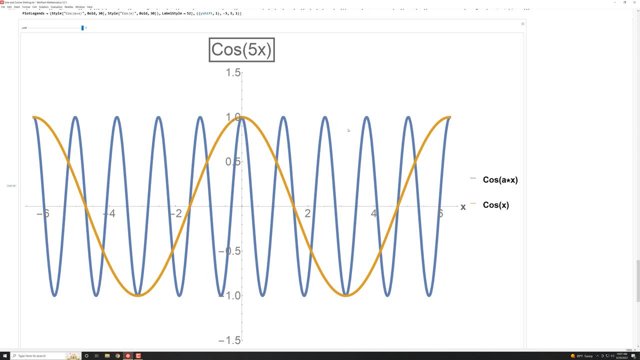 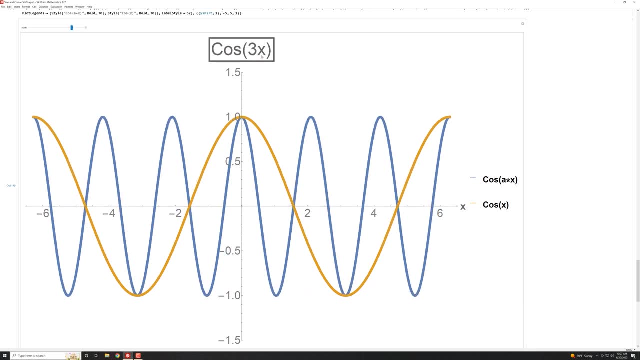 to five or six or whatever. this number increases the frequency. This blue curve is a higher frequency than the gold curve. All right, And again, why does this work? Because if I make it cosine of three times X, then I don't have to increase X very much in order to go all the way. 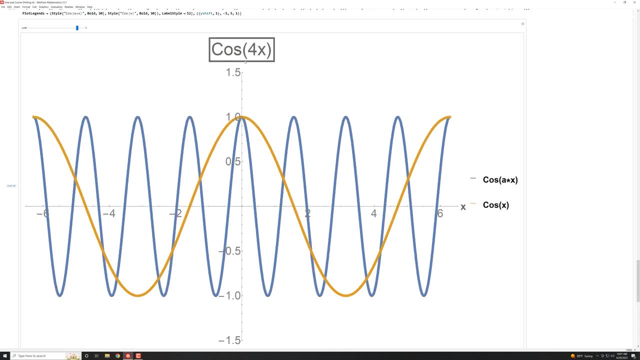 around the unit circle. Because, for instance, if I change it to cosine of four times X, if I go to, let's just say I put two pi radians in here, Well the gold curve, the regular cosine, is going to only have one cycle when I do two pi radians. But if I put two pi radians here, that's going to. 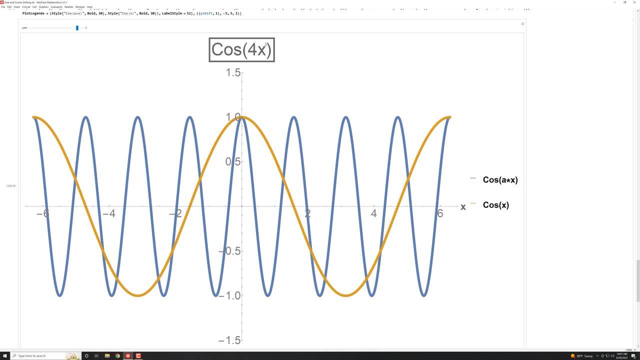 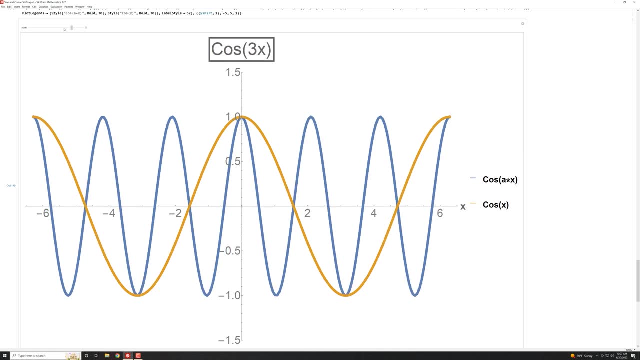 be cosine of eight, pi. So eight pi is already four times around the unit circle. So that's why it's like one, then two, then three, then four, like this. And if I change it back down to cosine of two, X, for instance, if I only go pi radians, which is only halfway around the unit circle, 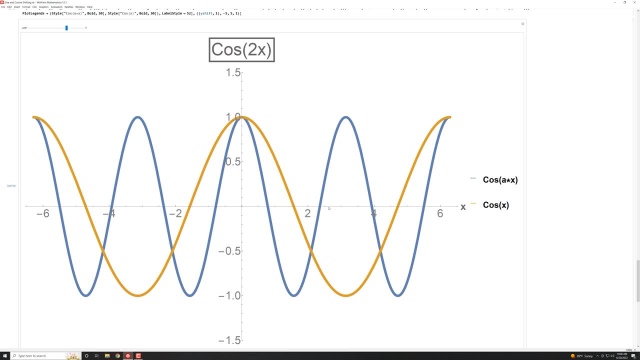 then I've completed this cosine of two pi, which means I've completed one cycle of this thing. So the number that's in front of the variable basically makes you go around the unit circle twice as fast. And then here I'm going around the unit circle three times as fast. And here I'm going around the unit circle. 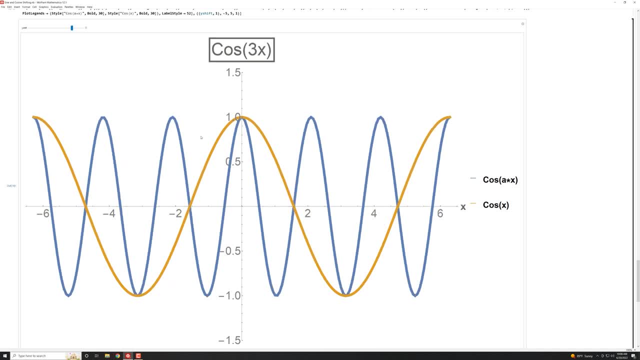 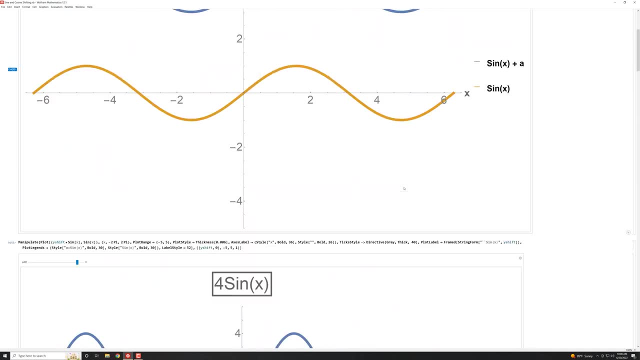 four times as fast and five times as fast, And that is why you're seeing the thing repeat so many times in a two pi region. So that is something I want you to try to remember. That's why I kind of went over it a few times. We do have some more drawing to do on the board and do some problems. 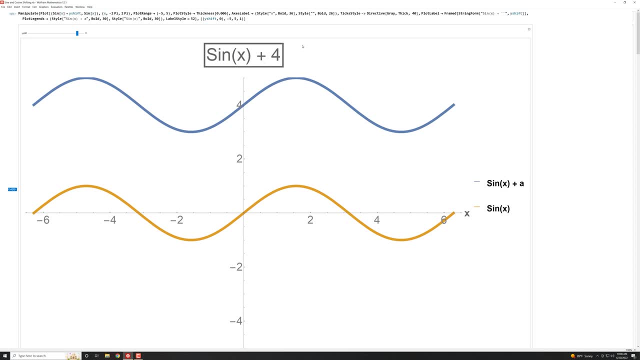 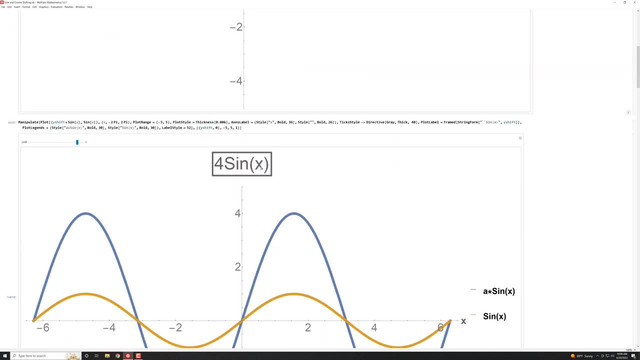 to show you how to work with it. But basically this is the way it works for all trig functions. If you add a number on the side, then it just shifts the thing up and down, But it's the exact same shape If you put a number. 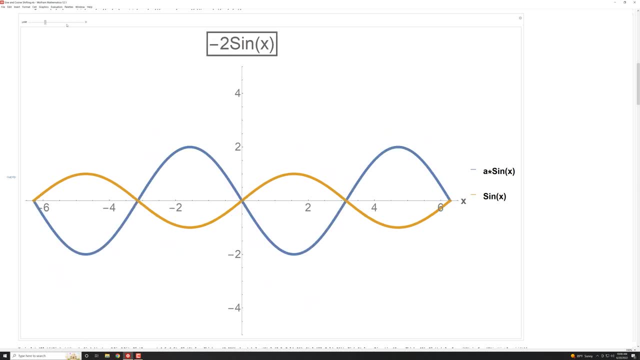 in front it just. everything else stays the same, the crossing points and all that stuff. The only thing is the amplitude goes up, which means the maximum and minimum go up to hot. positive four and negative four. In this case, if you put a number on the inside, you're forcing the thing. 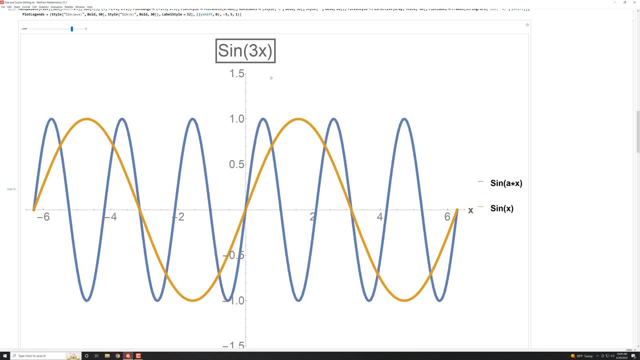 to go the angle, to change around the unit circle faster. So you have more cycles. how many more cycles? whatever the number is, that's how many complete cycles You must have in a two pi region, because the baseline sine function has a, has a period of two. 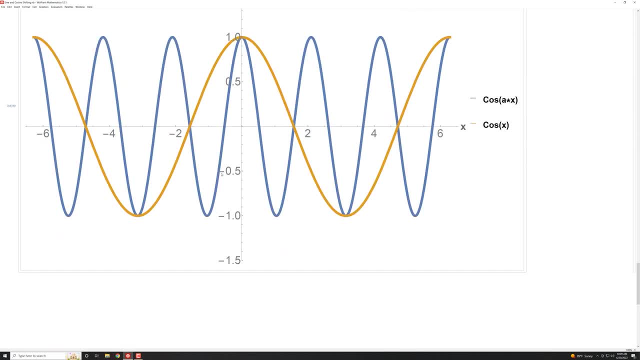 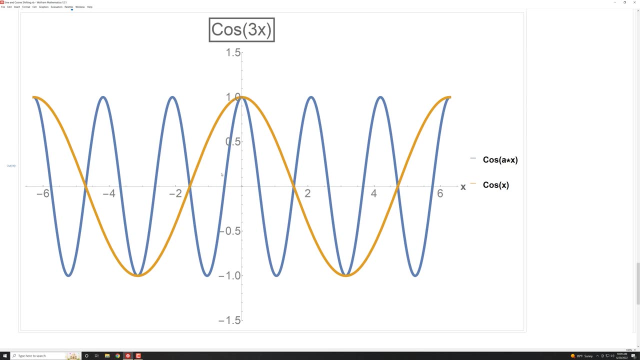 pi. Same exact story for the cosine function. So now what I'd like to do is: let's step away from the computer, go back to the board. we'll draw more pictures and cut into our example so that we can get a hang of how to use this. All right, welcome back to the real world where we jump in. 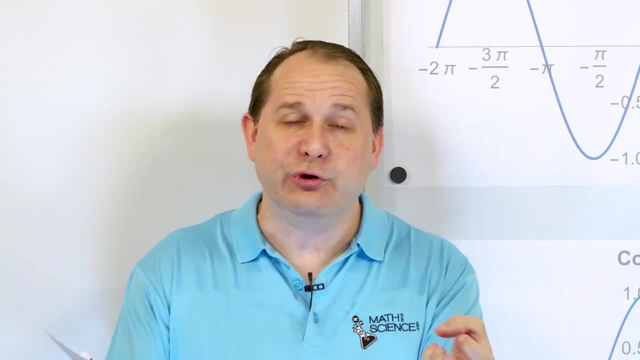 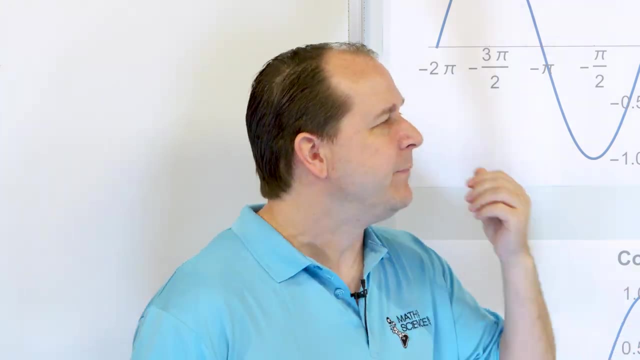 and draw things, and write things and and so on. So here we have to use what we learned in the computer to apply it to real problems. Hopefully, seeing it graphic, you can burn in your head what these different numbers do. right, So we have our basic functions. 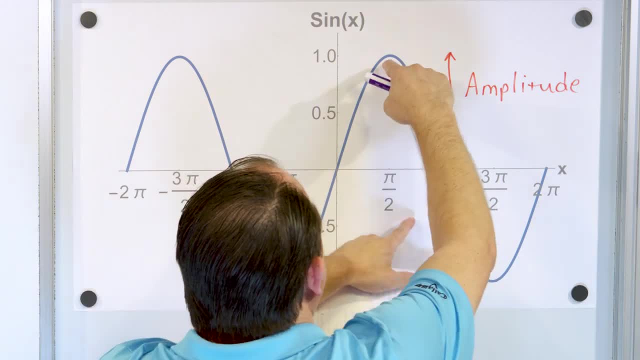 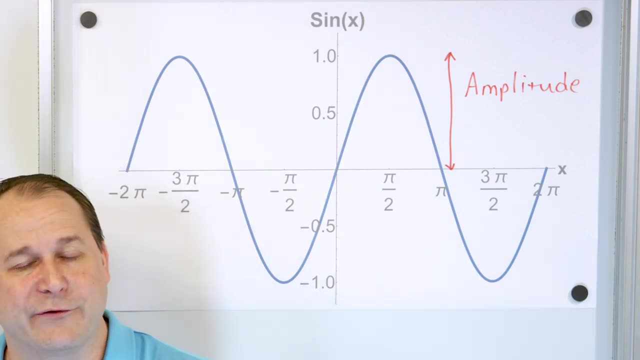 right, We can shift it up and down. right, We can increase the amplitude higher or lower, and we can also make it wiggle faster, which means we change the period of the function, Also change the frequency, because the frequency and the period are related to each other. We say: 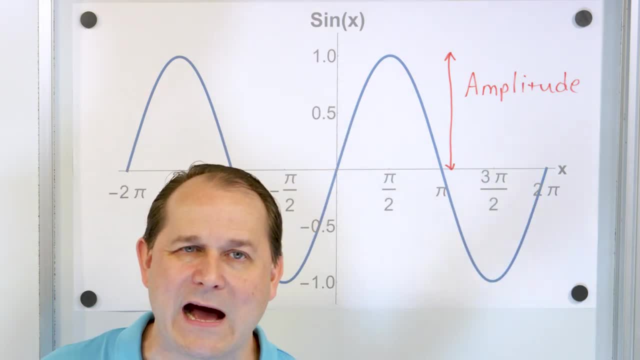 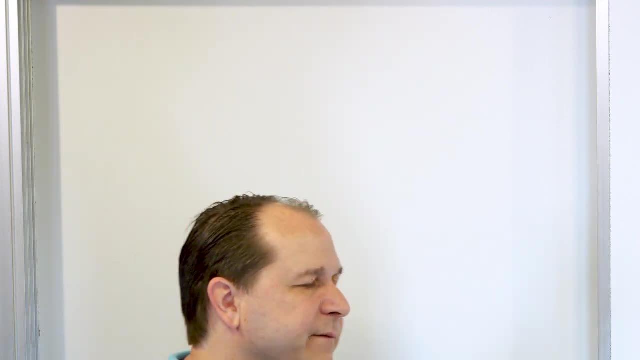 we have a higher frequency, the more wiggles that we have are, the higher the wiggling that's going on here. Same thing true of sine and cosine. So what I want to do first, it's kind of like I want to. 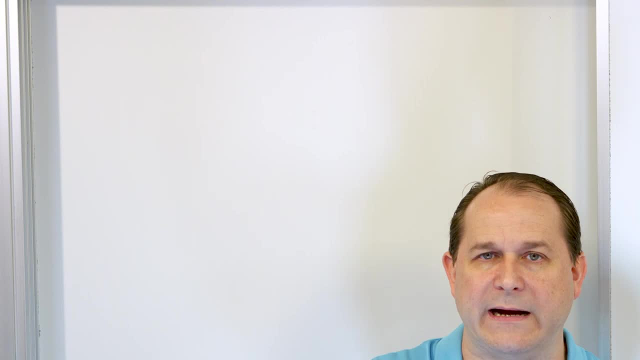 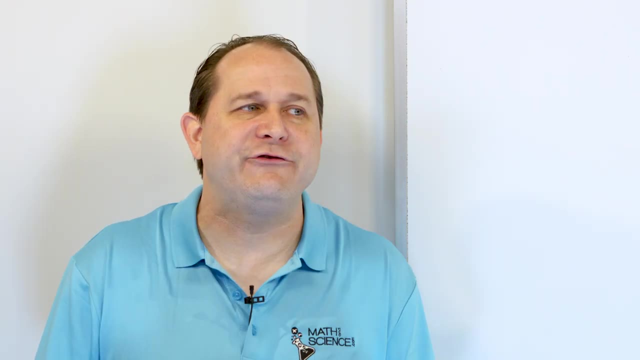 summarize what we did on the computer, because you can watch somebody play with a slider on a computer and it might help, and it does help. but we have to also get good at drawing things. I can't just tell you: here's some beautiful graphs, Good luck, Go ahead and draw them. I can't do that. I. 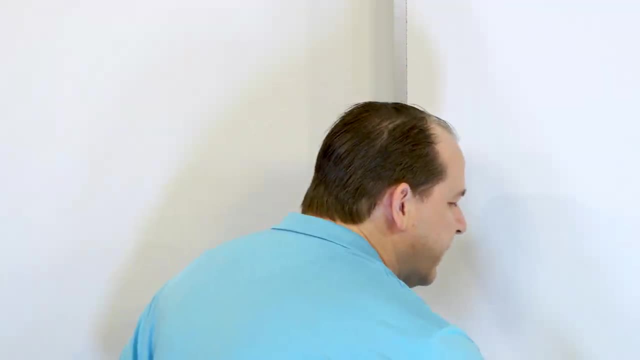 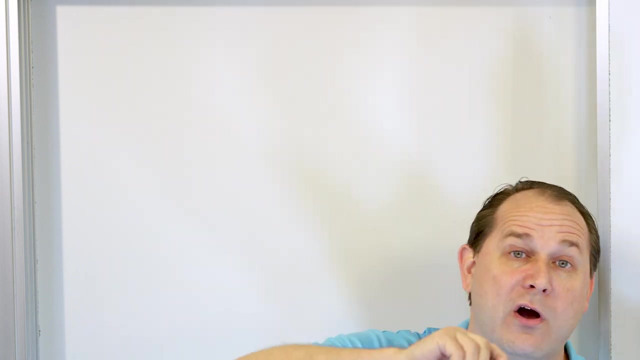 wouldn't feel good about myself. We have to learn how to do these, So I want you to get good at drawing these, and you just kind of have to to to do that. When you take chemistry and organic chemistry, you have to learn how to draw molecules. If you take art class, you have to learn how to. 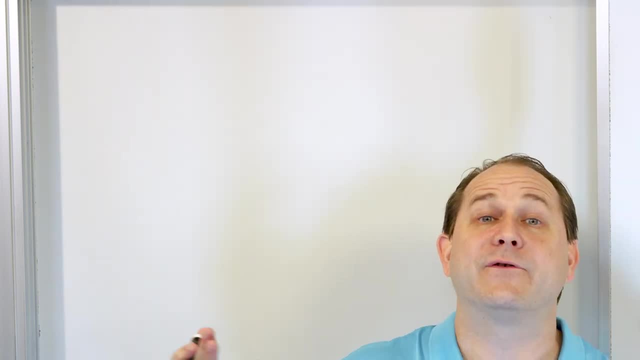 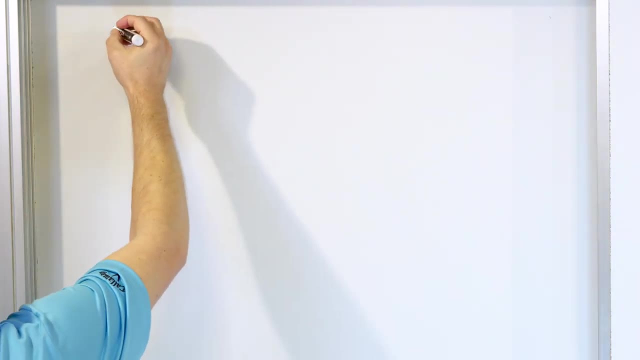 draw whatever they learned how to draw. If you take art class in math, you have to learn how to draw your trig functions. You just have to. but the good news is is very easy the way I'm going to show you. So, first of all, we have to. 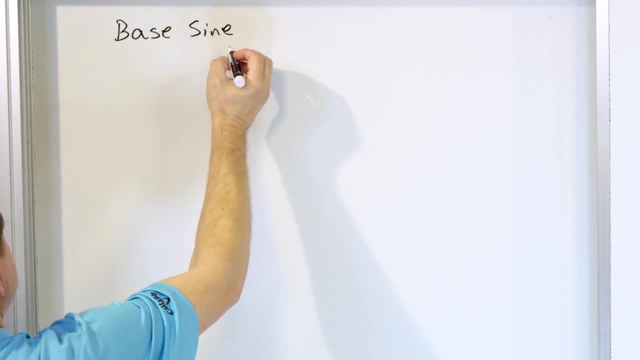 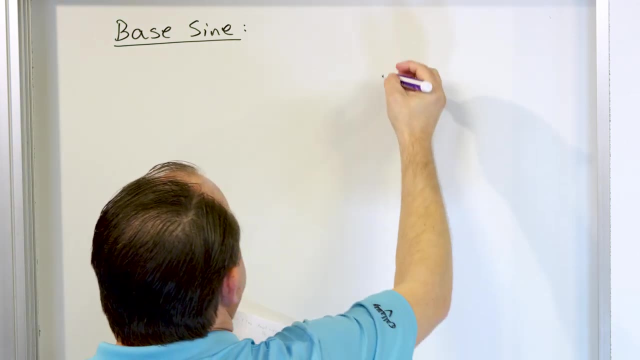 take a look at what I call the base sign. the base sign because we have to have the baseline function in our brain. I know that you know what this is, but we also have to get good at drawing it. So how do we draw it? We just make a little quick X- Y axis. It doesn't have to be pretty. 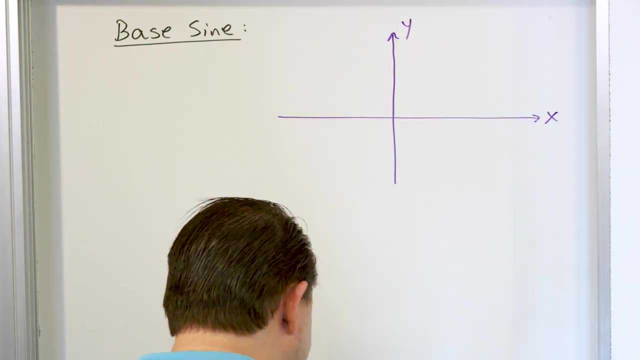 So we have X, we have Y. I know we have those beautiful graphs over there, but that's not the point. Now, where does that come from? It comes from the base line. It comes from the base line. So we have X, we have Y. I know we have those beautiful graphs over there, but that's not the point. 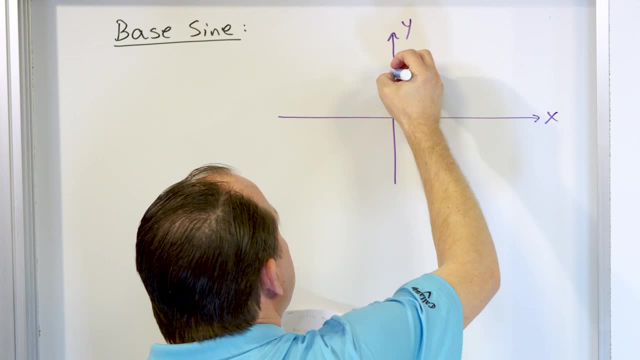 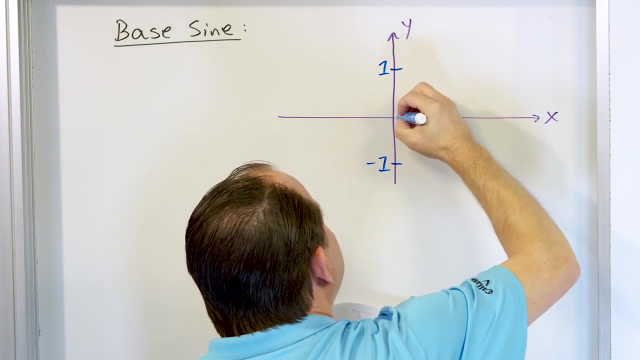 Now, where does the sign start right? Well, we know that it goes up only to a maximum of one and it goes down to a maximum of negative one. We know that it starts at the origin Sign, starts at the origin Cosine, starts up here. So we know it goes up and it reaches a maximum. 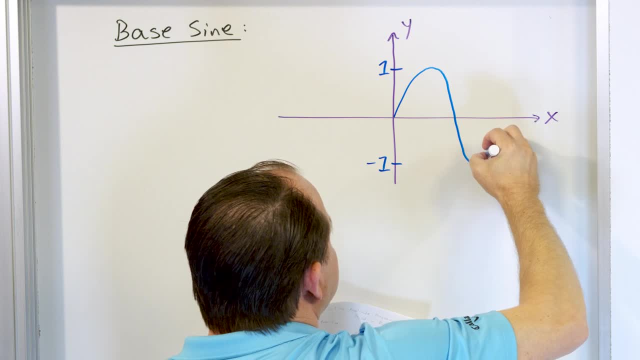 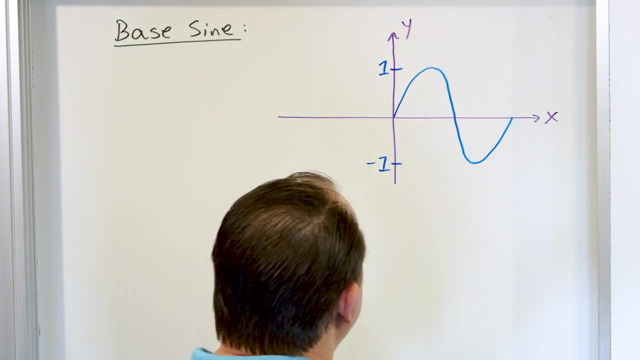 and then it goes down here and it reaches a minimum and then it has to go and start over again. So that's a basic sign. Now you don't have to label all of these every time, but we're going to label them here in the beginning. When does the thing begin to? 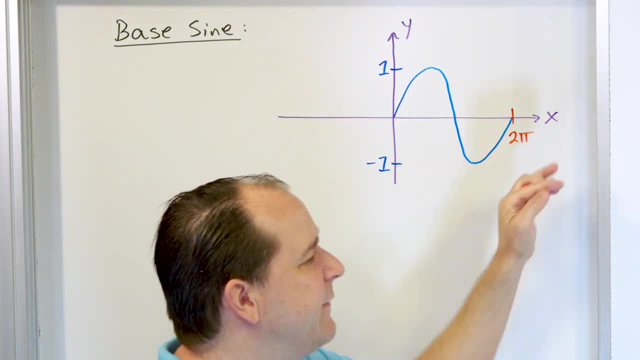 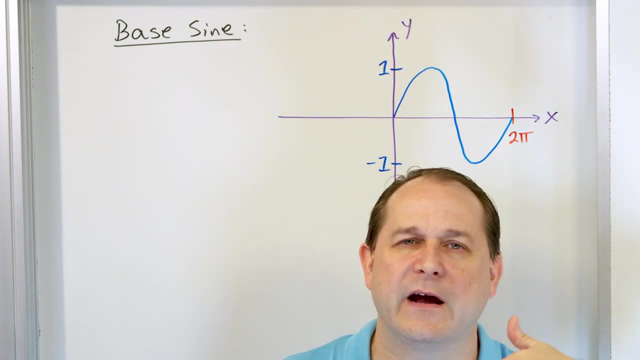 repeat Two pi radians, So X is two pi radians. or you can think of X being an angle theta, which is what it really is. So when you get more into engineering we refer to the input to the sine function as being an angle theta. But in math classes usually we say the variable is X. So 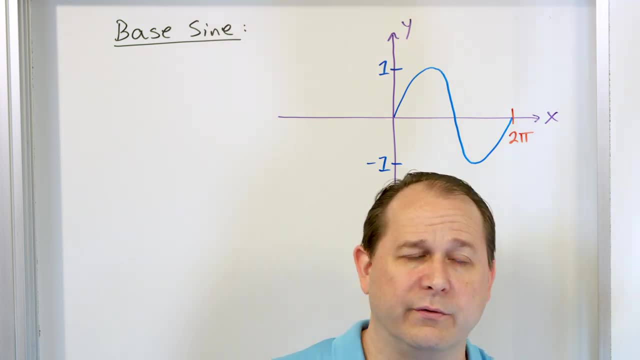 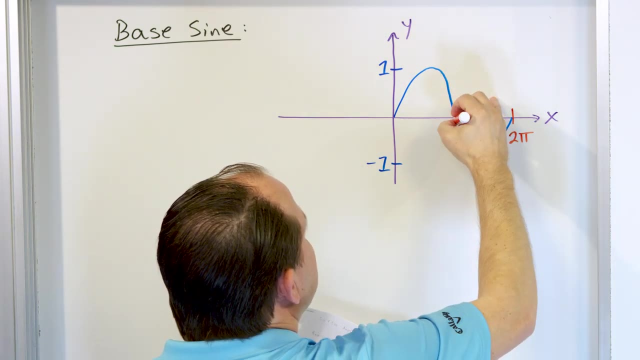 don't get too wrapped up in X. X is an angle on the unit circle. That's what it is. We begin to repeat ourselves at two pi radians. So if this is two pi radians, then what must be in the middle, here at the crossing point, must be pi radians. right, Because 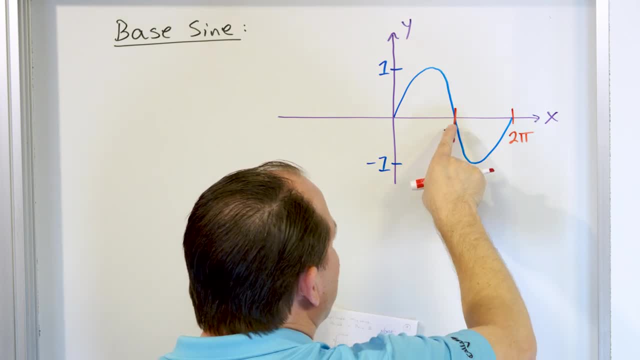 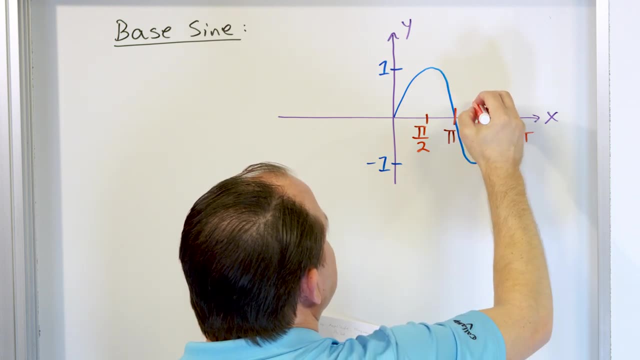 half of two pi is pi, And then if it crosses here at pi, then the maximum must be here at pi over two, And the minimum must be here at, so that's pi over two, then two pi over two, then three pi over two. 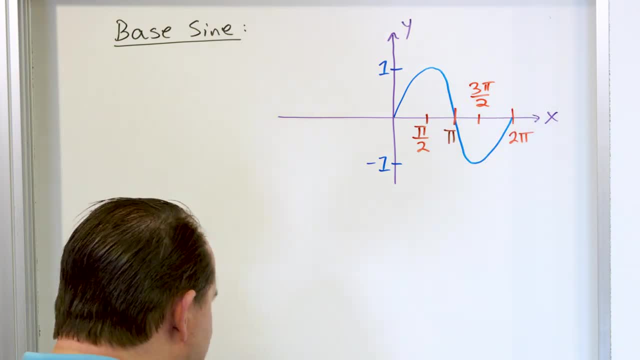 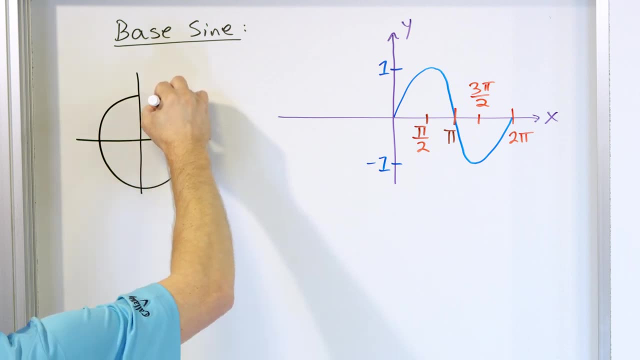 This is going to be three pi over two, So these are the quadrants of the unit circle. When you think about what's really going on here, if I draw the corresponding unit circle, just remind you that the unit circle is a radius one, so negative one, negative one and one like this, then you can 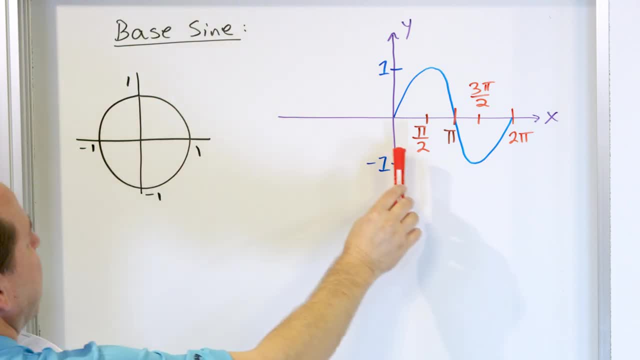 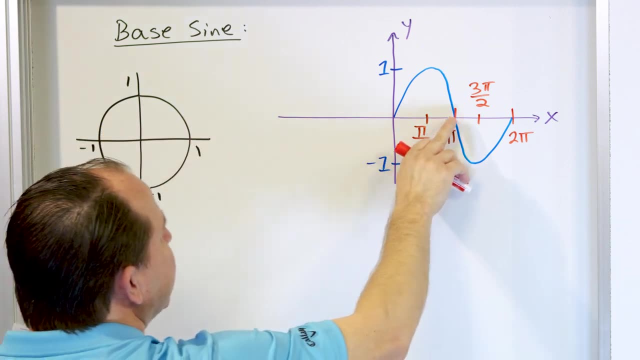 make the位 and distributed right here. Actually, you can make the ward right there in the case where the Monsters can't pick up what you're here And the Redo set, as I mentioned, features there. but what I highly 궂 Taxist. 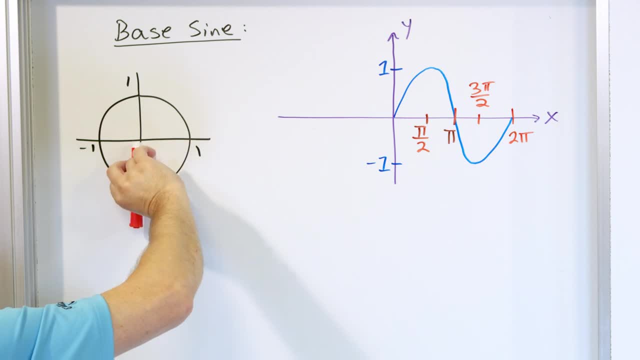 000.. 29, 0 radian 1 sin pie прав over 2 display directly Here. that's right here. That's why the sine is a maximum. This is Pi. That's why that, because it's a projection on the Y axis. That's why the sine goes to zero here. 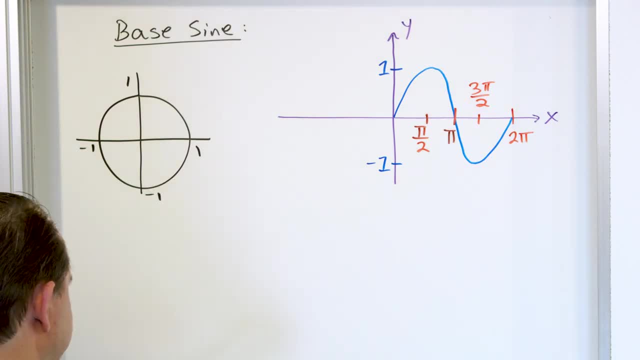 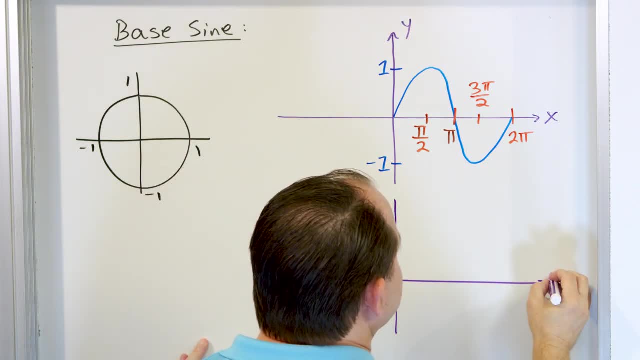 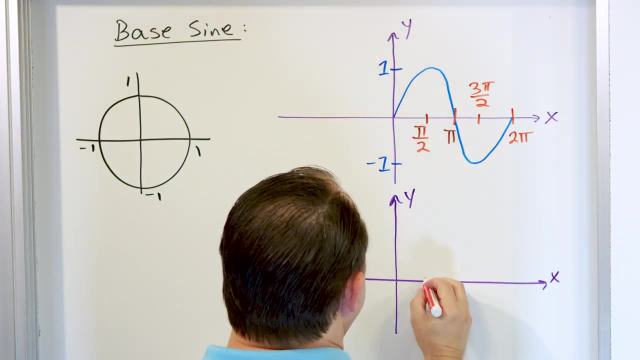 I am trying to get you used to drawing these things, but we're not gonna use those. I'm gonna use mostly the sine function to prototype these things. So we have basically the same little figures here. We have pi over two. that's an important number. 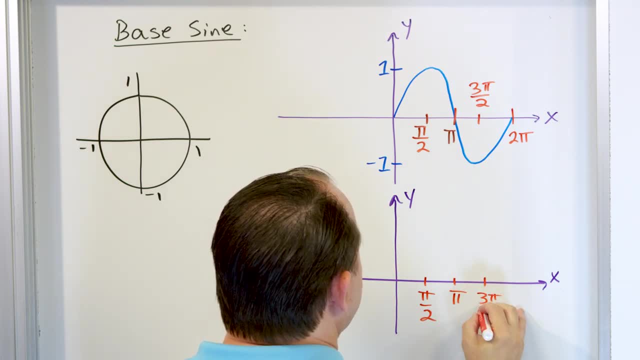 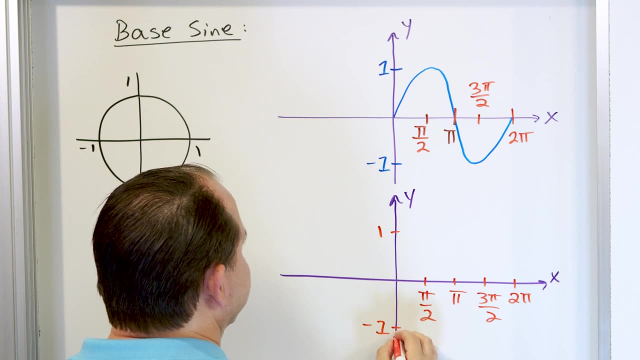 We have pi- that's an important number. We have three pi over two- that's an important number. And we have two pi, which is an important number, And then we have positive one and negative one, like this. So you have to get just good at drawing these things. 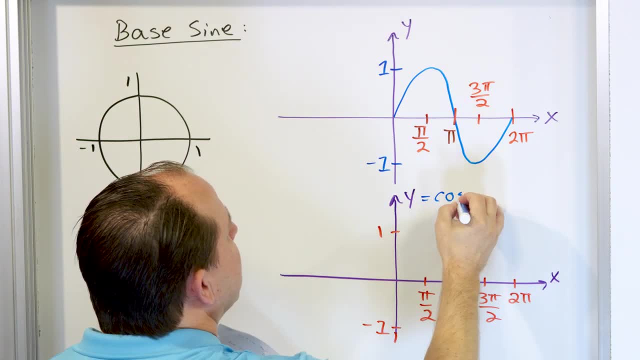 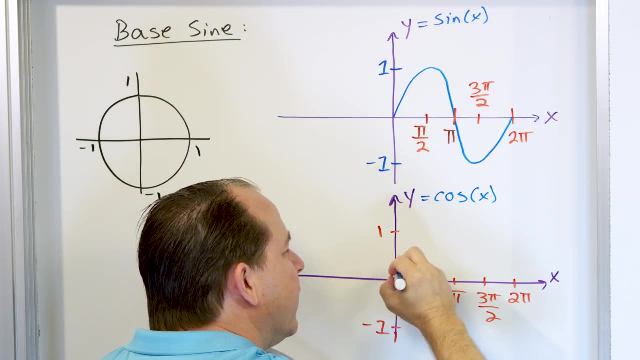 All right. so if it's a cosine function, this is cosine of x and we'll say this is sine of x. All right, so how do we draw the cosine function? It doesn't start here. the sine function starts here. 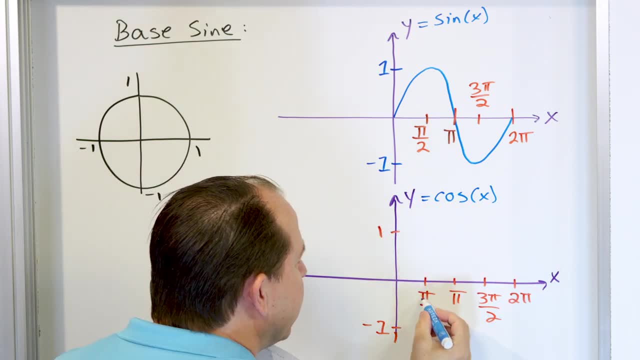 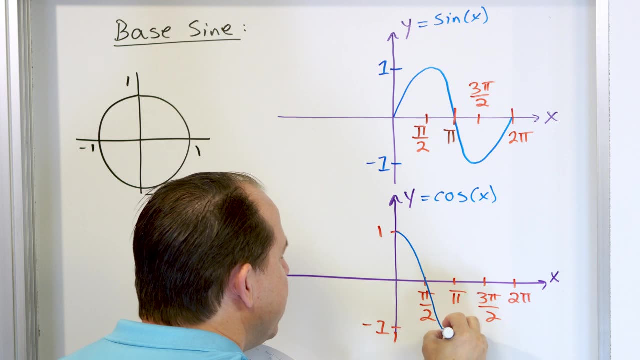 The cosine function starts at the top and that means it goes through zero here and reaches a minimum here and then goes through here and then goes back and traces like this. So it goes down through here, then down through here, up through here and then back, like this: 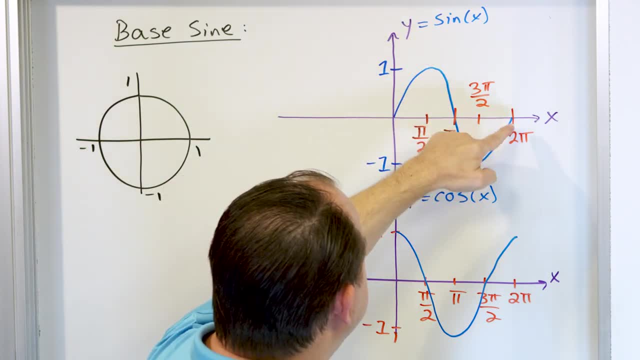 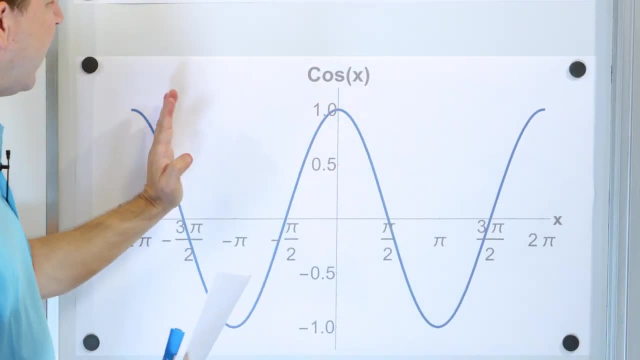 Is that perfect? No, but it's pretty close. So the sine function up down up, the cosine function down up here and then back up again. Let's check ourselves, because we didn't draw the negative side of it. 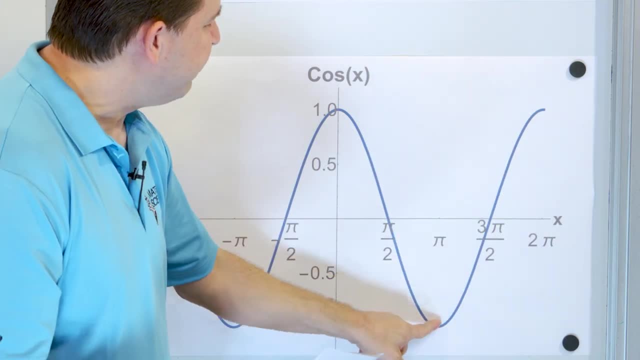 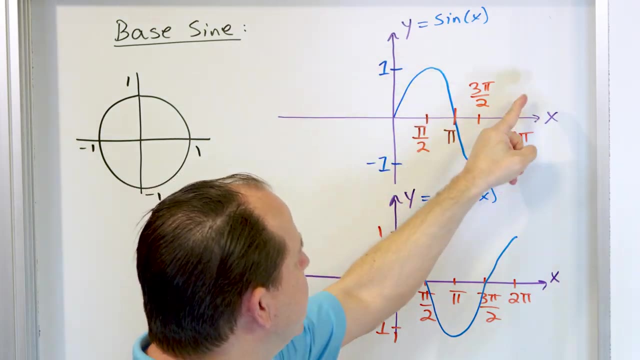 Over here, down and back up again at two pi. it reaches a minimum point at pi right here, which is exactly what we have shown here, And the sine goes up down, up like this, up down, up like this. 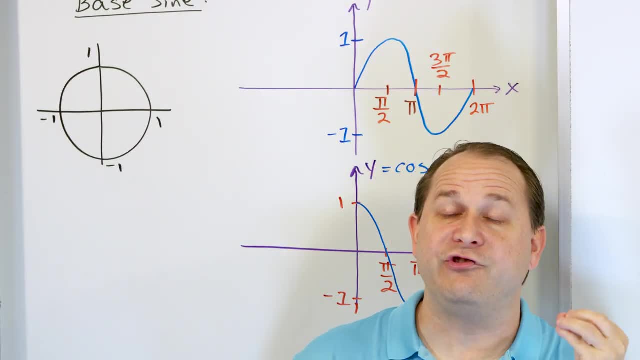 All right. so why am I drawing this? Because I'm trying to burn it in your head. the baseline functions. you have to have them in your head, Okay, So I'm trying to help you with that. Now, if I want to shift, 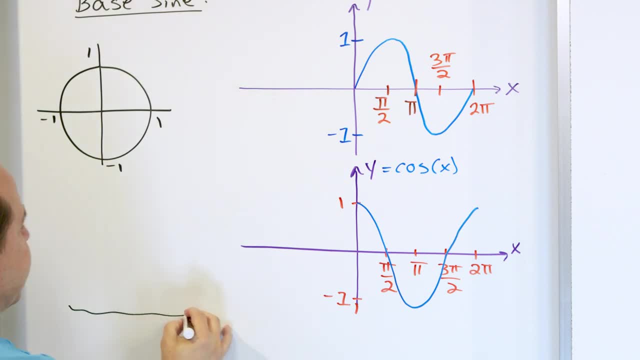 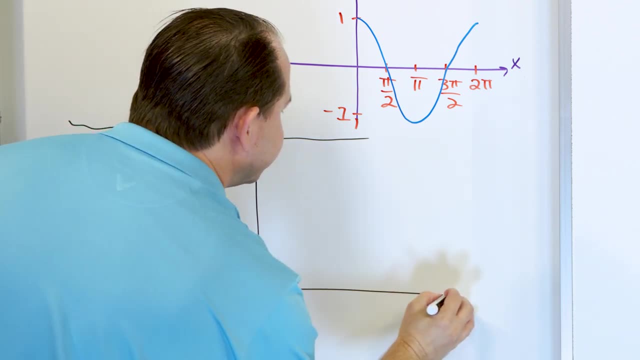 we're going to focus our attention on the sine function here. If I want to shift the sine up or down, how would I do that? Well, let's draw a graph like this: We'll say this is x and we'll say this is y. right, 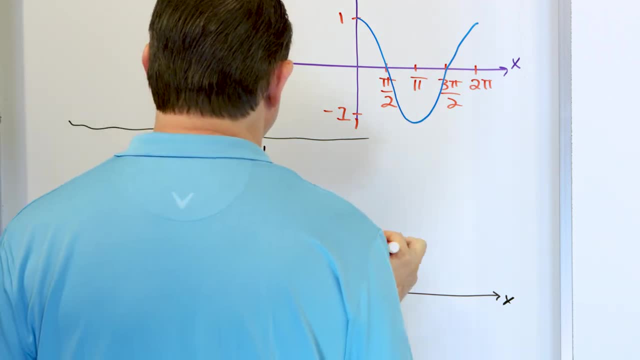 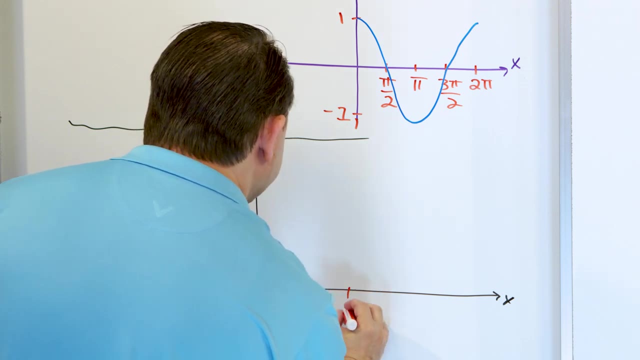 Now let's go ahead and put the same kind of thing in place here. If I want to say that this is pi over two, and then right here, this is pi over two. right, And right here is pi. we're just going around the unit circle. 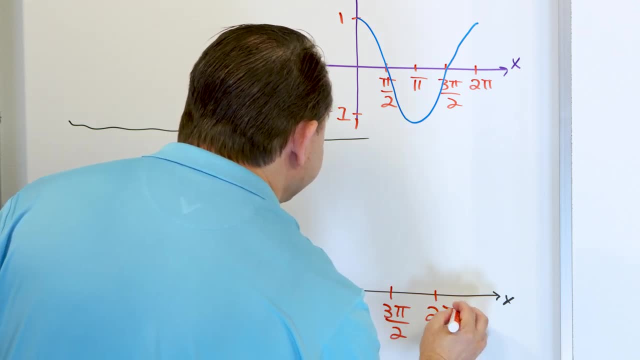 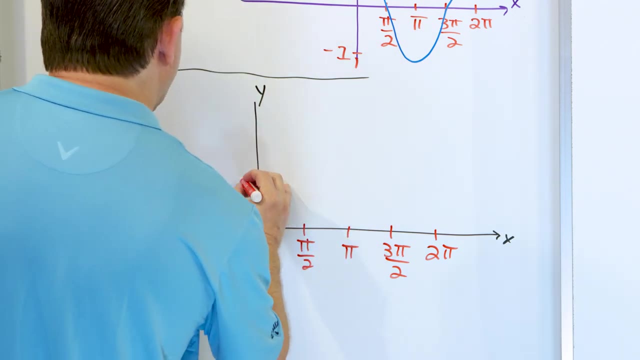 three pi over two. these are important numbers. and then two pi, These are the quadrants, the y-axis markings of the angles on the unit circle right. And then here we have one here, and then here we have two, and then here we have negative one. 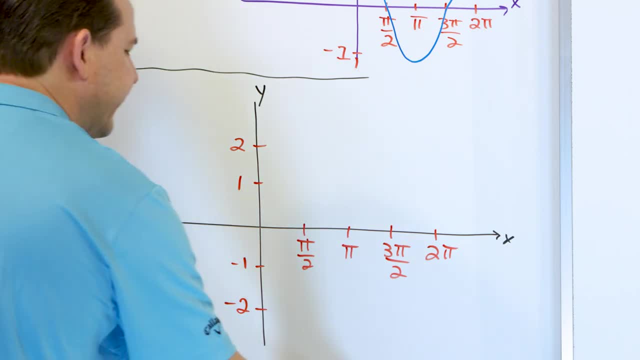 and then here we have negative two. All right, What does the baseline function look like? I'm not going to draw, but we know it starts here and then it goes up here and it goes to negative one and it goes here. 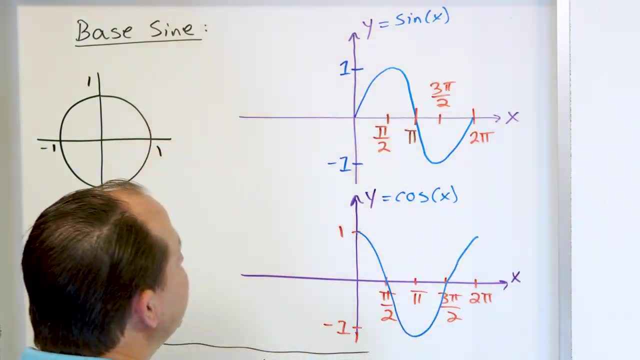 Now what if I want to take the sine function and then it goes to negative one and it goes here. I'm going to take the sine function and shift it up one unit. If you take a function, any function, and shift the entire function up one unit. 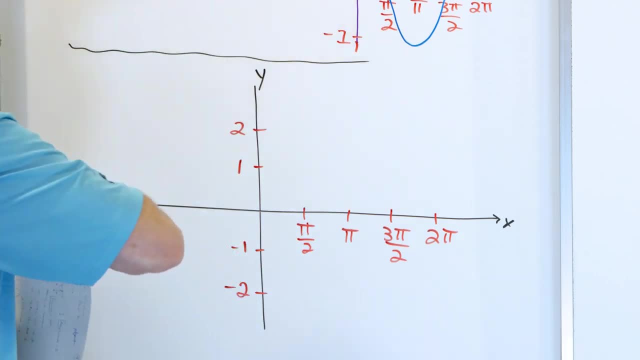 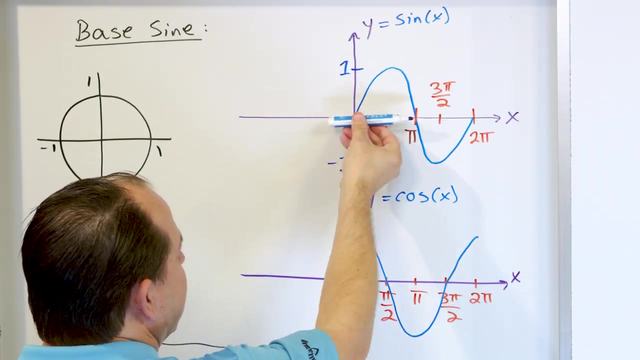 all you're doing is you're adding one to the whole thing, And what would that thing look like? Well, what you can do sometimes to help yourself is you can. you can say: well, the normal sine has a kind of like an average value right here. 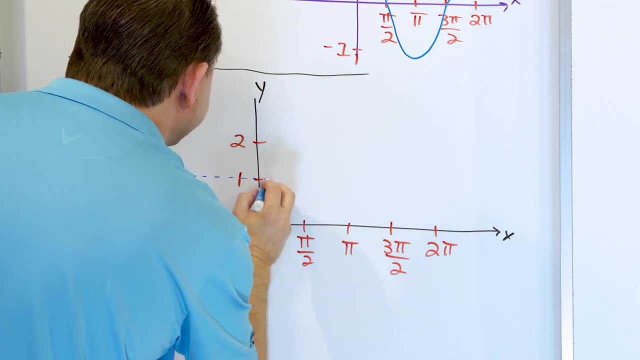 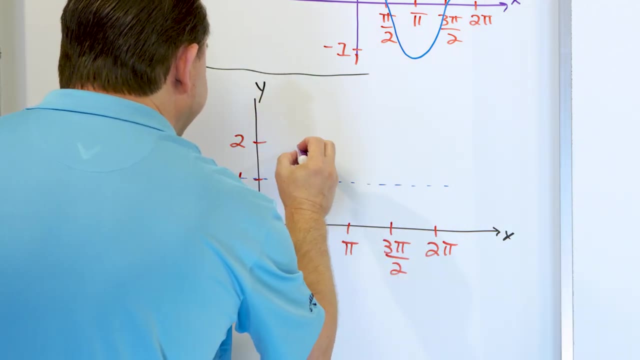 So what I can do, if I want to, to help me visualize it is I can draw this as a little dotted line to help me guide myself, And then I can say: all right, then I'm going to start it, this is going to be a maximum. 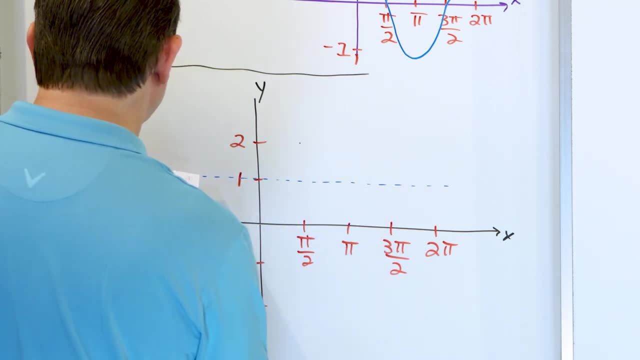 And then this right here is going to be a minimum, And then it's going to go back up to being a maximum right here, like this. So I could go down and then up, like this. So if you're going to shift this thing up, 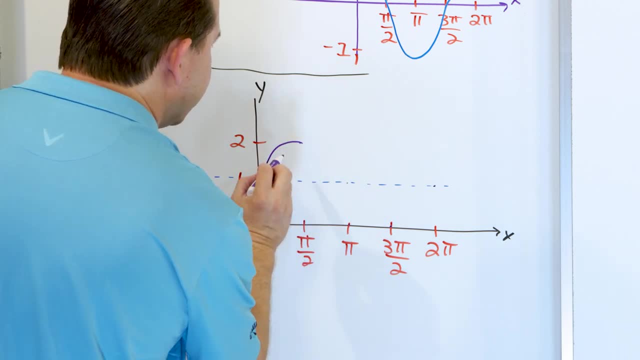 it's going to be something like this: It's going to be going up to a maximum right there and then it's going to go through zero right there. Then it's going to hit some minimum right there, Then it's going to go up there. 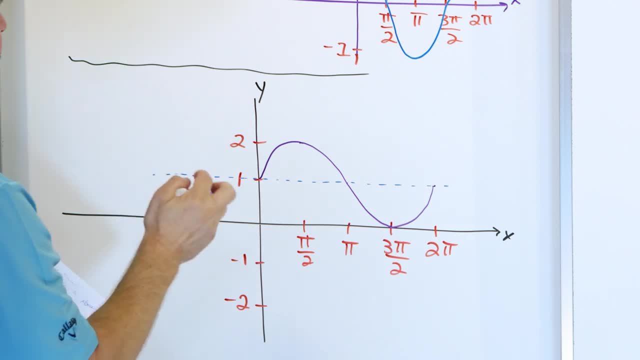 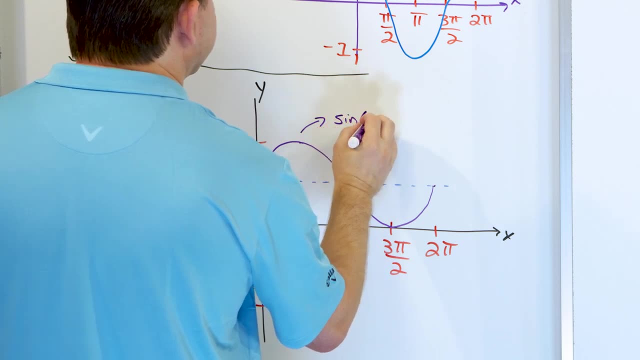 and you can see this is lopsided. This is not like a great graph. you get the idea. the entire thing is shifted up. So this graph right here is a sine of X And then, on the outside of the sine, function. 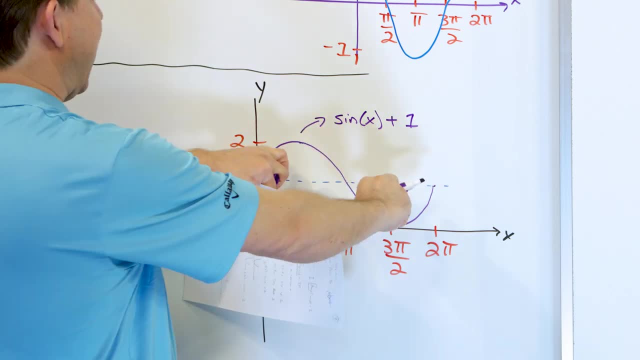 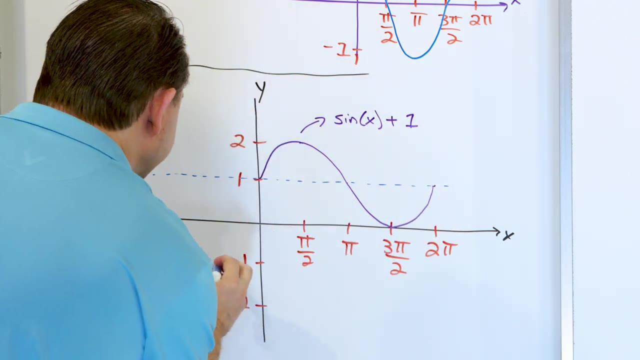 we add the number one. Now, what would happen if we wanted to take this graph and shift it? the baseline, remember, is here to shift it down. Well, you can do the same kind of thing here If you want. you don't have to. 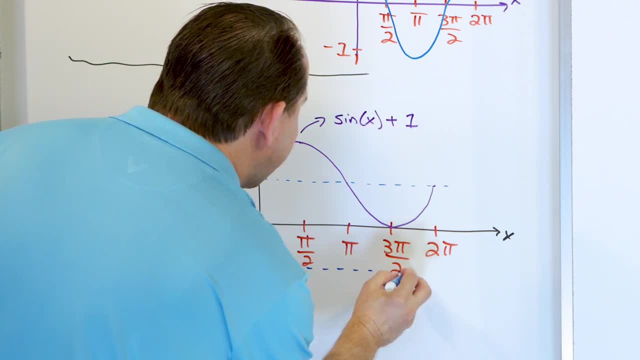 You could say, well, I'm gonna kind of give myself a little help and say this is kind of like the average value of that sine function there. And what am I gonna do? I would say, well, it's gonna start here. 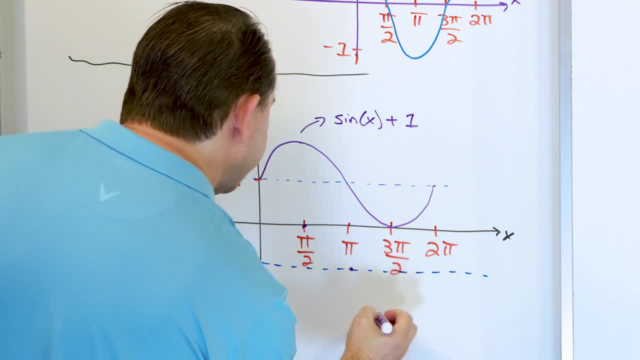 and you can put little dots to help you. It's gonna go there and then it's gonna come down there and then over here it's gonna come down here and then it's gonna go back to right there and then just draw the thing again the best you can. 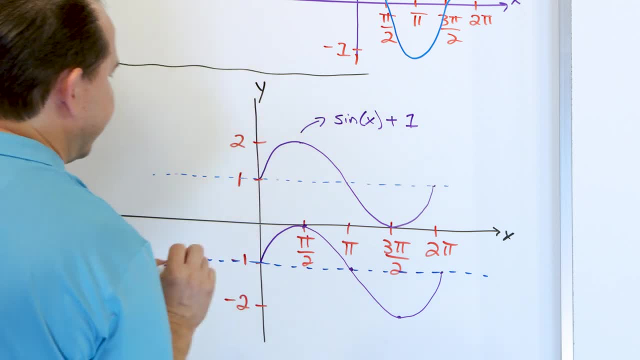 like this down here and then like this: And what is this function? This one is sine of X, and then we're gonna subtract one. So this is a kind of a regurgitation or just a repeating of what we did on the computer there. 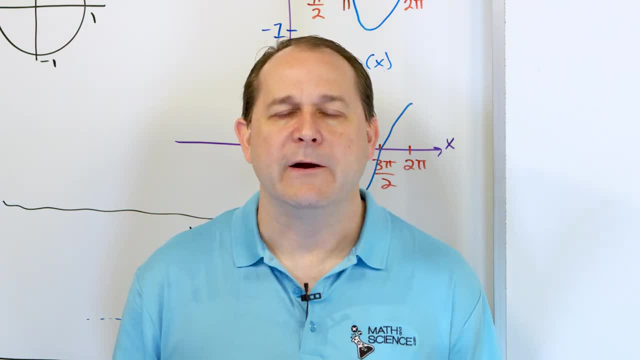 The reason I'm drawing it again is because in your homework you're not gonna be doing it on a computer. They'll say something like: here's a graph, sketch it. and you'll have to sketch it. So how do you do it? 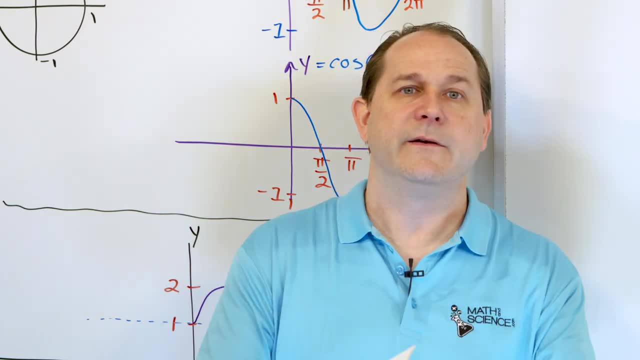 Well, you have to watch me do it. You can't just do it yourself. I can't just say here good luck. I mean that would be lame. So what I need to do is show you how to do it right. 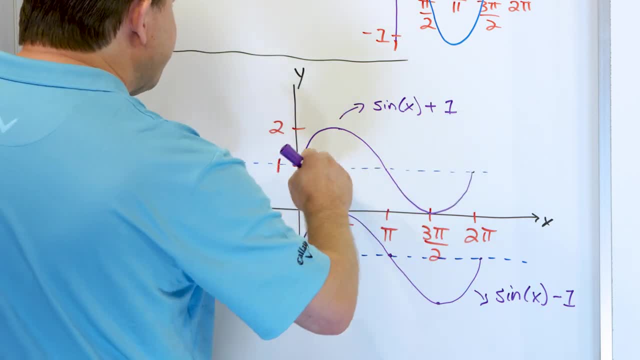 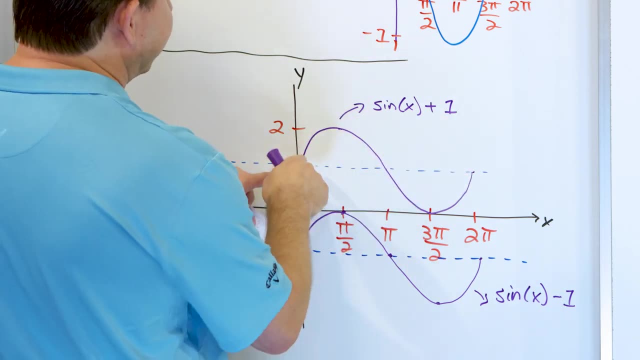 And this is how you do it. If you're trying to shift it up, draw yourself a new baseline, pretend that here is a new X and Y axis and put your dots somewhere. And I get confused with it. I got confused with it just a minute ago. 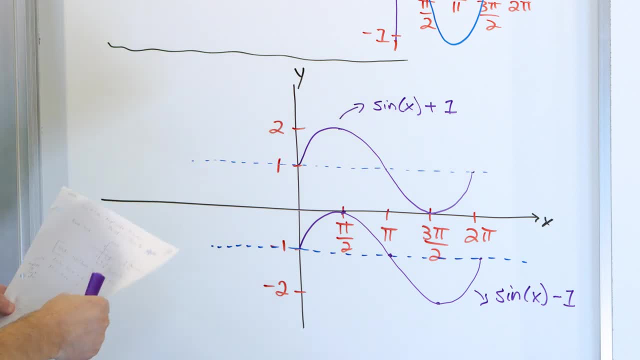 That's okay, Put your dots and then try your best to sketch it out, All right. so that's what we call changing the kind of the Y intercept of the function, or just shifting it up and down, basically by adding a constant or subtracting a constant here. 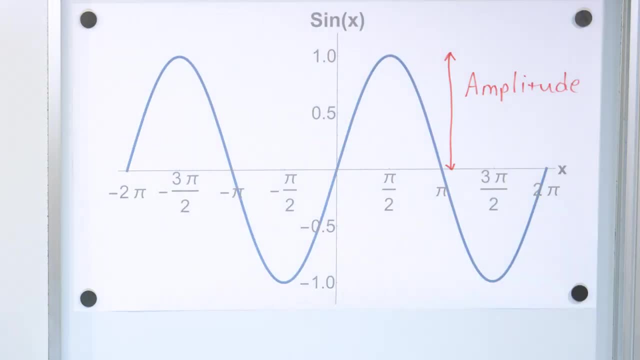 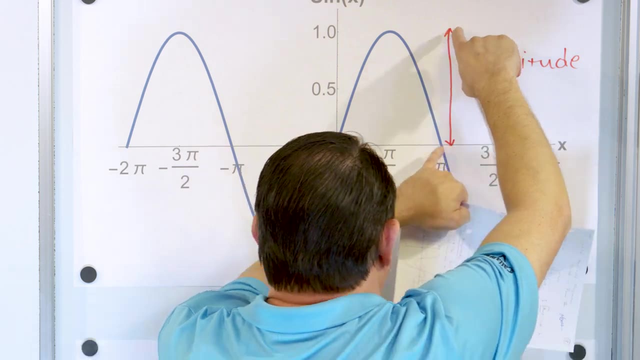 Now, how do we change the amplitude? Remember what is the amplitude. The amplitude of either of these waves is the distance from the X axis up to the maximum of the function. Same thing here. The amplitude here is one because it's a distance from the X axis. 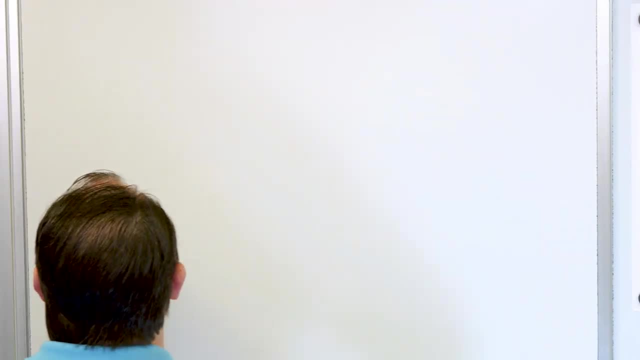 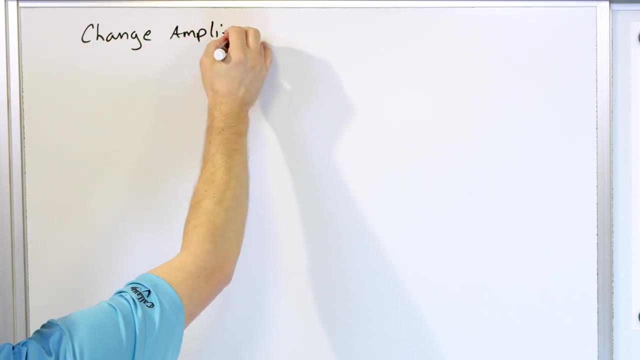 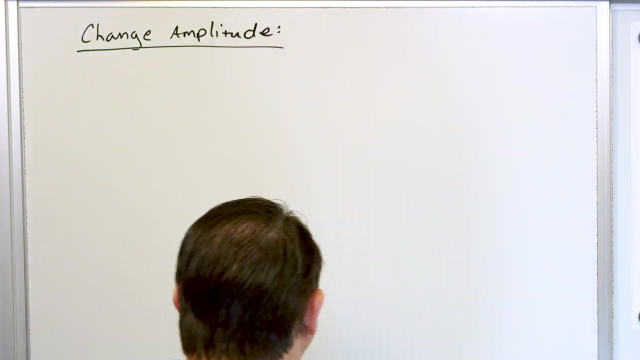 up to the amplitude of the function. So what we're gonna do next is we're gonna change that amplitude, and we've already seen how to do it because we've done the computer demo. but that's okay, We're learning and we're trying to figure this out. 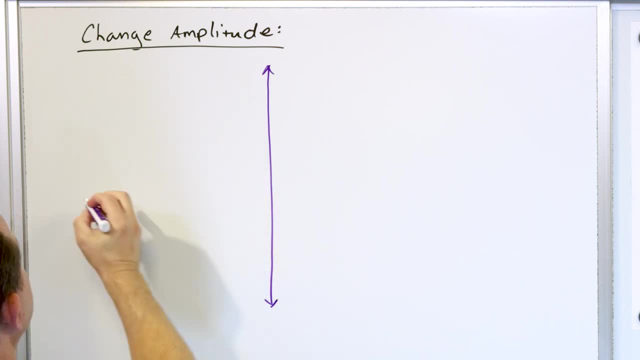 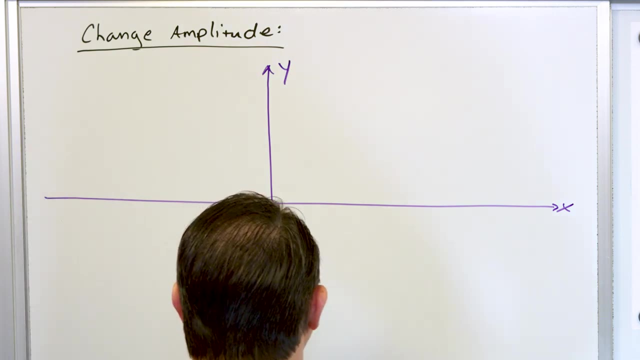 All right. so to illustrate this best, what I'm gonna do is draw a larger X- Y axis here. Here's X, here's Y, and we're going to draw the important points here. We're gonna mark there, mark there, mark there. 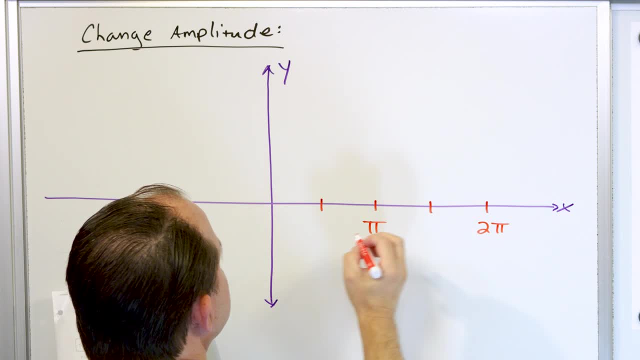 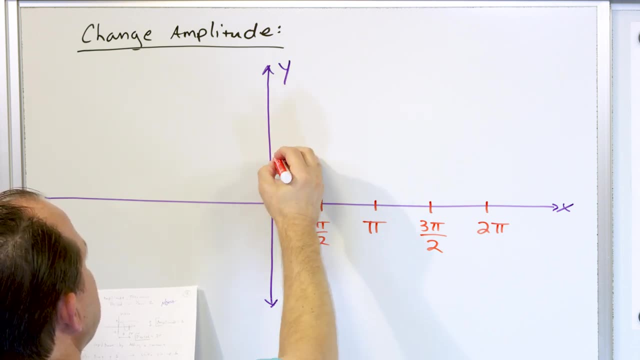 and mark there: This is pi, this is two pi. So this has to be pi over two, and this has to be three, pi over two, And this can go. let's do one, two, three. So that's one, two, three. 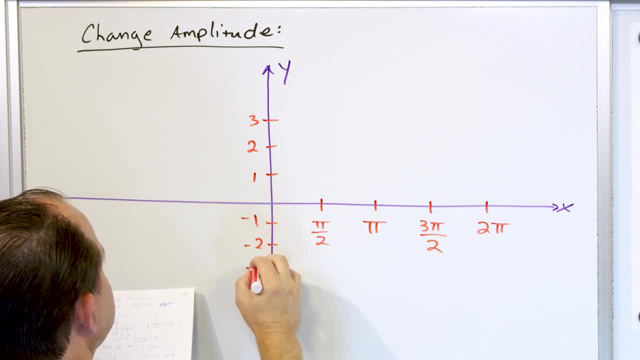 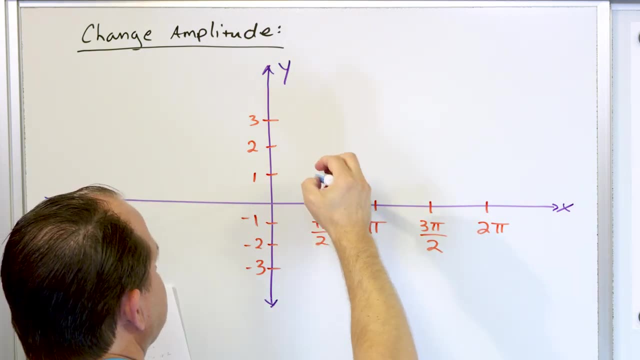 And this is negative, one negative, two negative, three Negative one negative, two negative, three. What's the baseline function? look like The baseline sine function. look like It goes up to a maximum of pi here, So it goes there, it goes down through pi. 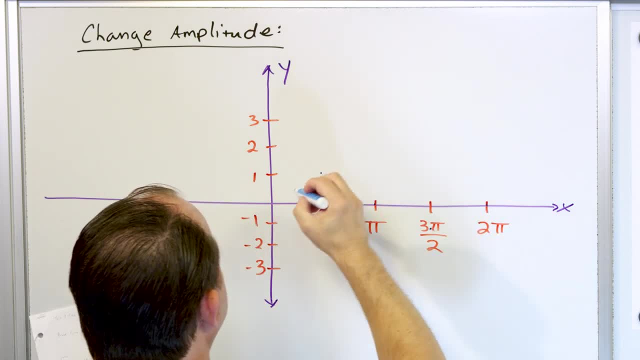 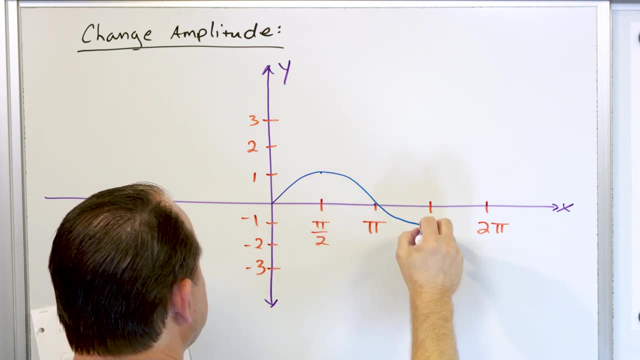 and then it goes right there and then back up to two pi. So if we could draw that without messing things up too much, we go up here and we go down, and we go down here and then back up, like this, That's how you would sketch it. 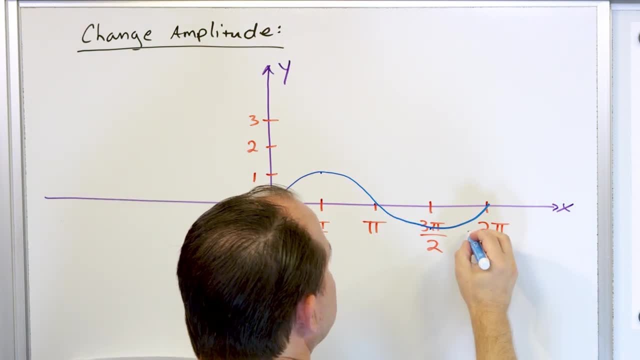 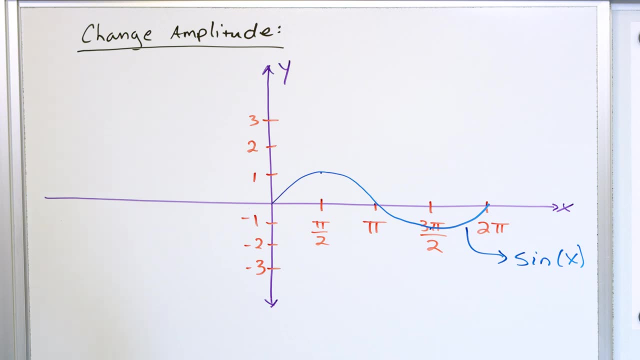 It's gonna look lumpy right, That's the way it is. So this is what The sine function. So what I'll do over here is I will say: this is the sine of X. all right, Now what if I wanted to make this thing larger? 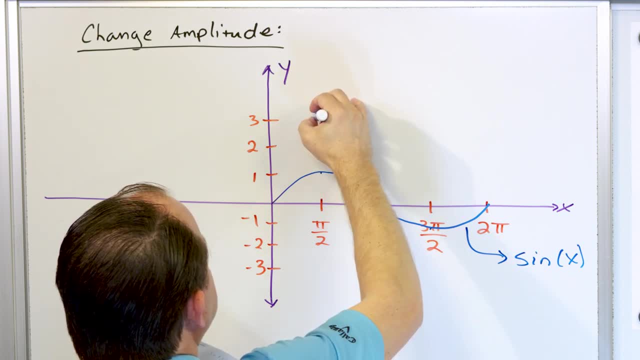 What if I wanted to make it look exactly the same, but go up to three, So it would go up to there, then it would go again through here and then here it would be down here negative three, and then it would be up here. 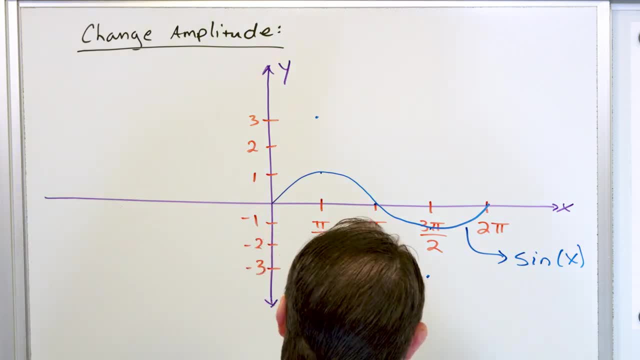 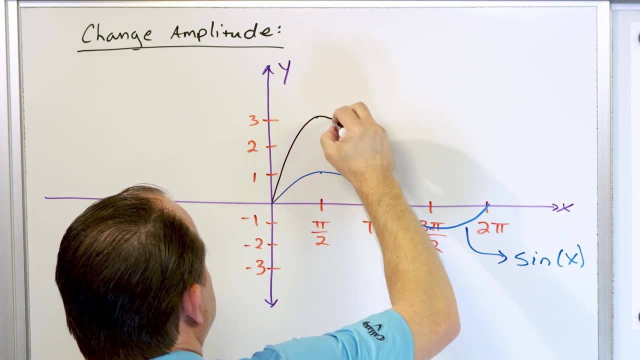 Then the graph. let me switch. let's switch colors to black, I suppose. So we'll go up here. it'll go something like this: It'll go up like this, then it'll go down through like this, then it'll go down like this: 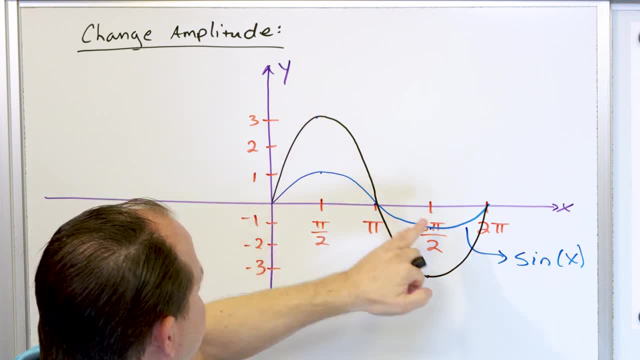 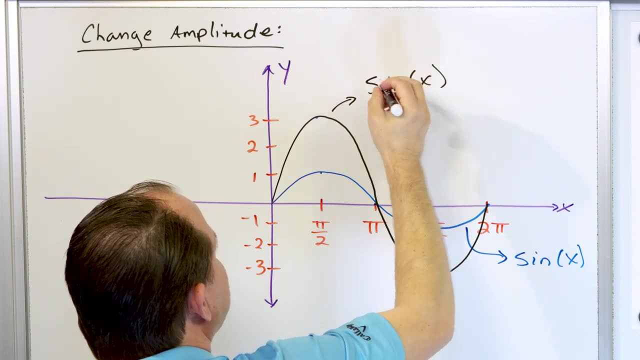 and then go up like this: Notice the crossing points are the same, the maximums and minimums are all lining up. What is this function? This is the sine of X, with a modification. What's the modification? The modification is that I've multiplied. 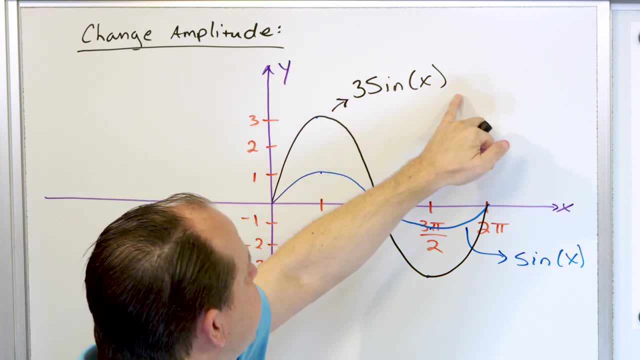 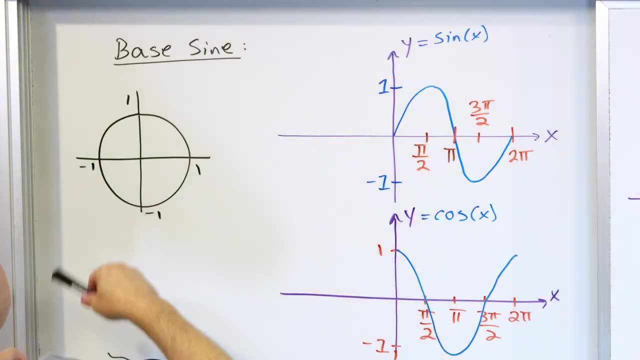 the entire function by a number three. because the sine function only returns plus or minus one. Why does the sine function only return plus or minus one? Because on the unit circle, whatever angle I choose, the sine is the projection on the Y axis. 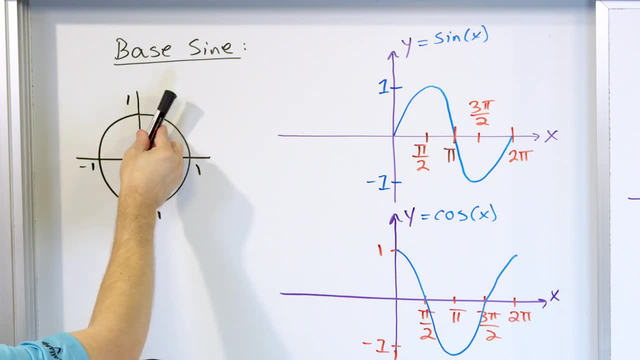 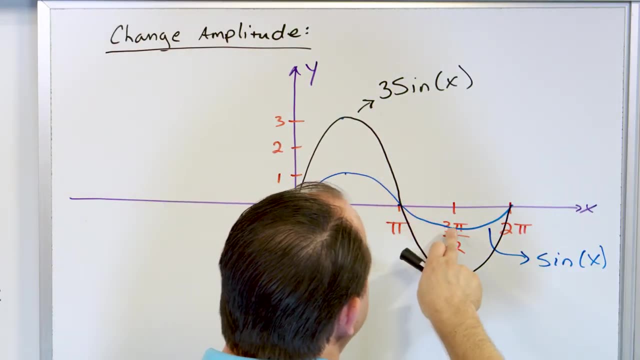 sine's projection on the Y axis. But since it's a unit circle, the most it could ever give me back is a one, and the least it could ever give me back is negative one. So the amplitude of this can only go between those points like this: 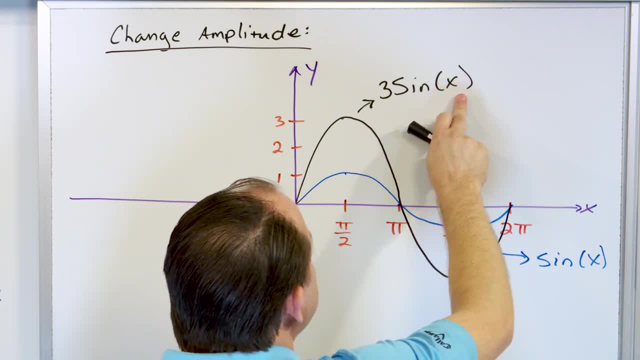 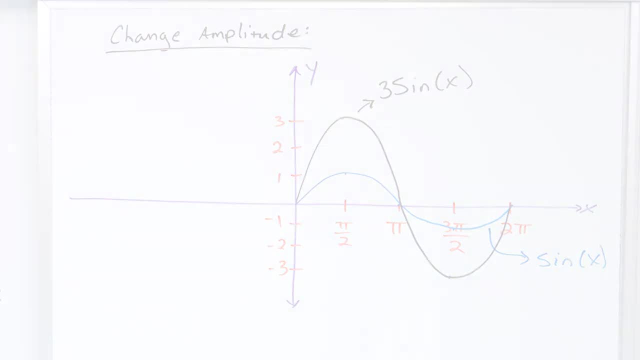 But if I take the output of this, which can go plus or minus one, and I multiply by three, then it can go up to plus or minus three, which is exactly what we have drawn right here All right now. we save the best for last. 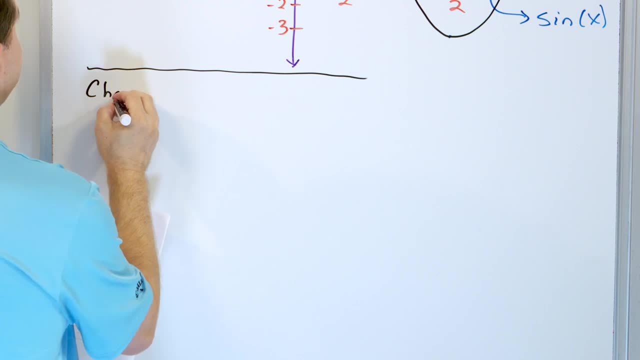 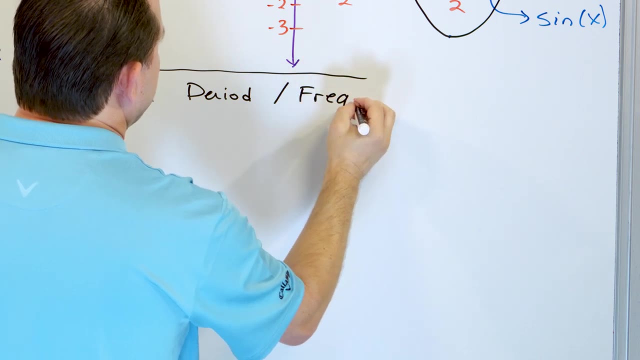 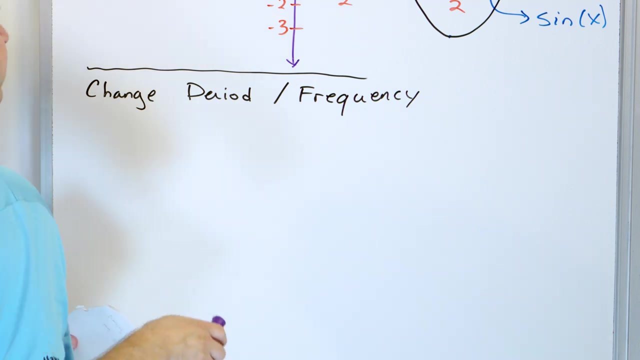 the one that gives the people the most trouble. but we'll try to make it very simple. Let's now change the period, also the frequency, because the period and the frequency are basically different words, different ways of saying the same thing. that we change the number of wiggles that are in this thing. 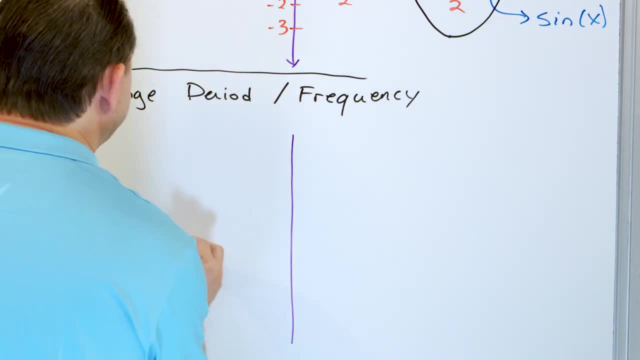 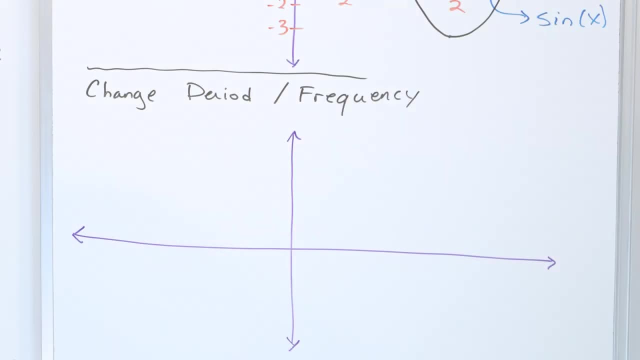 So let's go ahead and draw a nice big X- Y axis. When I'm done drawing these, I'm gonna show you the pretty graphs of all of these so that you can see a nice version of them as well. All right, so let's take a minute. 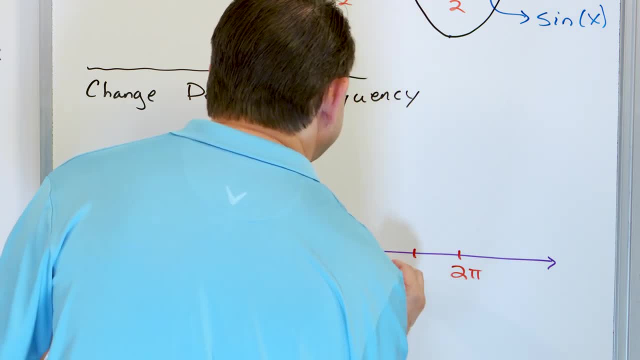 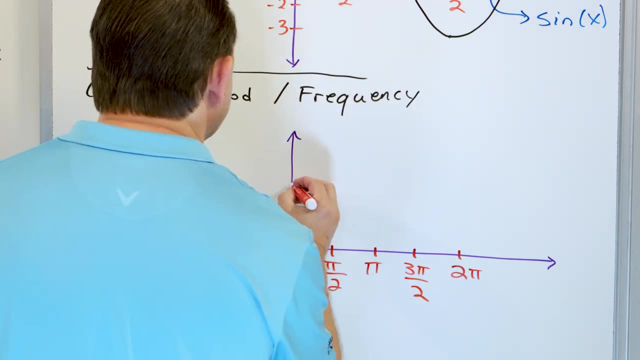 to draw our important numbers. So we have two pi half of that is pi, half of that's pi over two. and then this one must be three pi over two. So it goes up to a maximum of one and a minimum of negative one. 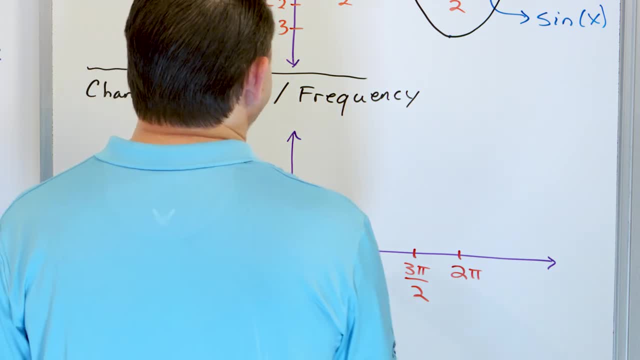 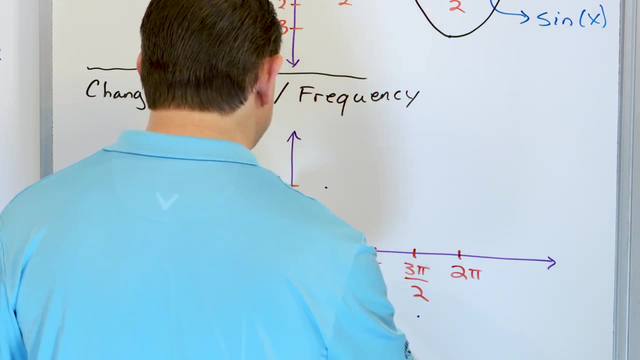 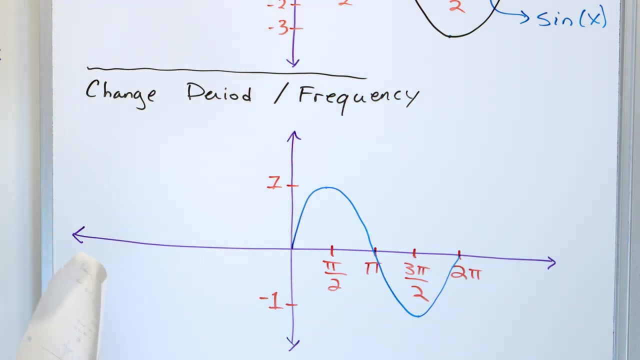 Let's first draw the baseline function. Hopefully you'll get used to doing this. The baseline function goes maximum, then zero, then it goes through minimum here and then back up to zero. So the baseline sine function goes up and then down and then up, like this: one cycle and two pi, all right. 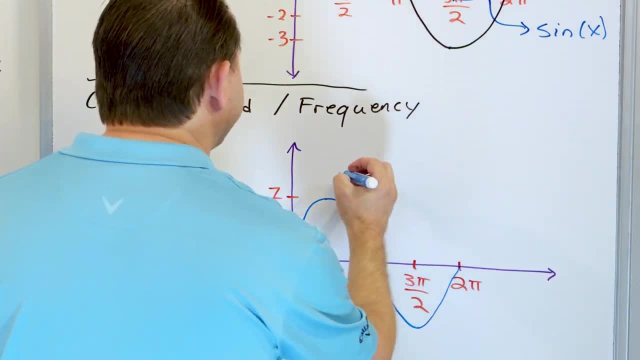 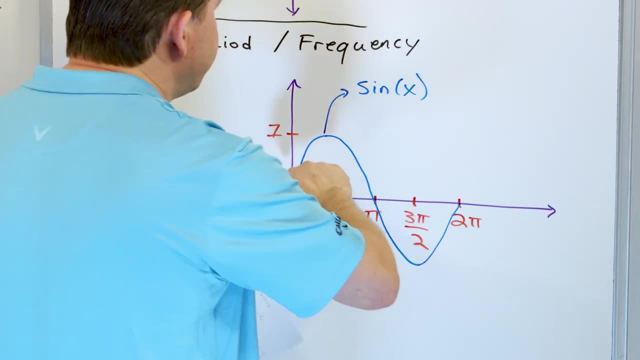 Now what we're trying to do is change the number of wiggles here. So the actual function that we have right here is sine of X. All right, what we're gonna do is what if we wanted to make this thing have two periods? 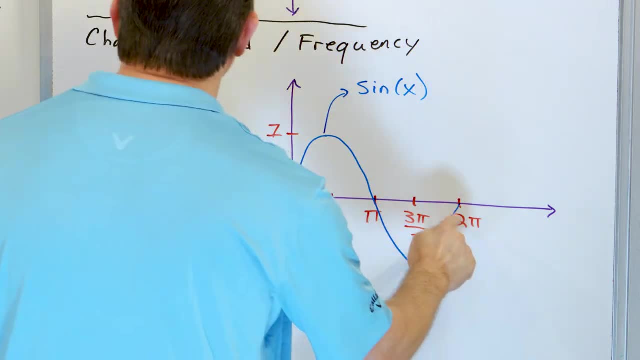 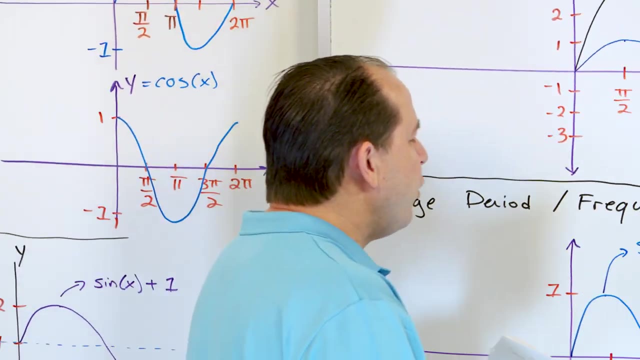 that exist in the same amount of angle, because, remember, the two pi here is the angle. That's the angle. Two pi radians means we've gone all the way around the unit circle one time. So what if, instead of having one complete cycle, 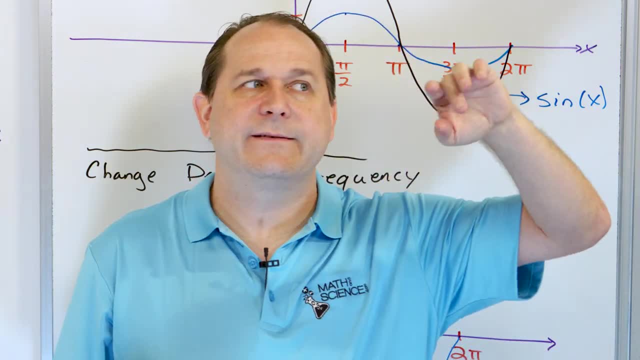 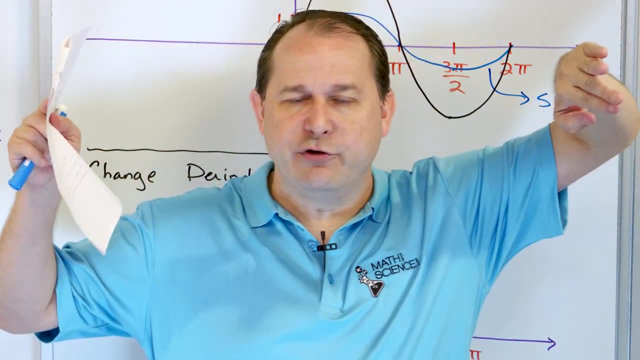 I wanted to have two complete cycles in the same exact region that the original graph takes. So the original baseline graph has one complete cycle and two pi radians. What if I wanted two complete cycles to exist there? And of course, you can go up from there. 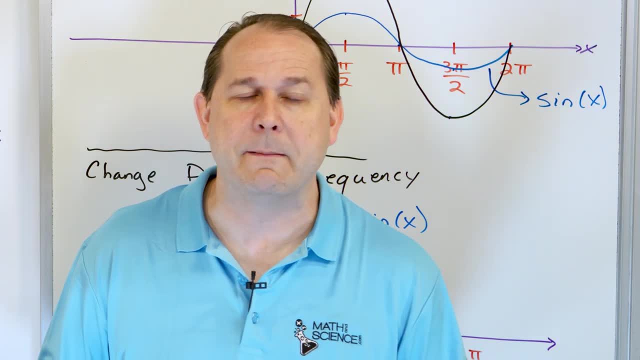 You can have a thousand cycles or a million cycles. You ever heard of that? You ever heard of a megahertz? right, That's a million cycles per second. in that case, We'll talk about that's more of an engineering. 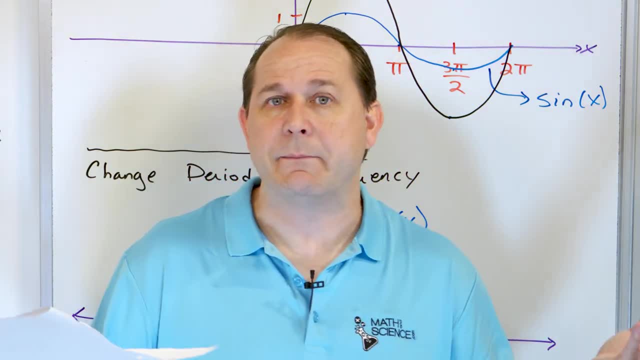 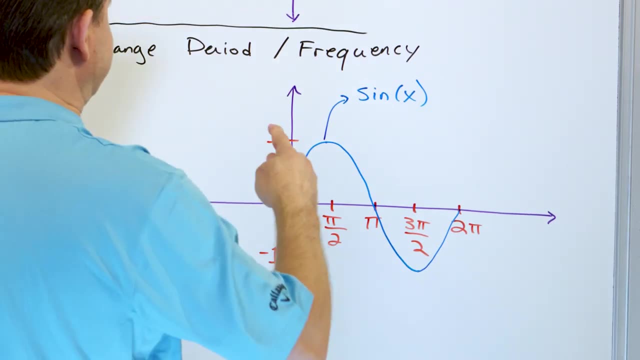 but it's the same thing. You can have millions of cycles happening in the same amount of time, for instance. So how do we do that, Or what would it look like before we actually graph it or before we actually write anything down? 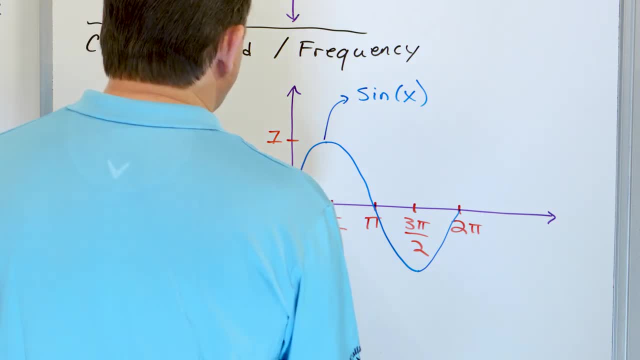 What would it as far as the equation, what would it actually look like? Well, what would happen is, since this one goes here, then I would expect the new one. it would have to reach some maximum right here and then it would have to go through zero right here. 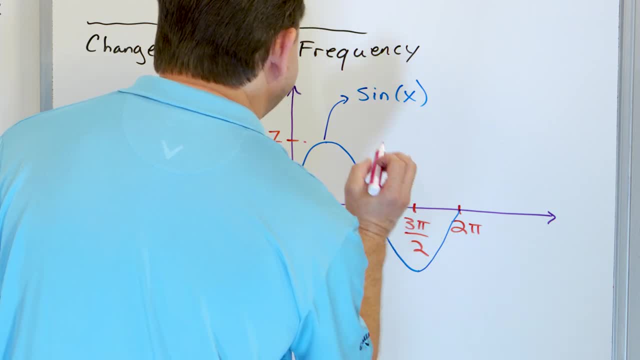 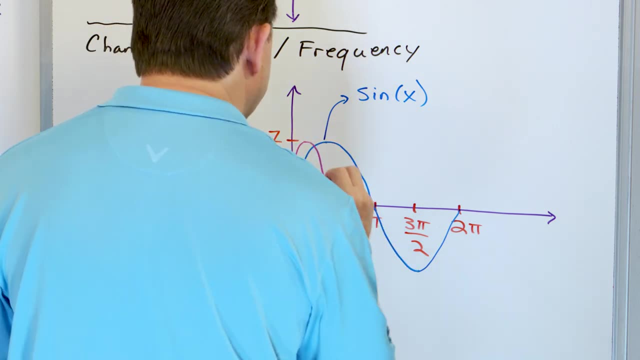 And then it would have to reach a minimum right here and then it would have to go up right here. Let's just draw that part of it and see what that looks like. It would have to go up very steeply. Then it would have to go through zero, right. 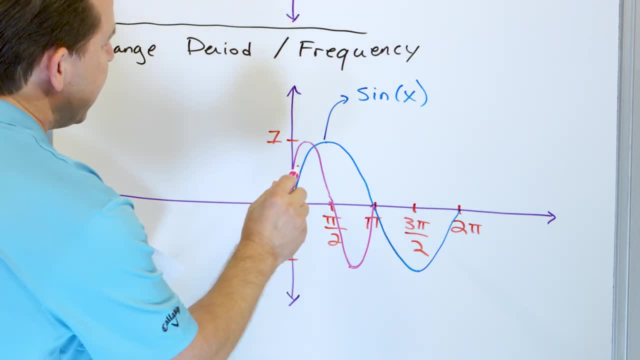 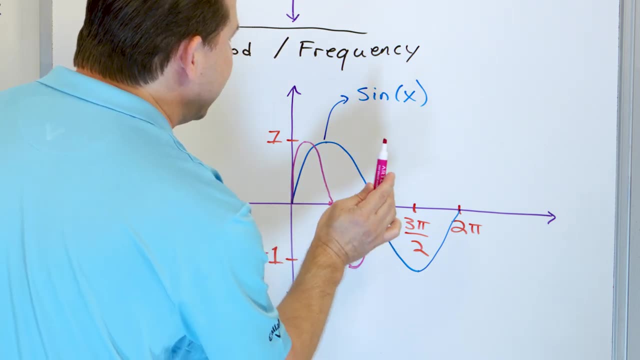 Then it would have to go down here and then it would have to go here, Because in the original graph it goes once: this is a half of a cycle, but it completes this other one completes a complete cycle in the time or in the angle that the blue curve. 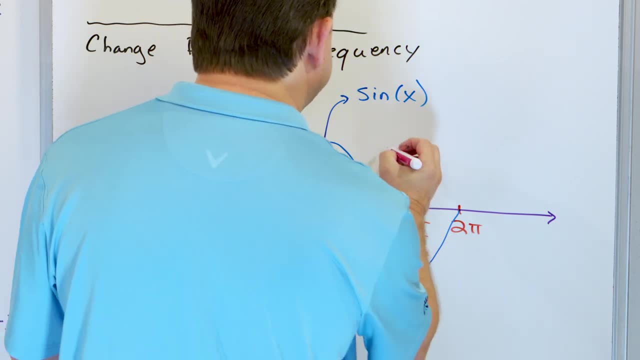 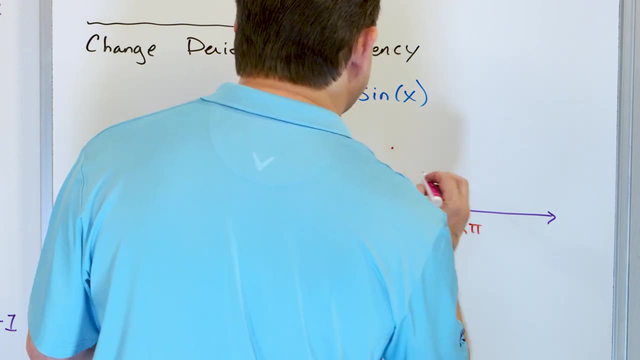 takes only half of a cycle, Then the thing would continue on and do the same thing here, So it would reach a maximum somewhere around here, then right around here, and then a minimum would be somewhere right around here, and then it back up like this: 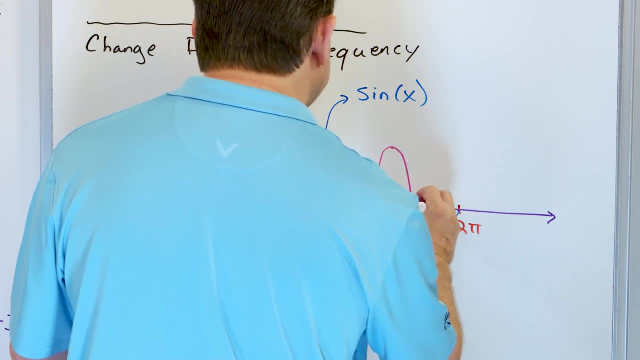 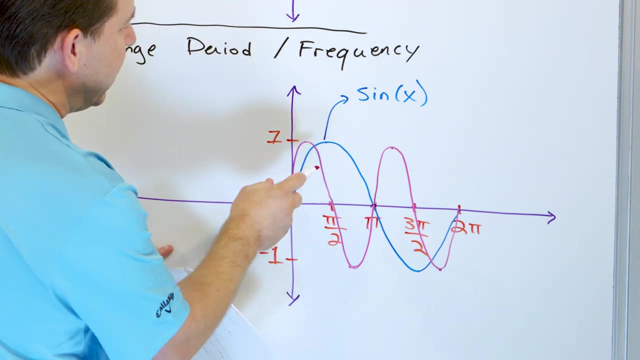 So it would go up to a maximum and then it would go down, like something like this, to a minimum, and then it would go back here. Do you see how the purple curve? and I know it's hard to read, but that's life sometimes. 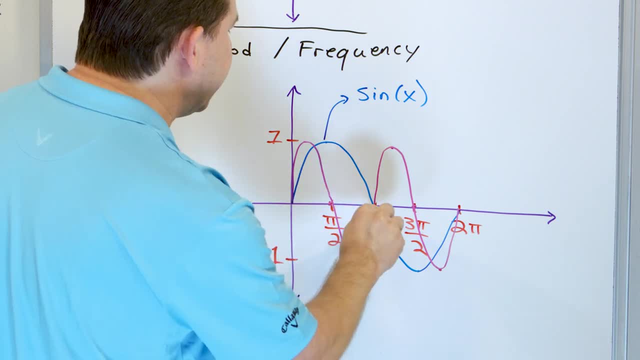 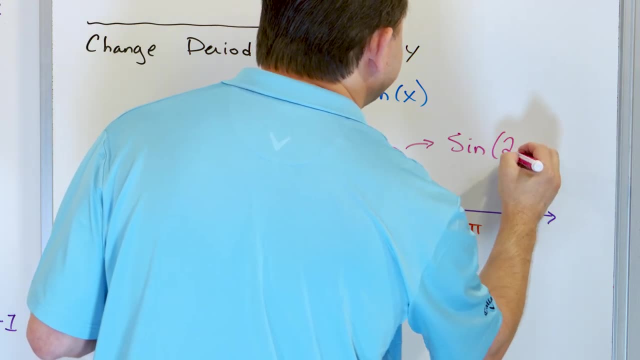 The purple curve. there's one complete cycle here and there's another complete cycle here. What would be the equation of this? It will be the sign of, according to the computer demo which we just did, two times x, So the number that exists in front of the number x. 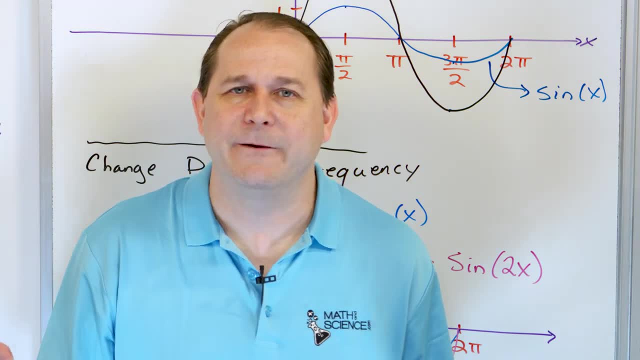 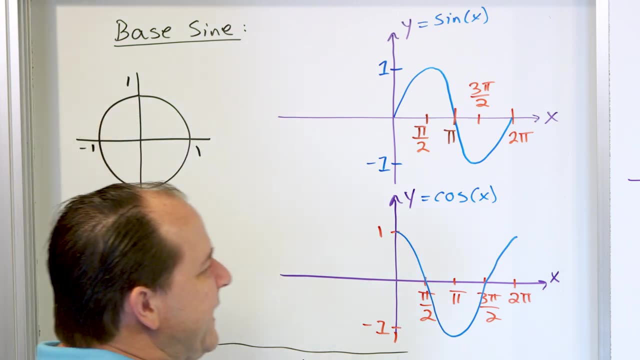 or the angle is sort of like a speed multiplier. That's like the best thing I can describe, Because over here you're going around the unit circle two pi radians. But if I put a number in front of the variable, that represents the angle. 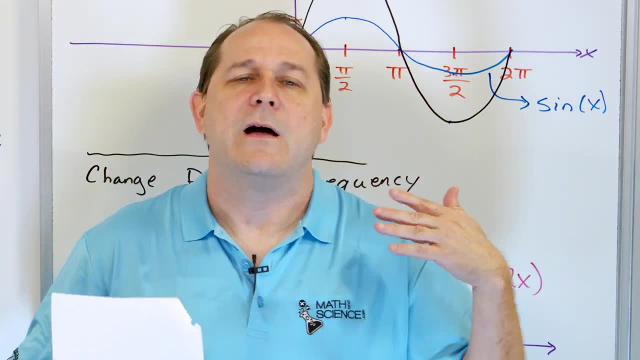 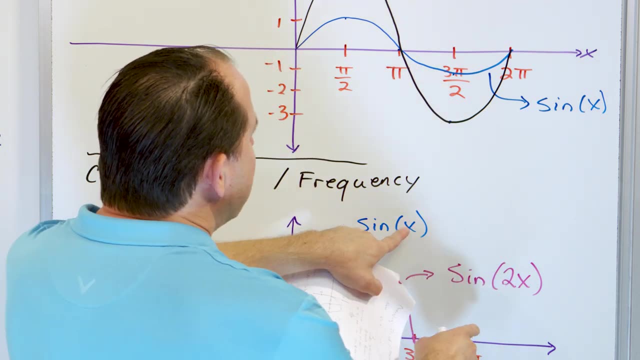 it makes it go around the unit circle two times faster. I'm gonna say that again, It go arounds two times faster. And when I say two times faster compared to what? If I compare these two functions? In other words, let's say I've got an input variable here of pi, radians. 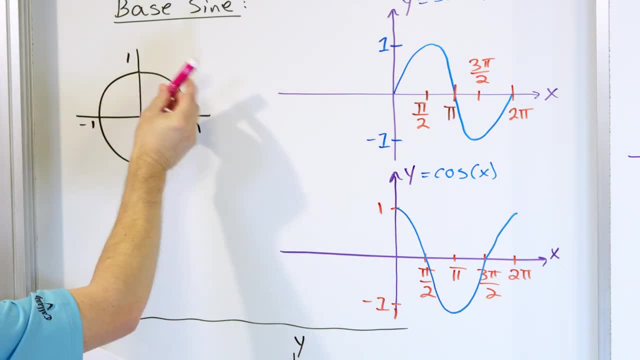 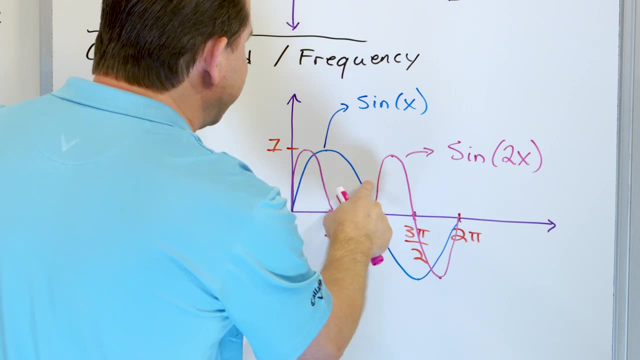 Where is pi radians on the unit circle? Pi radians is just halfway around. that's what pi radians is. So here this function. if I put pi in here, it only goes half around the unit circle, which means it completes half of a cycle there. 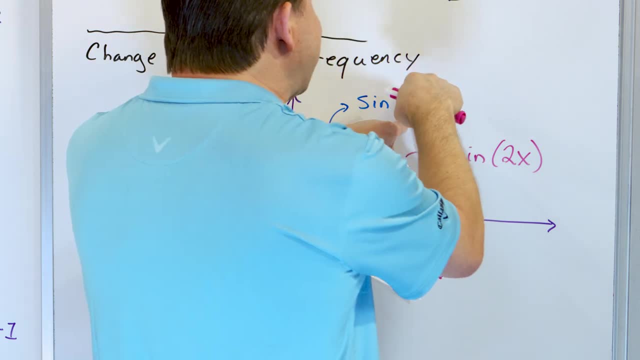 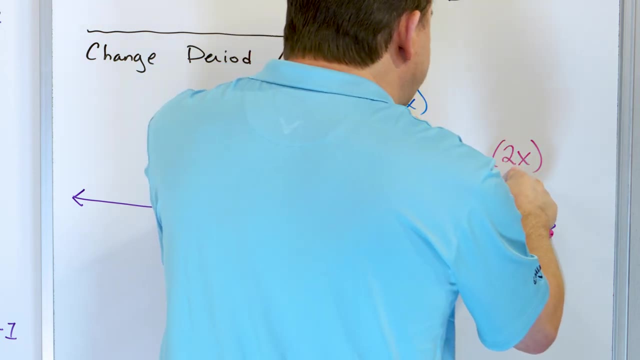 And that would be the blue curve would stop right there. But if I take that pi radians and I put it into the second function, then it's pi times two, which is two pi, which I'm taking the sine of two pi. and basically a sine of two pi is a is a sine of two pi. That's called the two pi, which is times pi, times two, times two pi, And I'm taking the sine of two pi and basically a sine of two pi. 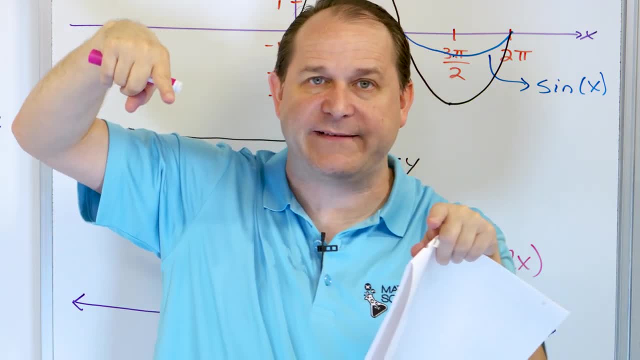 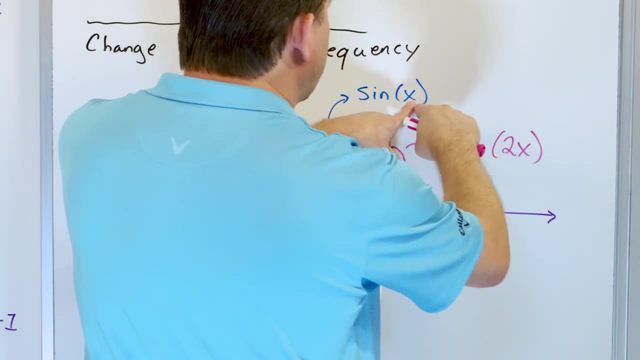 sine of two pi is as if it had gone all the way around in that second function, And so sine of two pi is again zero. So basically, at the same exact point where this one only went halfway around, this one went all the way around the unit circle. So at this point, when the input was pi, radians. 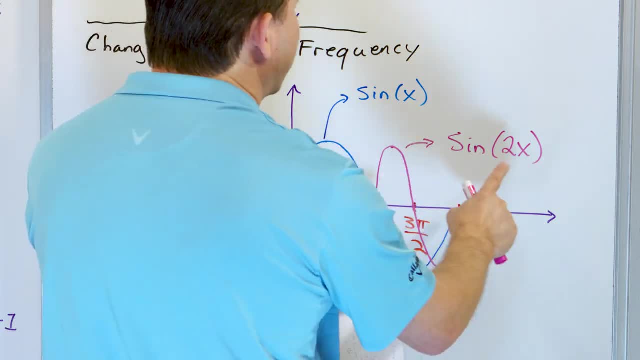 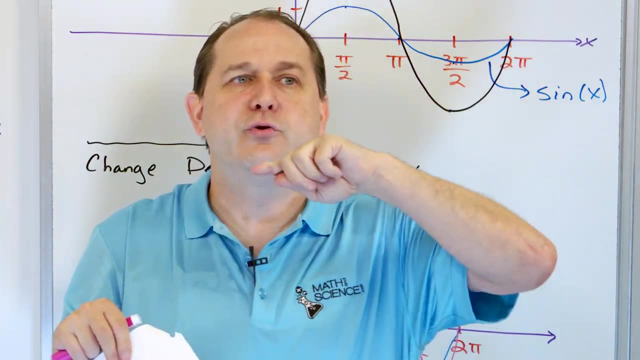 the blue curve got halfway around, but the pink curve went all the way around. Basically, like I say, it's a speed multiplier because you don't have to increase the input value of x very much to complete one circle of the unit circuit, of the unit circle. And when you go around once in the 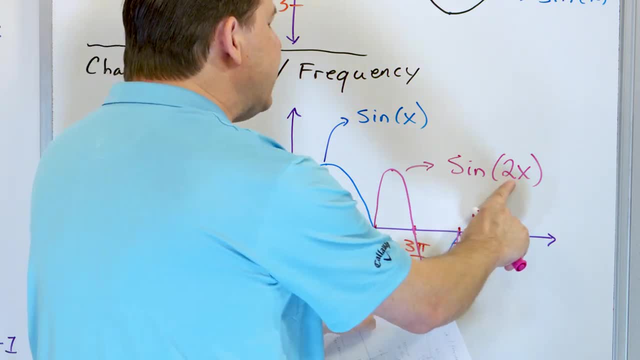 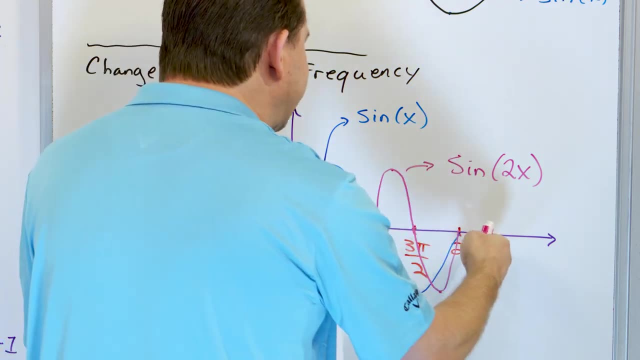 unit circle. you complete one cycle on this graph. So the number that you see here is literally telling you how many complete cycles you have inside of a two pi region where the baseline graph exists. That's why I was telling you it's important in your mind to have a baseline graph. 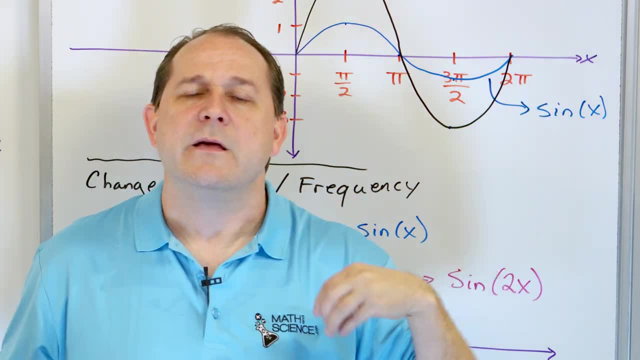 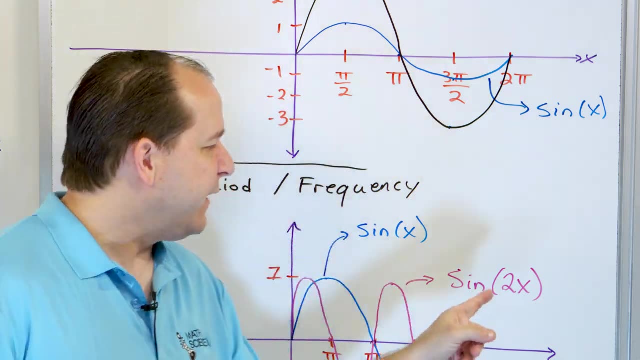 The baseline for the sine and the cosine have a period of two pi, Then if you modify it by adding a speed multiplier right in front of the two pi, then you have a period of two pi And so the variable. then you know: okay, there's got to be two periods inside of the baseline time. 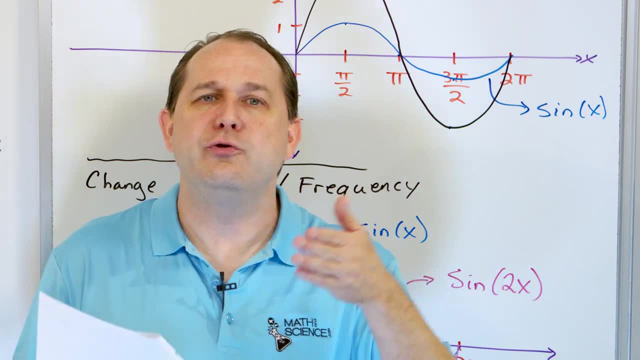 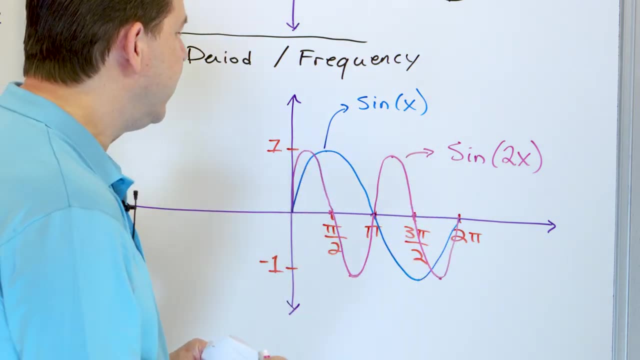 timeline for sine, which is two pi, So two periods in a two pi time. And that's what we have. If I put a three here, there would have to be three periods that would exist in this same window here. If I put four or five or 10 or 15 or 20, it would be that many number of periods that would exist in. 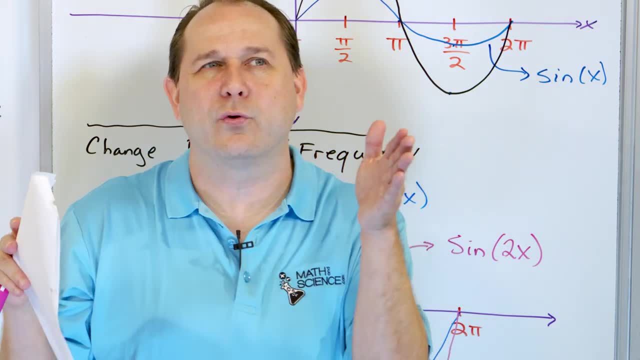 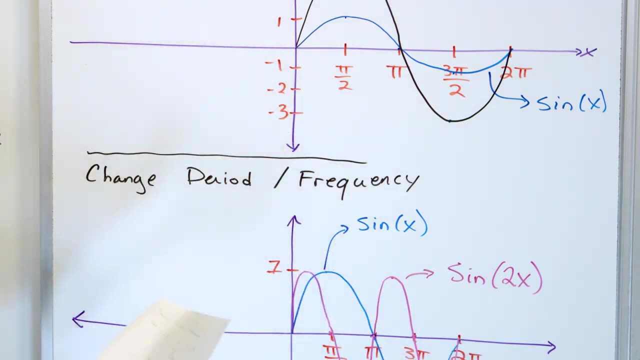 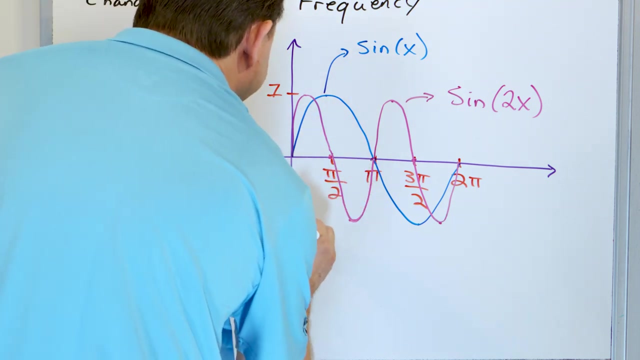 that same default window for the default. So everything is sort of like, based upon what the default sine function exists And does as a behavior, All right, The next thing I'm going to write down here I'm going to put- I'm going to shorten this because we're going to use this in our problems here, right? So what I'm? 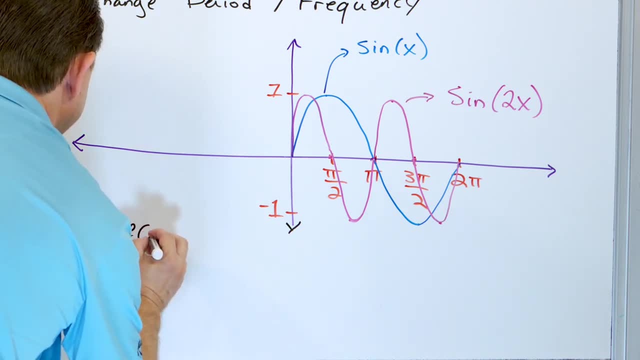 going to write down. here is four. four. F of X is equal to the sine of B X. Now don't get so scared, right, B X. All I'm saying is I'm modifying the sine function. So there's a number, B is a constant. 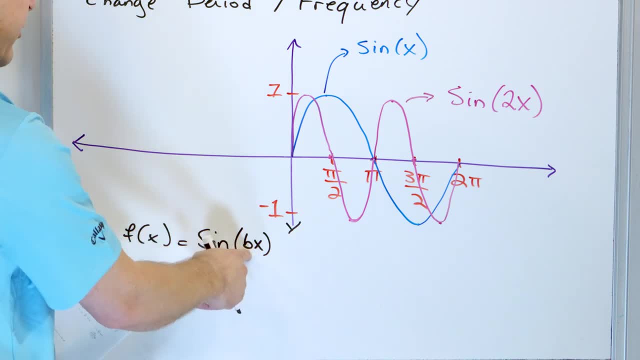 in front of the variable and the constant. I'm allowing myself to change. So I'm modifying the sine function. If I make B one, then it's just sine of X, which is the baseline default sine function. But if I put two in here for B, I get this one. If I put three, four, five, six, seven, 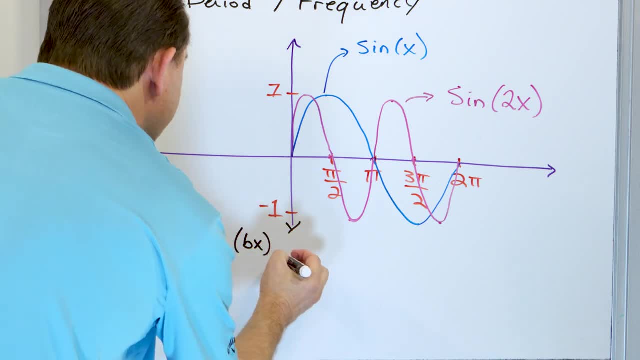 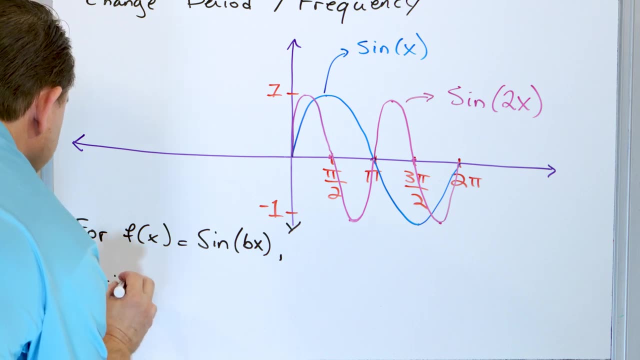 I'm just increasing the frequency, like we've been talking about, right? So when you have a baseline function like this, then what you can say is the period of this function. the period of this function is equal to two pi divided by B. right, This is a handy, dandy little formula that. 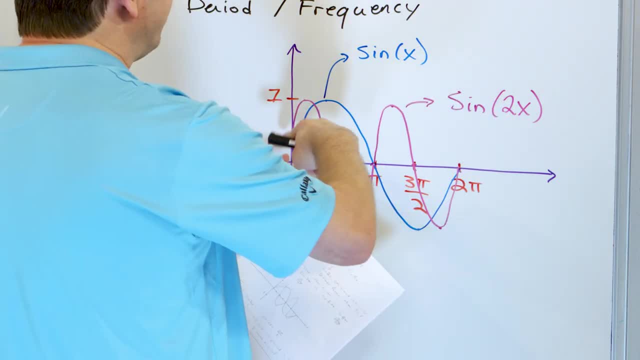 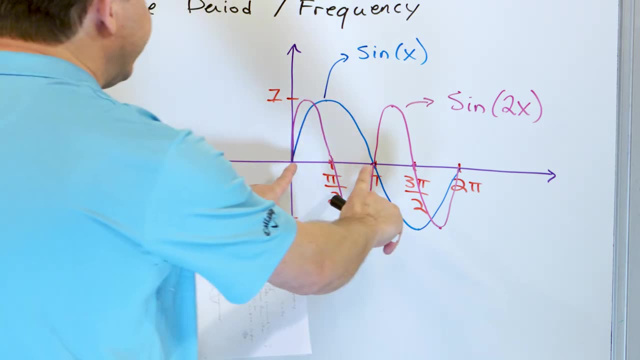 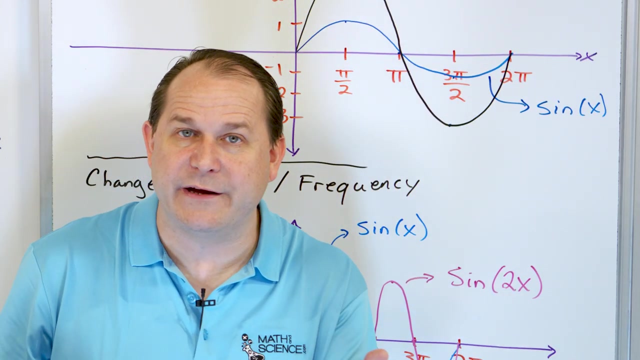 whole time is that if I put a speed multiplier in here, then I must have two complete periods in the baseline default period here, In other words the new period. notice: the new period is only pi for this one. here The reason that the period is pi is because it's half of the period. 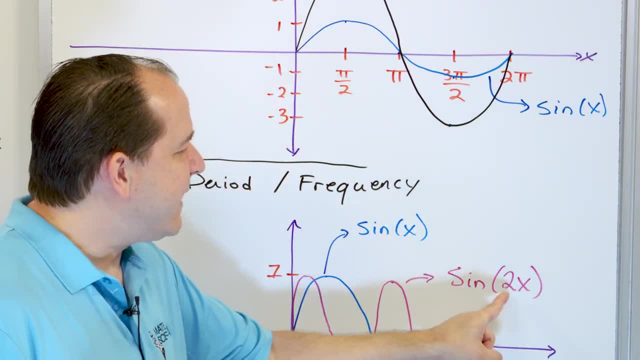 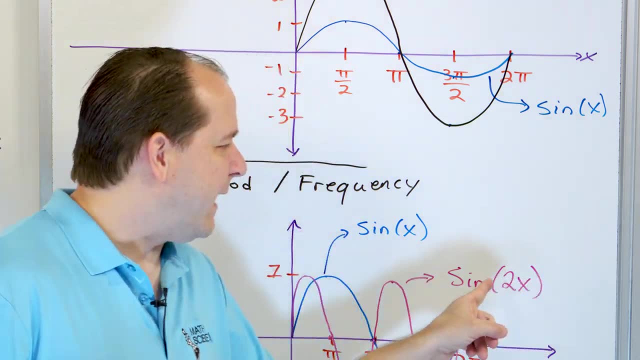 of the original baseline function. So another way of looking at it: instead of a speed multiplier, you can look at it as a period reducer. Think of it that way: a period reducer, but not reduced by a factor of two. it's really a factor of one half. 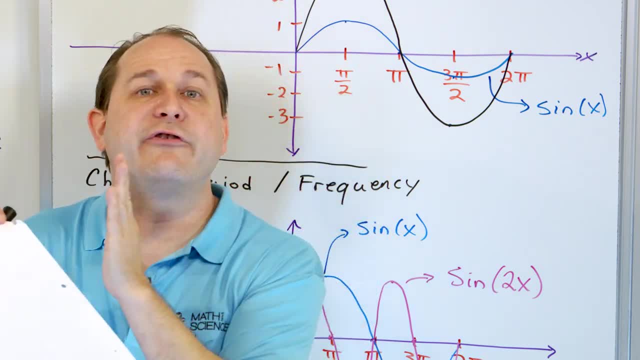 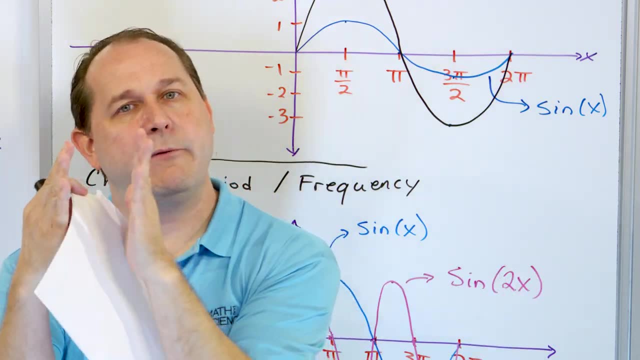 So the bigger the number is, the more waves are squeezing in there, the smaller and smaller the period is. You see how period and frequency go together. Higher frequency means higher wiggles. At the same time, the period gets smaller by the same factor. 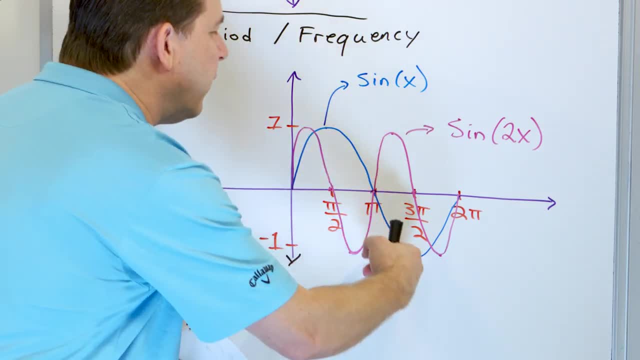 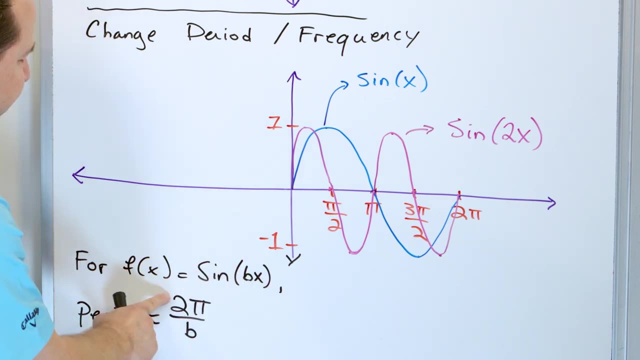 So the new period is two pi, because that's the default period cut down by whatever this factor is. So if you put a factor of two in here, then it's two over two. they cancel and the period is pi. That's exactly what I have here. 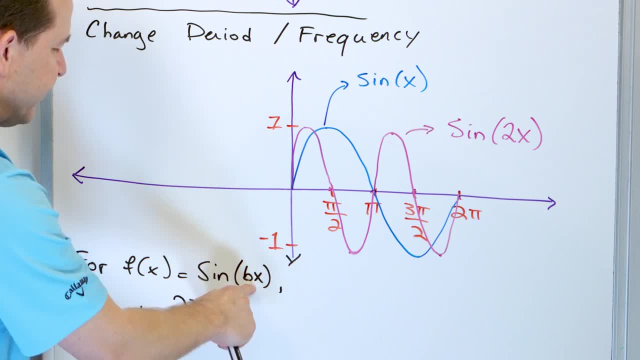 If you put a four here, so it's sine of four times x, then it'll be two pi over four and the period. so you have a two and a four, it'll be pi over two, the period would be pi over two. 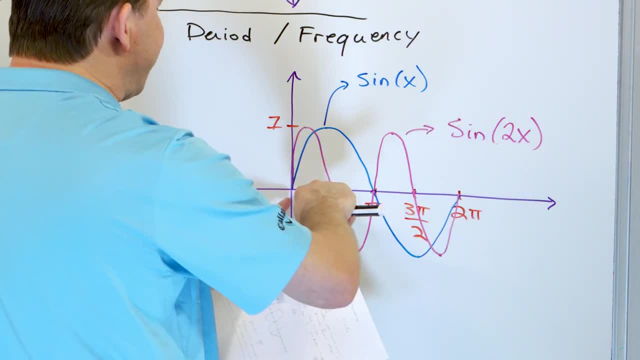 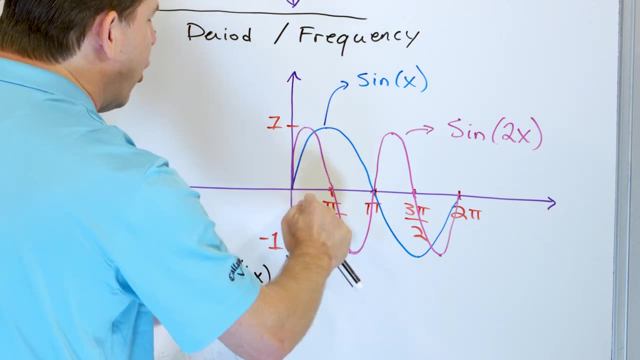 So if I doubled it again and made sine of four x, the period would have to all exist. instead of this wide, the period would be cut in half again, so it would have to be a whole cycle inside of pi over two. So what you're doing when you look at this formula. 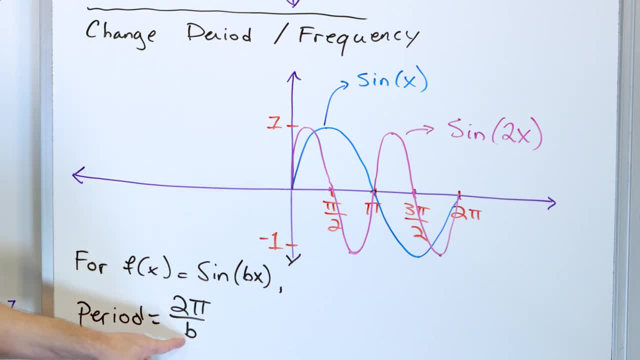 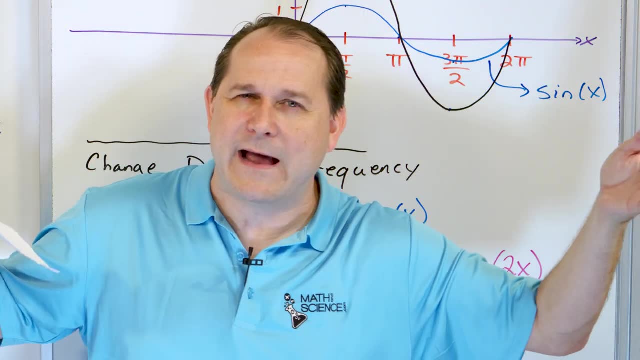 is you're taking the period of a default sine function and you're cutting it down by whatever this factor is, because that factor is alternatively telling you how many cycles you have in that window. So if you have five cycles in that window, the period must be cut down by five. 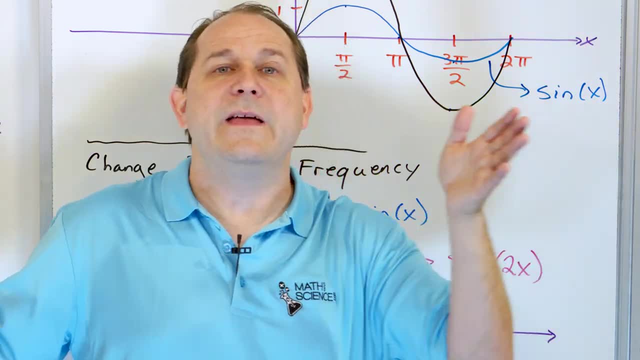 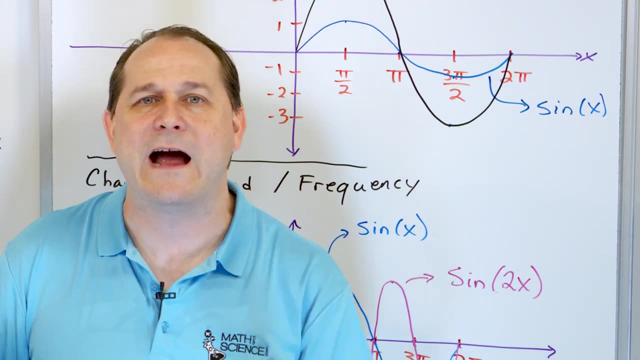 If you have 10 cycles in that window- a lot of frequency- then the period's cut down by a factor of 10.. So this new period is the original period divided by this factor, this chopped down factor of basically whatever this is telling you. 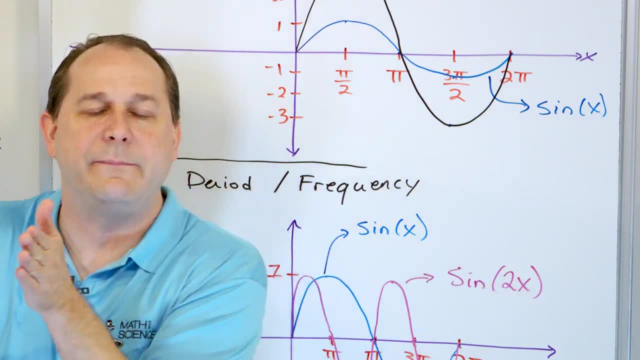 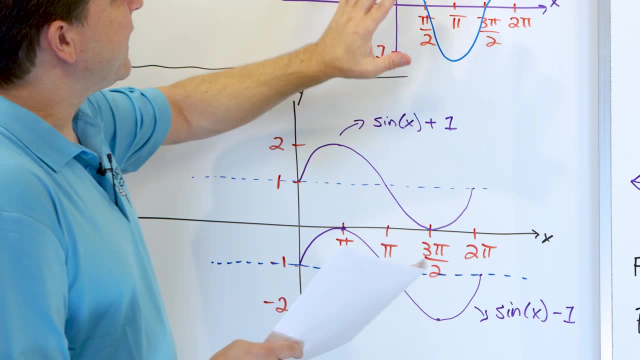 of basically whatever this is telling you of, basically whatever this is telling you. It's telling you: the period has to be that factor smaller. That's really what I'm trying to say here. So here we've done the shifting sine up and down. 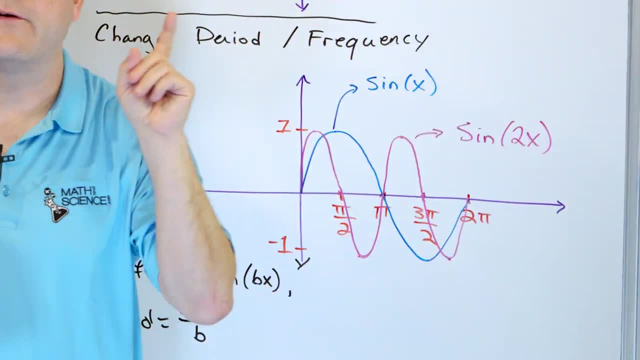 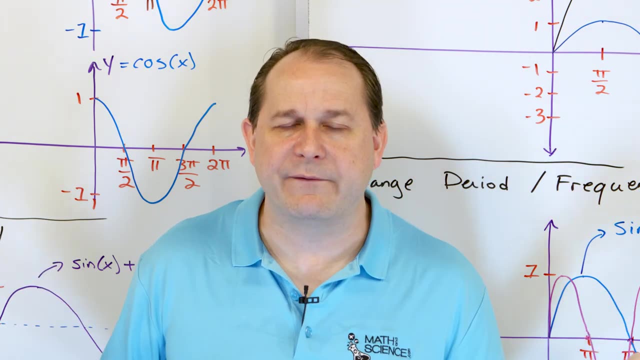 we've done the changing of the amplitude, we've done the changing of the frequency, Before we solve our problems, I've drawn these on the board. but I wanna show you a pretty- I say pretty- a nicely drawn computer graph of each of these, so that we can 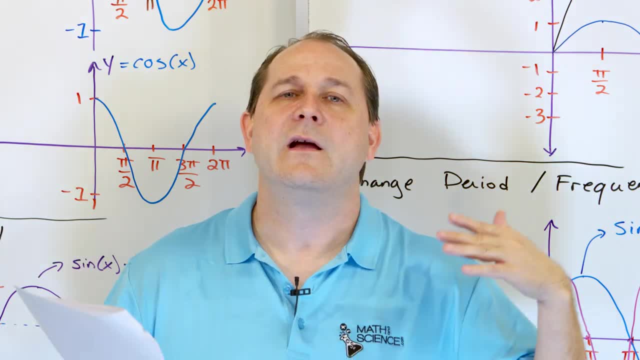 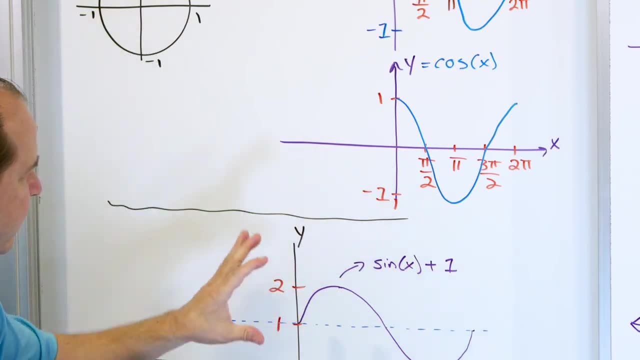 so that my little sketches don't confuse you, because there's irregularities in my sketches- I'm gonna show you what they look like beautifully and then we'll solve a few problems. All right, so for our first, the thing we did first is we took the sine function. 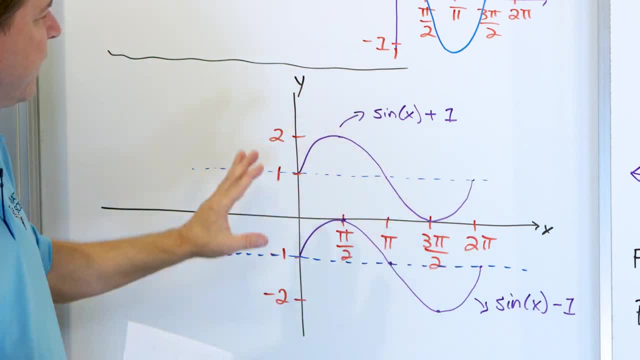 we added one to it. we got something like this: we subtracted one, we shifted it down. I know there's irregularities in my graph, so I do wanna show you what the pretty version of that would look like. This would be the sine function. 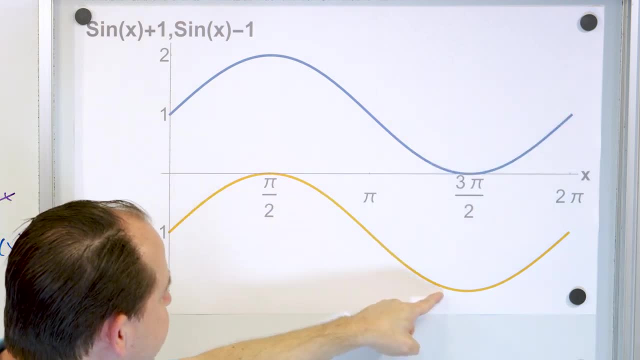 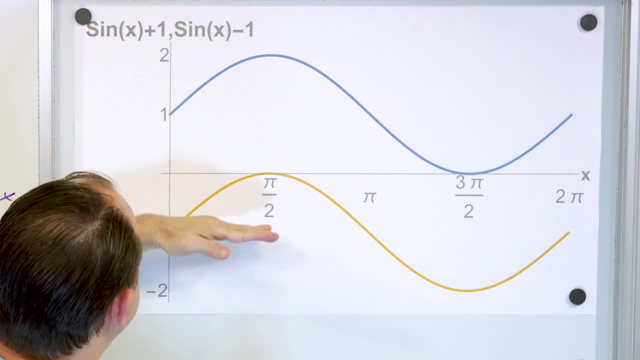 If you shift it up by one, this would be the sine function. if you shift it down by minus one, Notice that the middle of this graph right here is at the one position. That's like if we shifted the thing up in the middle of this graph right here. 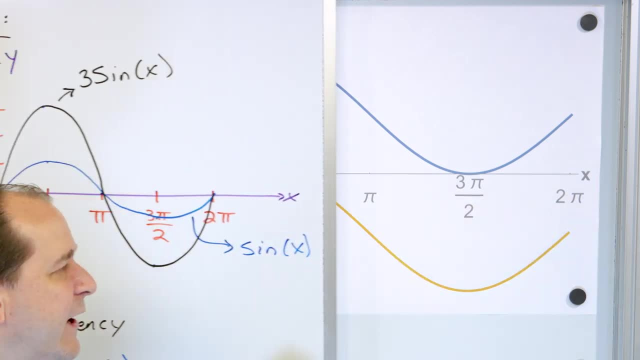 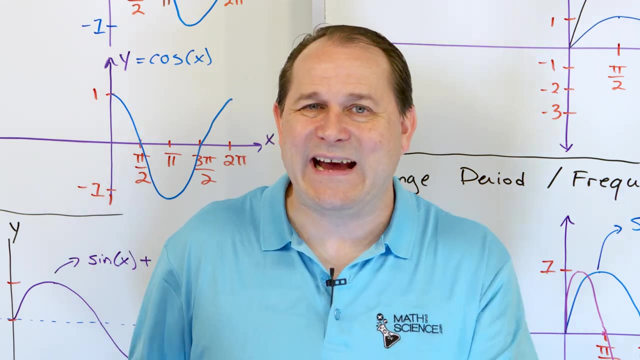 is at the minus one position, That's if we shift the thing down. Believe me, I could have saved a lot of time by not drawing anything on the board and just showing you computer graphs of everything. But I really wanted to draw it because when you're on an exam you have to draw it. 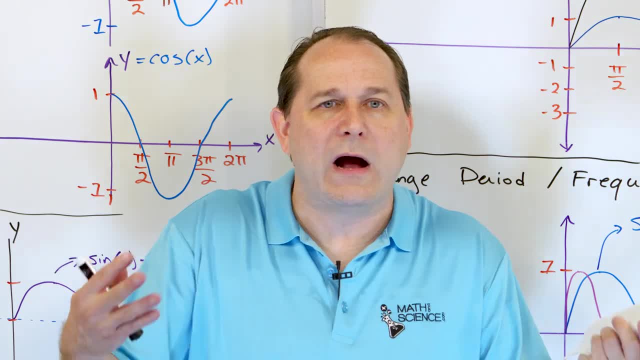 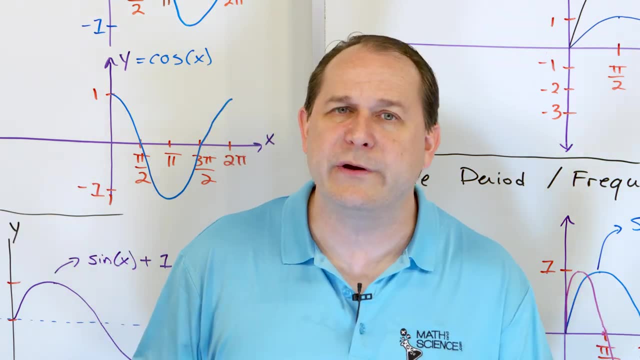 And so if you don't ever get any practice drawing it, then you can't do it, because just watching some computer graphs, no one gets good at that. So I encourage you to watch this lesson a couple of times, And when you see me sketch these graphs, do it yourself. 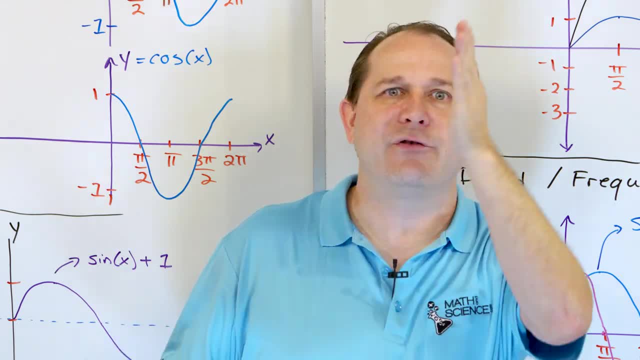 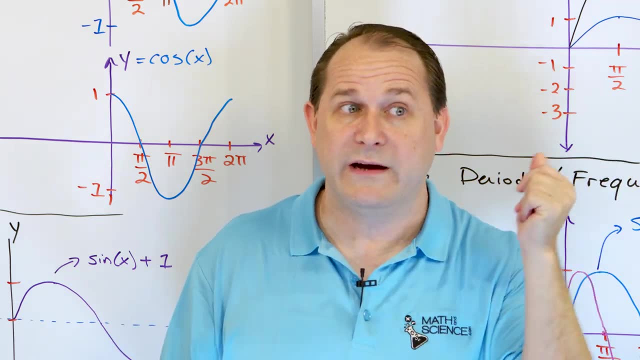 You don't get good at doing that until you write the pi over two pi, three pi over two, two pi, and actually sketching it maybe at 50 or 100 times, And then you will know exactly what these graphs look like. 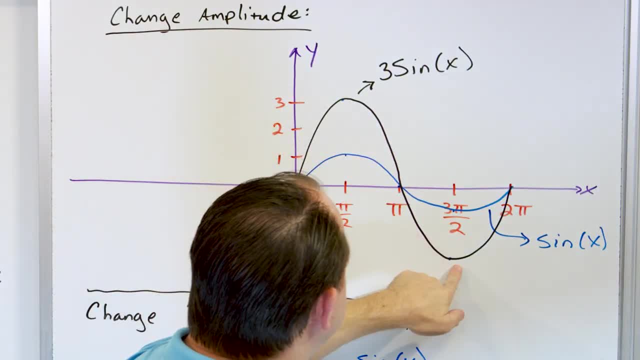 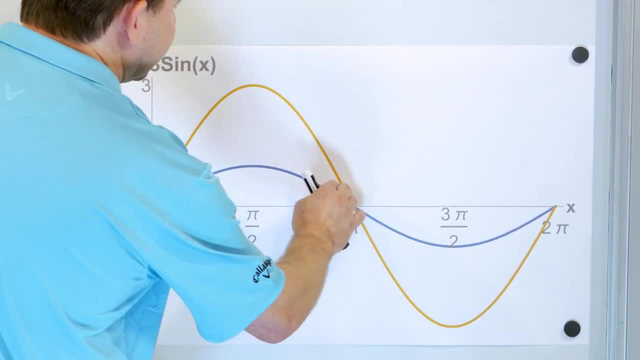 So we did that. The next thing we did is we changed the amplitude up to three, down to minus three, by putting a number in front. So what does that graph look like when it's beautiful Is well, here's the baseline: sine function. 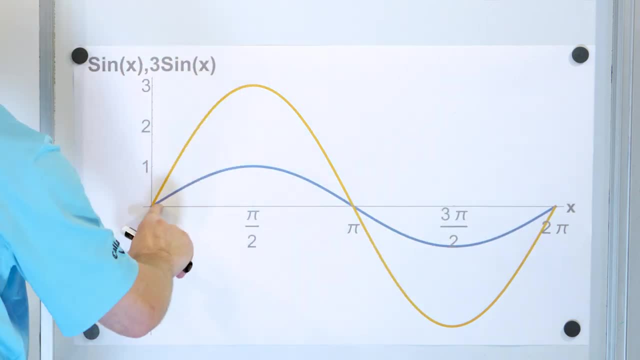 It goes up to positive one and down to minus one. The new function has all the same crossing points, goes up to positive three, down to negative three. Again has exactly the same period. All right, then. the next thing we did is we said: 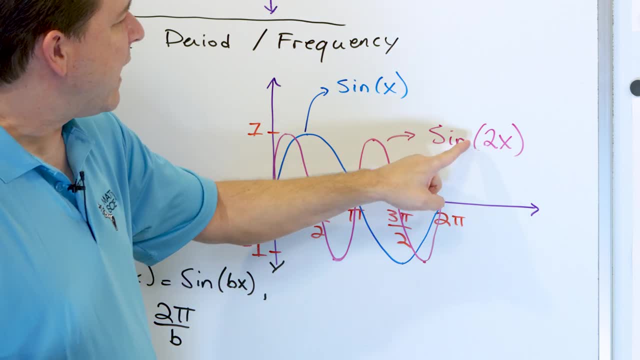 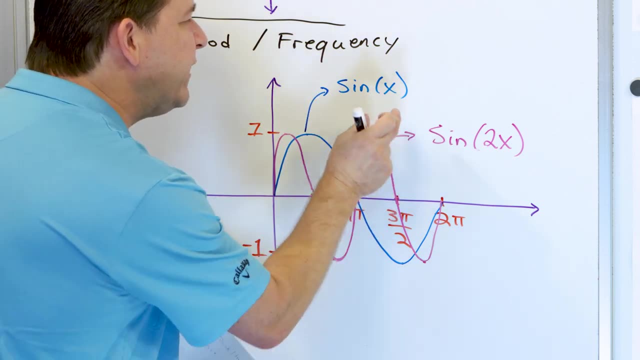 well, if we take a sine function and we put a number in front of the variable where the sine is acting on the product, this acts as a speed multiplier, So that now I have to have two complete cycles of a sine in the same window that the original function would. 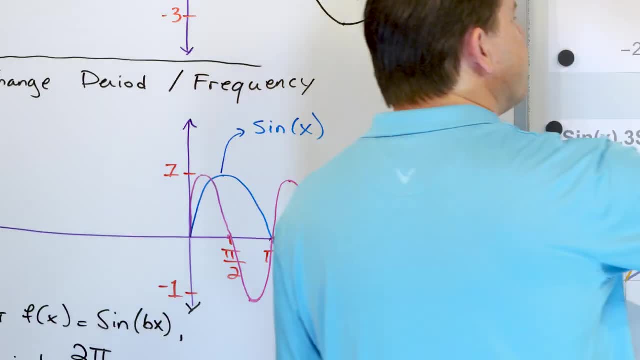 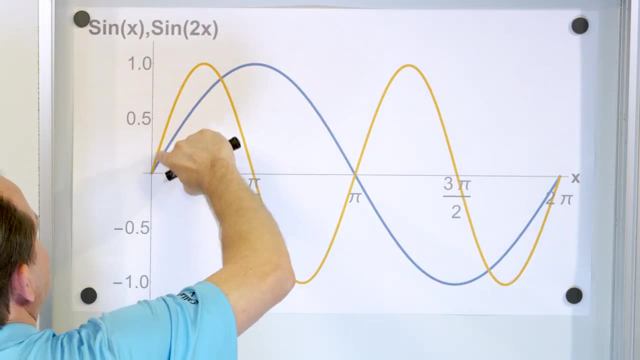 because it speeds up how fast I'm going around the unit circle. So the pretty version of that graph would look like this: The blue graph is the baseline sine graph and the sine of two X is this one. So here we have one complete period again at pi. 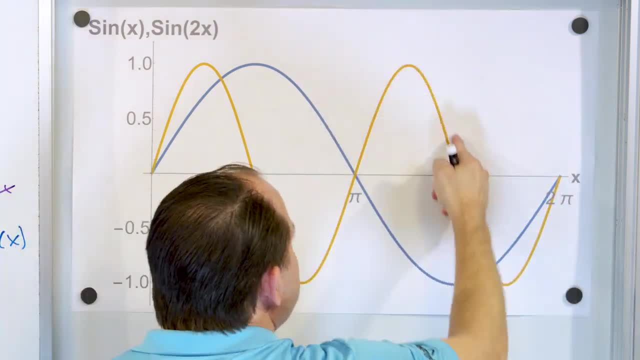 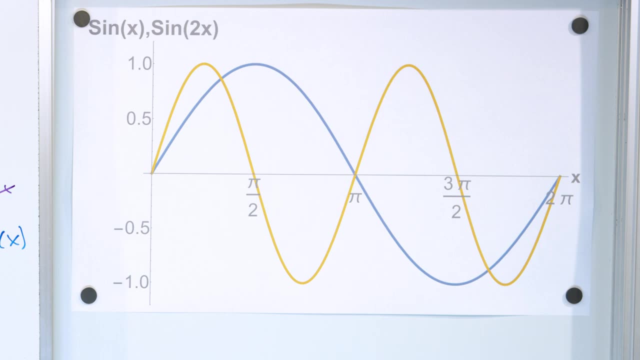 which is half of the period of the original function, And then we have another complete cycle. so we have two complete cycles in that window. So let me take these computer graphs down and we'll solve a few problems. All right, for our first problem. 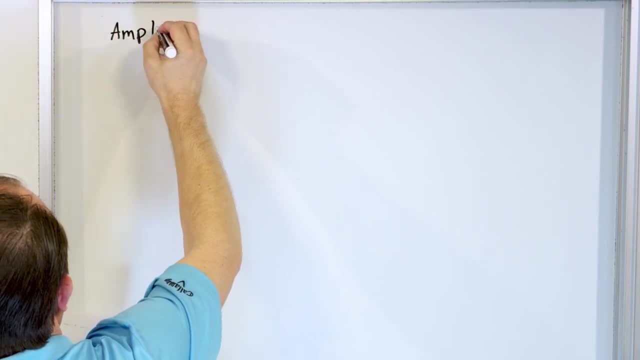 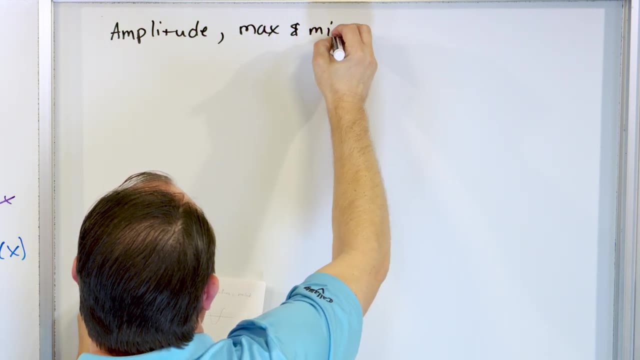 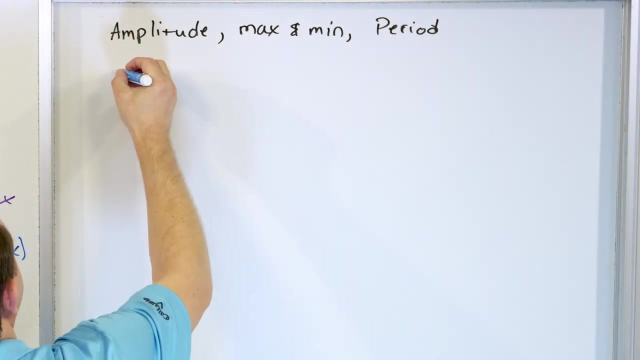 we want to list the following: We wanna write down the amplitude of the graph, We wanna write down the max and the minimum and we want to write down the period. All right, what's the function we're dealing with? It's F of X is equal to two times cosine of X. 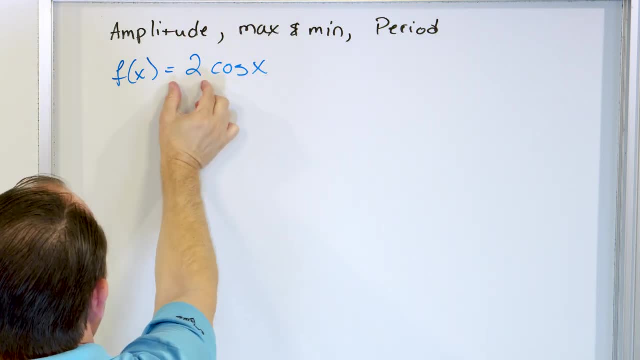 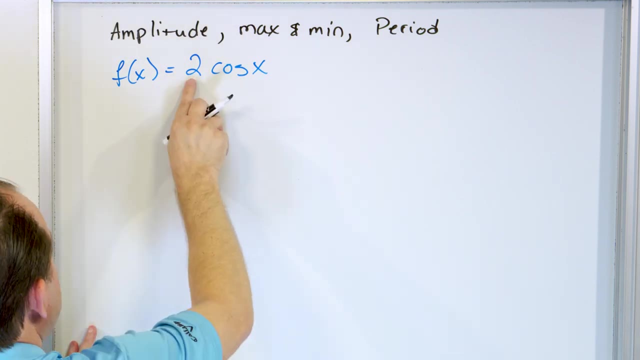 Now notice: the cosine is unchanged, It's just that we're taking it and we're multiplying it by two. So this is just changing the amplitude of the function, Right? so the new amplitude. if there was a one here, the amplitude would be one, but the amplitude here. 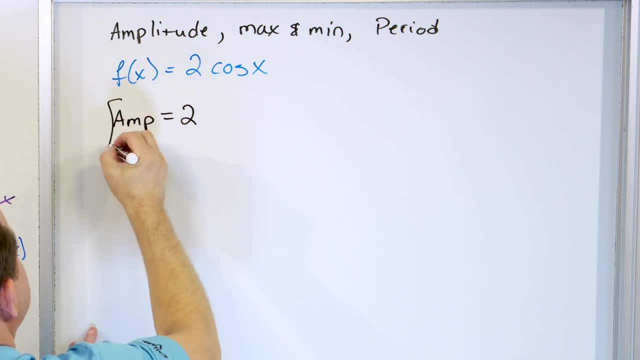 I'm just gonna put amplitude, and that amplitude is equal to two. That's the distance from the X axis up to the top there. And before we do anything else- maximum, minimum- let's go ahead and sketch this guy, Because doing a sketch can actually help us. 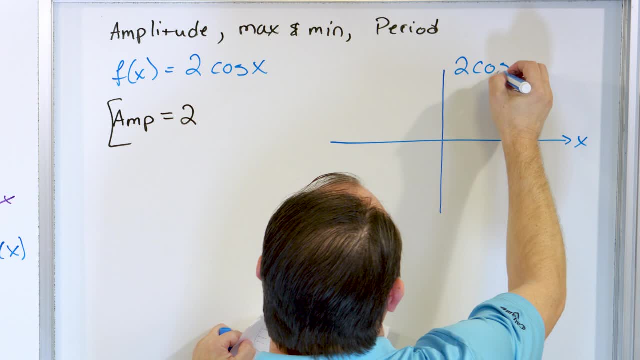 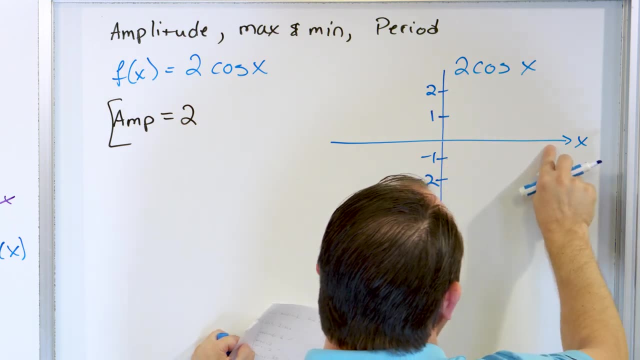 answer the question. So we have X and here's two times cosine of X. So what you can do is you could say: well, this is one, this is two, this is negative one, this is negative two. I don't care about putting every last thing on the graph. 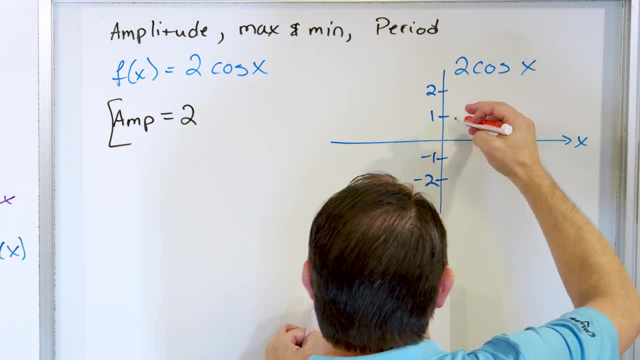 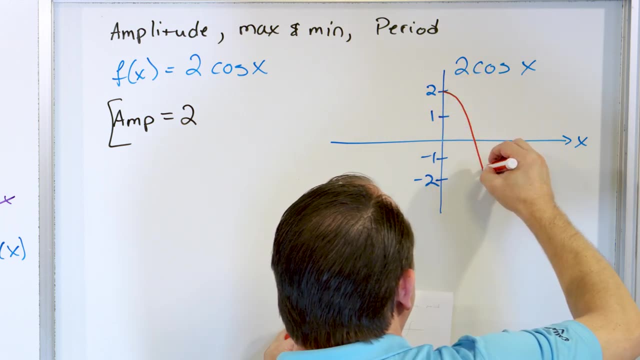 as far as like the numbers here, because ultimately you're gonna get tired of doing that, But basically a cosine starts at the top, whereas a sine starts at the origin. cosine starts at the top and then it goes down, in this case to negative two. 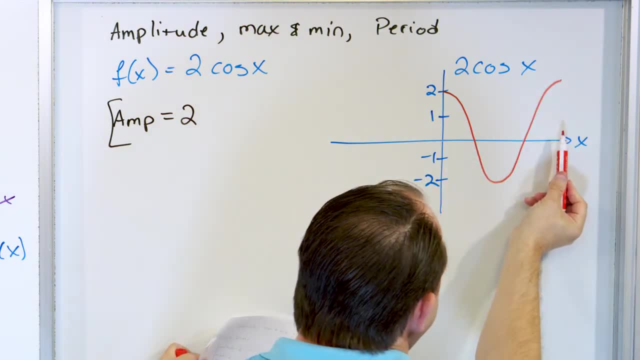 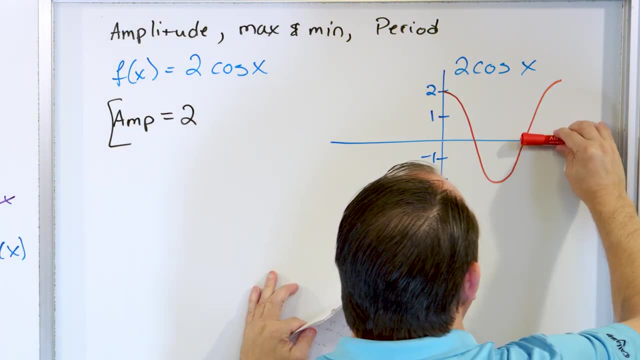 and it's gonna go back up again. The crossing points: of course you could fill them in, but after a while you don't need to because you're just doing this so you can answer the rest of the problem. The amplitude is two because that's the distance. 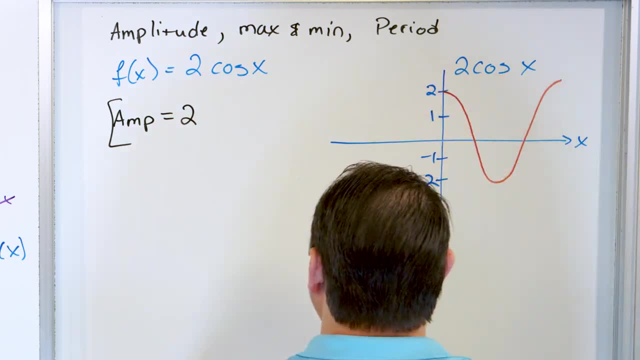 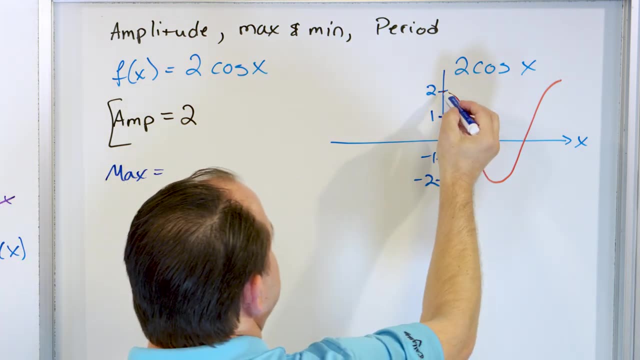 from the X axis up to the maximum, or yeah, to the maximum, of this function here. Now, what would be the maximum and minimum values? Well, the maximum value is positive two. The minimum value is what Negative two, that's what an amplitude is. 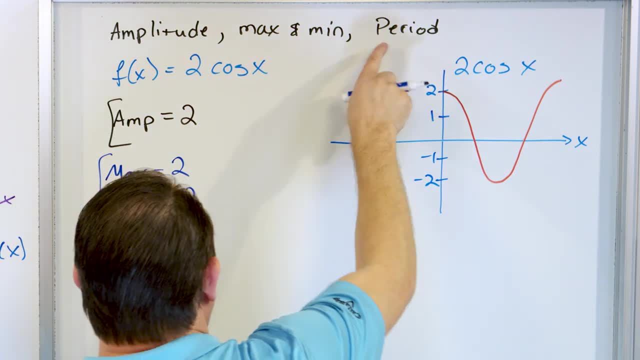 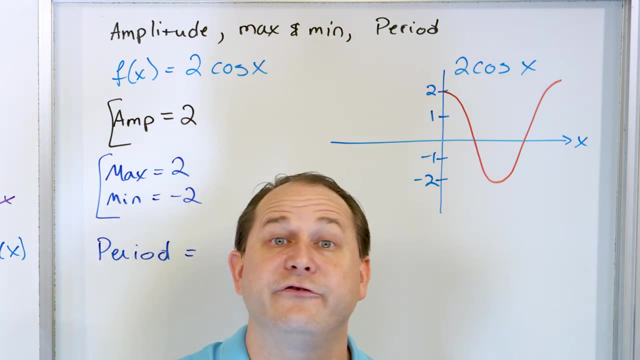 Maximum, minimum. it kind of defines it for you. And the last thing we wanna write down is the period. What is the period of this function? Well, the period of a basic cosine is two pi. What's the period of this one? 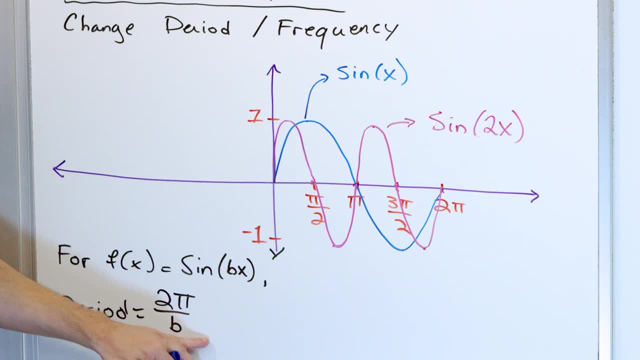 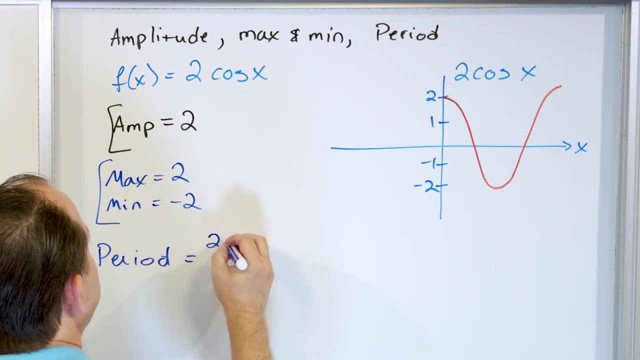 Remember we said it might be modified, So what I want you to do is start using this all the time. The period is two pi divided by B, where B is whatever number is in front of X. So the period is two pi divided by B. 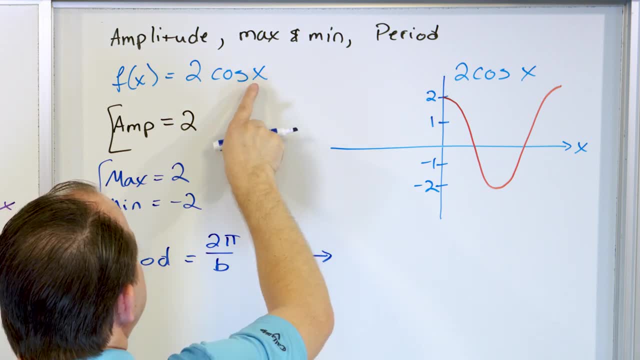 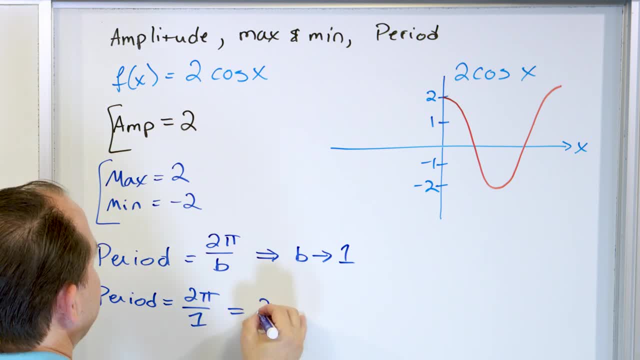 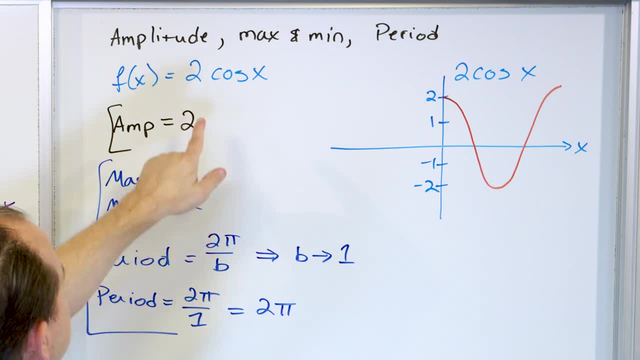 So the period is two pi. So we'll just circle this. If I had a, just for giggles, if I had two times the cosine of two X, where two X was in parentheses there, then I would at the same time be changing the amplitude. 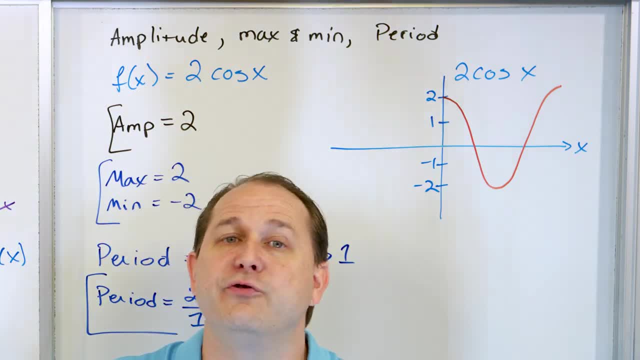 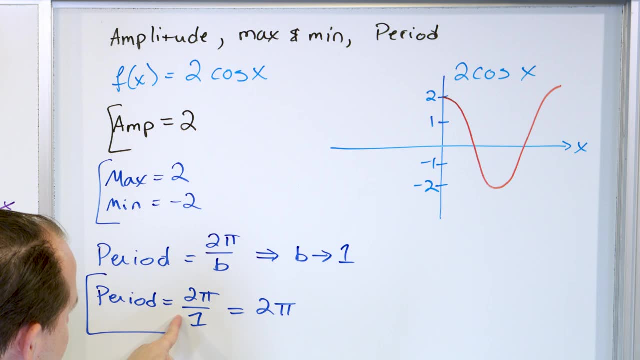 and I would be changing the frequency So you could do both at the same time, And so in that case the period would be: if there was a two in front, then it would be two. pi over two, B would be two. 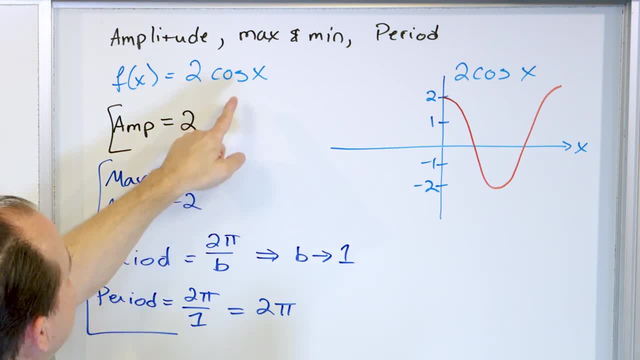 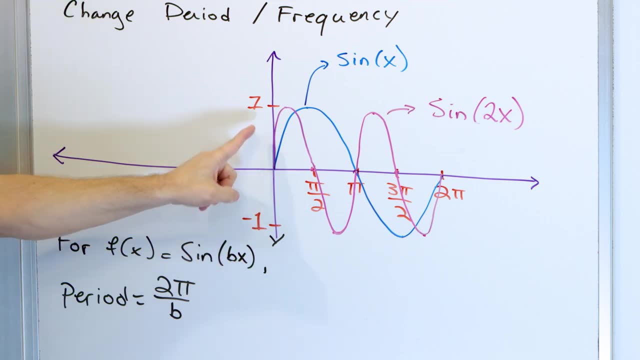 And then what basically be saying is: the original period is cut in half because I'm increasing the speed of the wiggles there. So two pi over two would be a period of pi, And that's exactly what we found in this example here, where the period was pi. 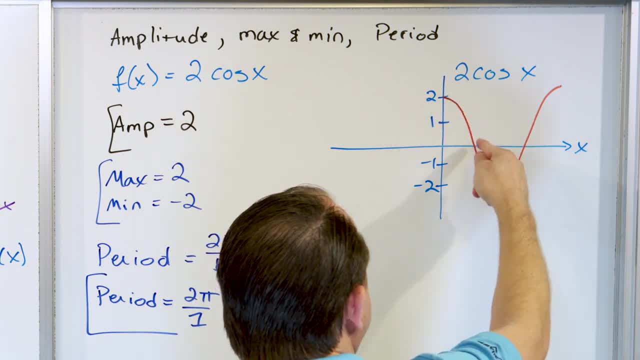 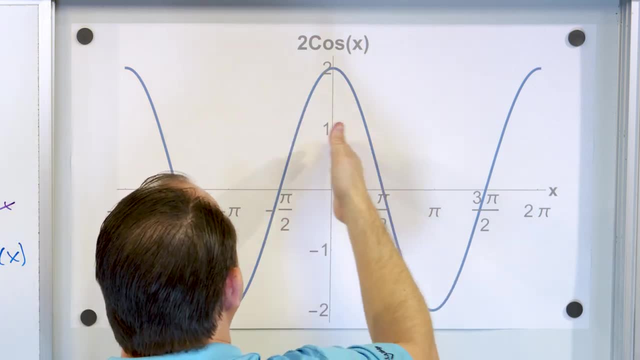 All right, Now just to close the loop. this is the little sketch we made. It goes up to two, down to negative two, And here is a prettier version of this: Two times cosine of X. This is drawn over some negative values. 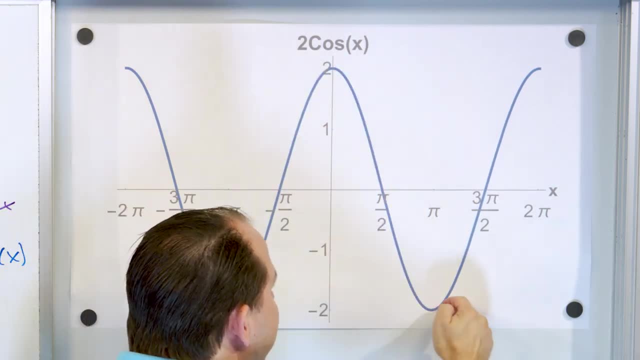 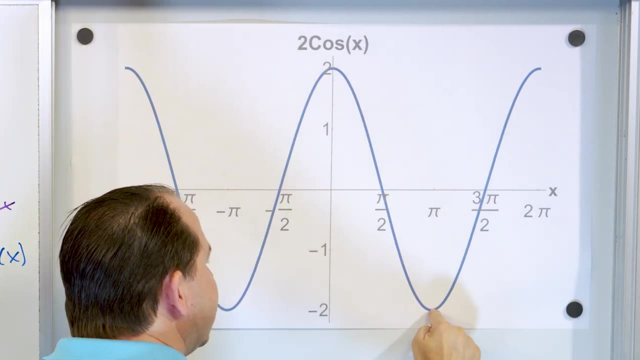 and some positive values so you can see Notice that it still has a period of two pi. So we said that's correct. But the only difference is it's starting at two and then going to negative two and then back up to the starting point. 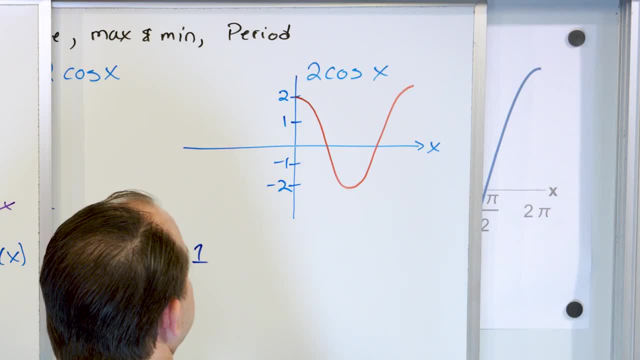 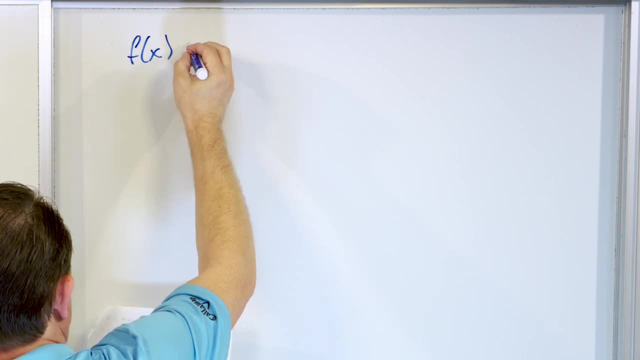 And, of course, the same thing is happening on the other side. All right, so let me erase this and we'll solve our next problem. All right, the next function we're gonna deal with. F of X is gonna be equal to sine of four X. 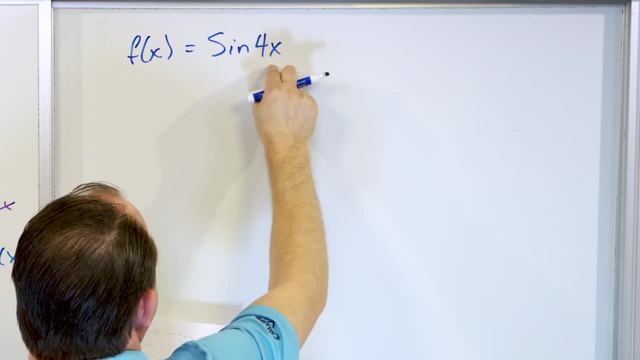 Now, when you write it like this, we know that both of these are together and the sine is operating on it, but you can be more clear by wrapping it in parentheses. So the first thing we wanna do is: let's try to sketch this. 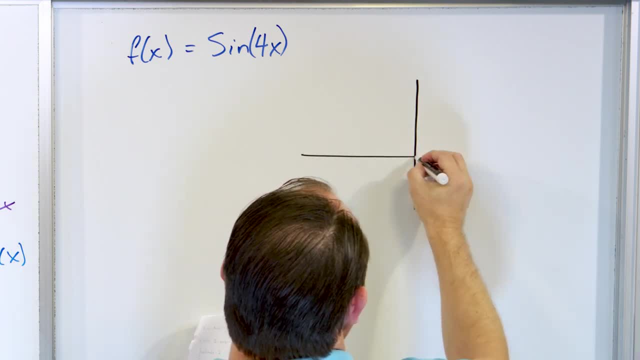 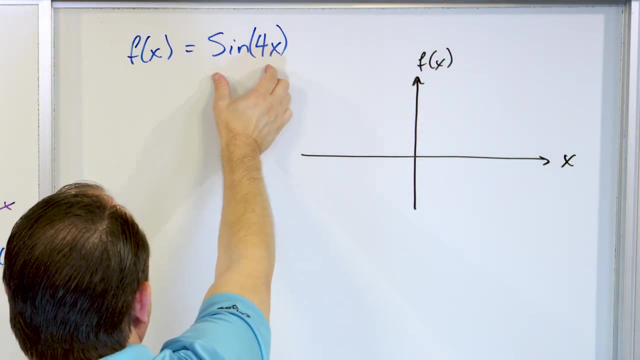 before we answer anything, because sketching it is very important and it can actually answer your questions. There's X, here's F of X. Now, this case we know. the only change to this thing- the amplitude has not changed- is we're changing the frequency. 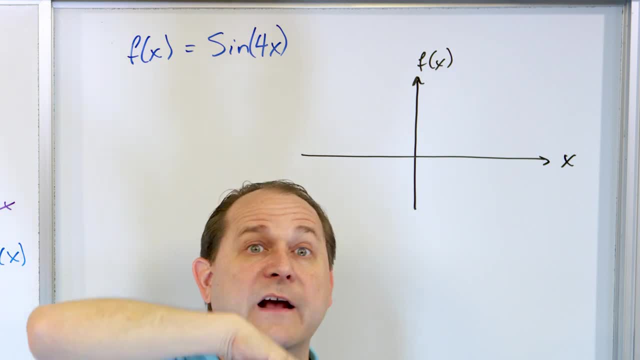 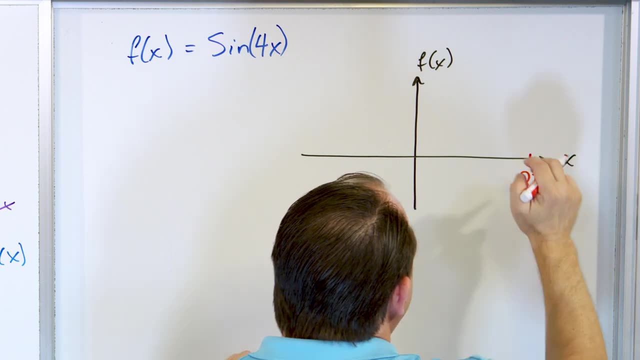 The number four inside of there is gonna make this thing oscillate four times faster than a normal sine function. And we know that in a, when X is equal to two pi, it's one cycle of the sine right, But this thing has to actually oscillate four times. 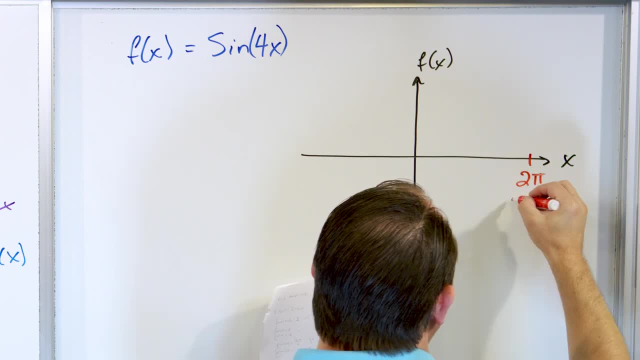 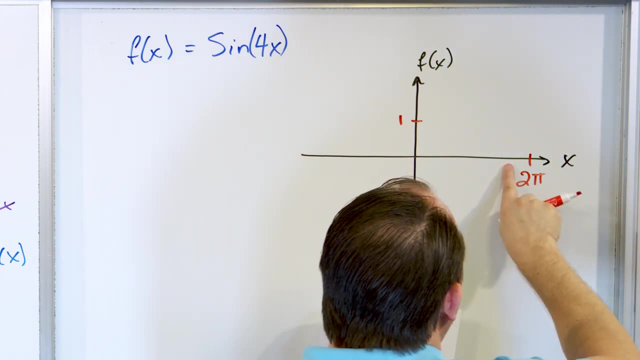 inside of the same window. A normal sine would just go up, then down, then up, but this has to make it four times. It's not gonna be beautiful. So I can't draw it perfectly, And I don't care about marking all the angles here either. 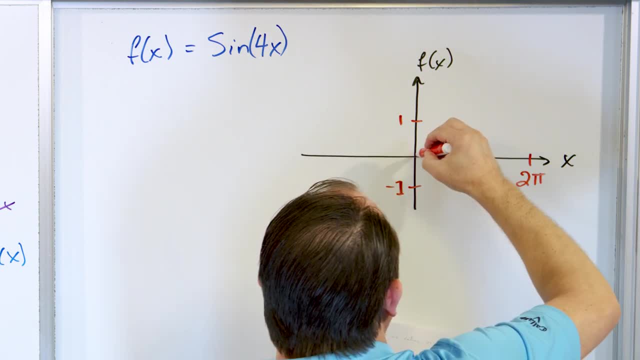 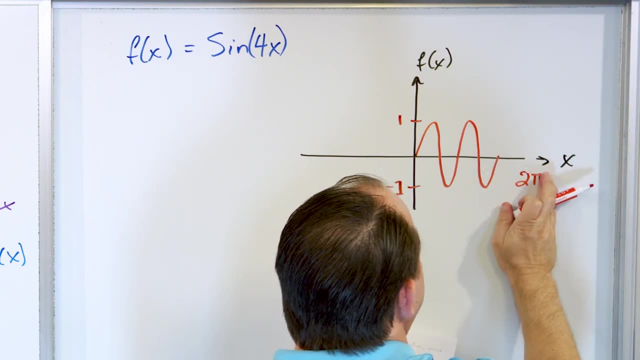 All I want you to know is that there's four of them that exist in this region. So here's like there's one, there's two, and see I'm not even gonna have room, So I'm just gonna erase this. 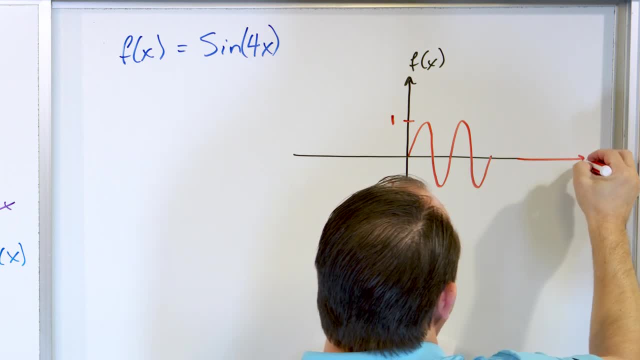 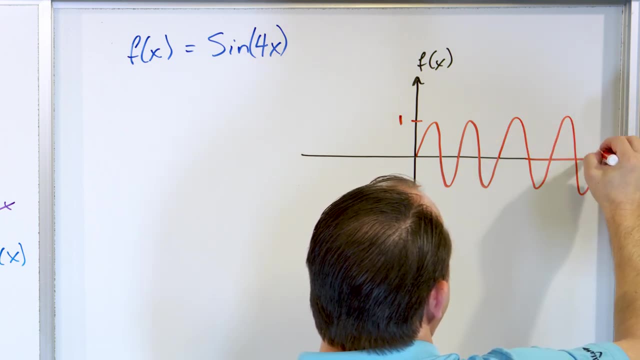 I can already tell I'm not gonna have room, So let's just extend this like this: Okay, there's two, And then it goes, here's another one, three and then here's four, And this spot here is two pi right. 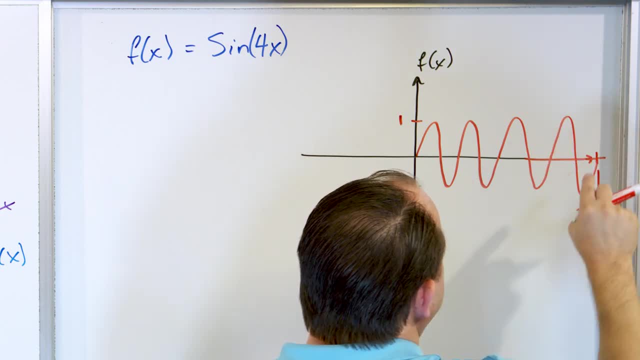 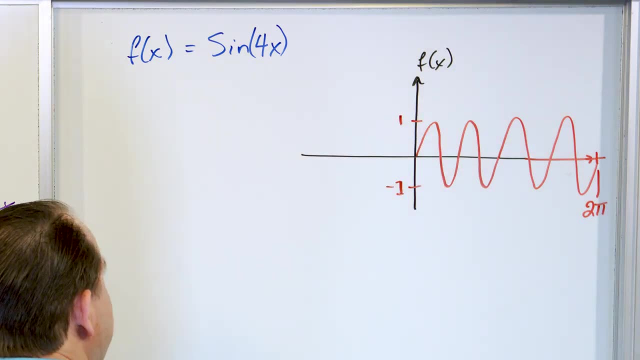 So we have to have one cycle, two cycles, three cycles, four cycles. Notice, my graph is terrible because I'm getting bigger here. It really should be exactly in there, But putting a sketch helps us visualize what's going on. because here the first thing I want you to write down. 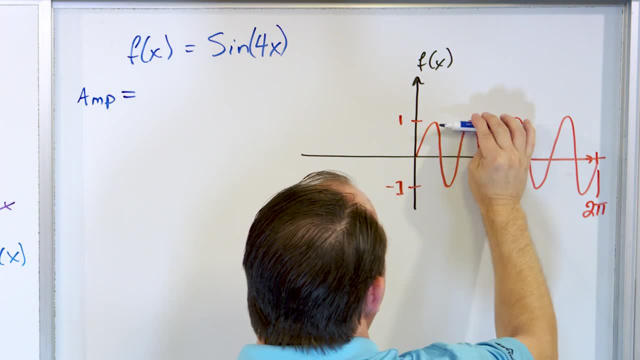 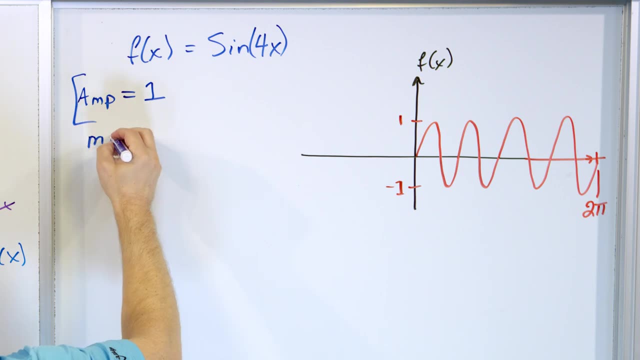 is, what is the amplitude of this function, That's, the distance from the x-axis up? Well, the amplitude is still one, because it only goes up to a plus one or a minus one. What is the maximum value of this function? Again, it goes up to a positive of one. 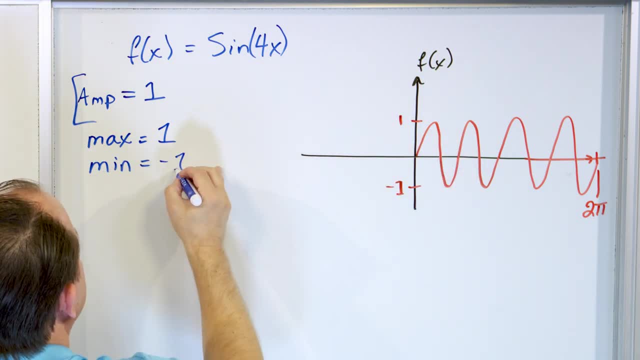 What is the minimum of this function? It goes down to a minimum of negative one. Okay, so we answer all the questions just by looking at our sketch. Now, what's the period? Well, what we do is we take the original period. 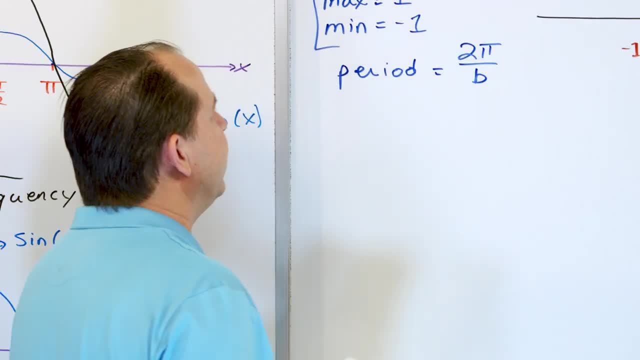 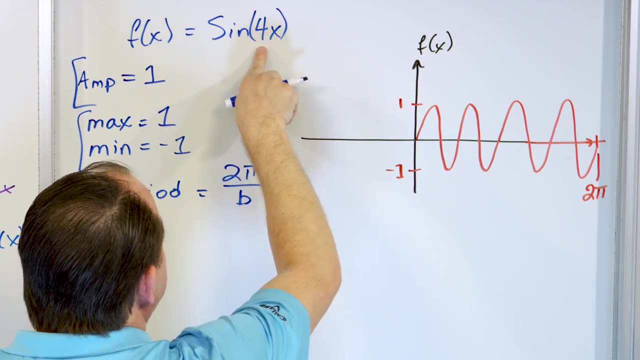 of a baseline sign, and then we divide it by whatever this factor is, And this is the same equation we wrote down on the board earlier. okay, This factor is whatever number it's like the speed multiplier in here. This means the thing is oscillating four times faster. 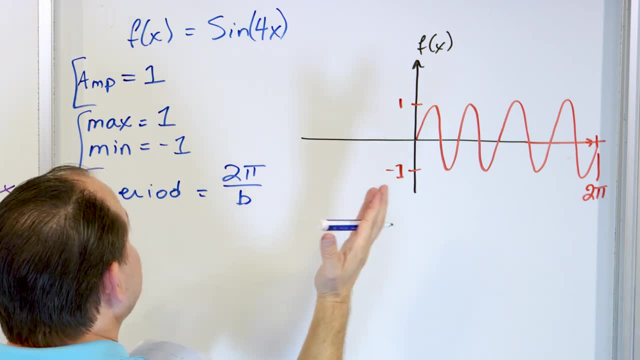 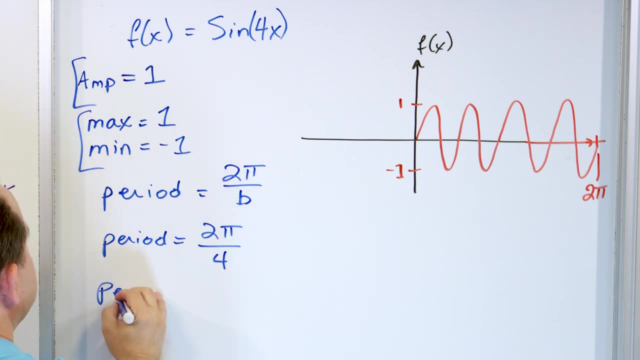 but it's the same thing as cutting down the period by four times the amount smaller. So the period is gonna be two pi divided by four. So the period is gonna be when you divide these out, or two divided by four is gonna be pi divided by two. 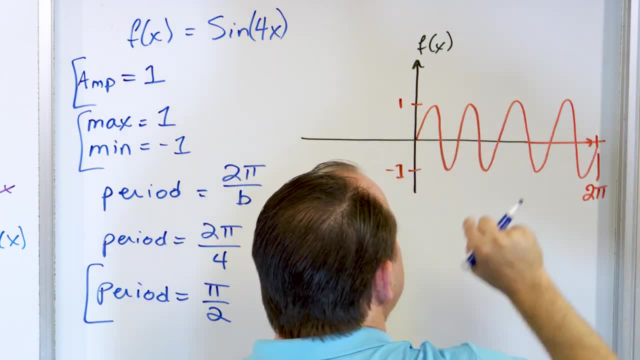 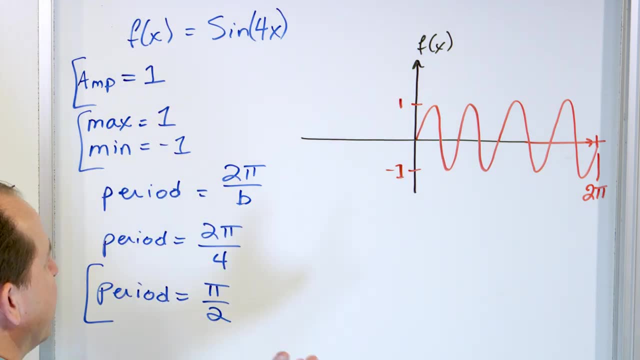 So, whereas a normal period of a sign actually oscillates over a two pi region, the period of this function is gonna oscillate four times faster, which means the period is four times smaller, only needing to go up to pi over two. What this is basically saying? 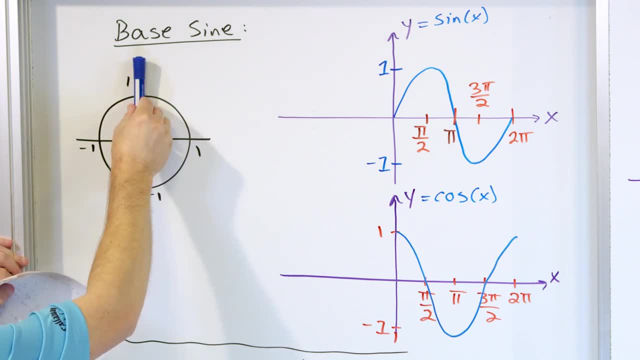 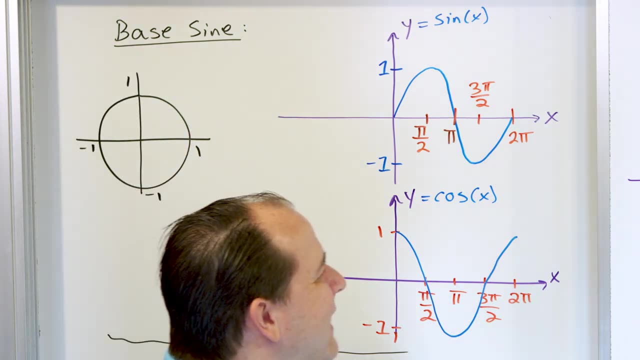 if you look at the unit circle, remember here's zero and here's pi over two. What it means is when the input variable X gets to here, right at pi over two as an input angle, what happens? What happens is when I put pi over two in here, times four. 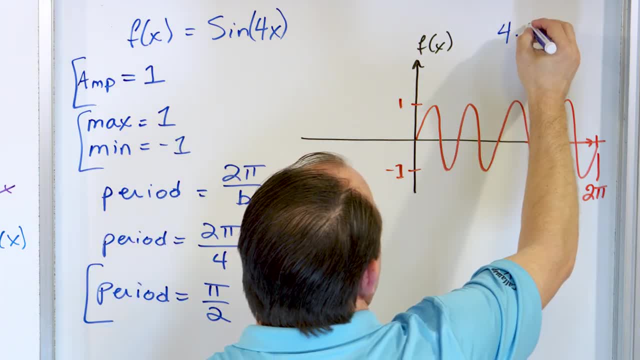 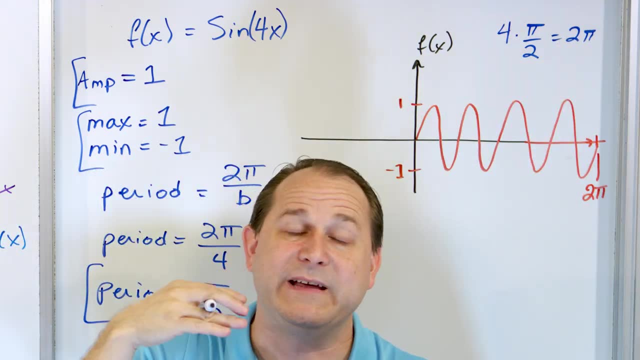 what I get is because if you just look at what four times pi over two is, you cancel these guys and you get two pi And then you have sine of two pi. So that means that when the X variable, the actual input, only goes one quarter of the way. 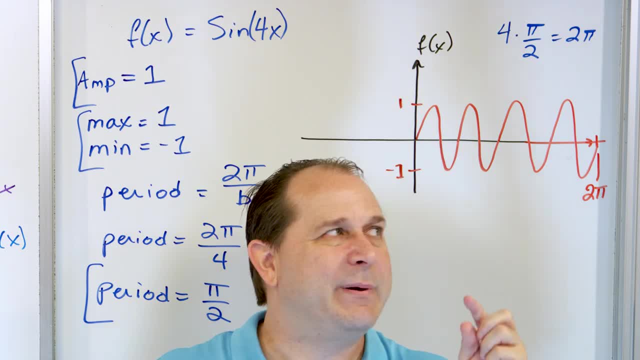 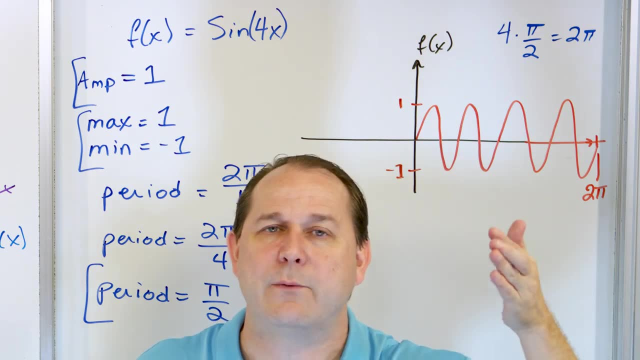 around the unit circle instead of all the way. then, because of the multiplication by four, I'm actually taking the sine of not pi over two. I'm taking the sine of four times that, which is two pi, which means I've gone all the way around. 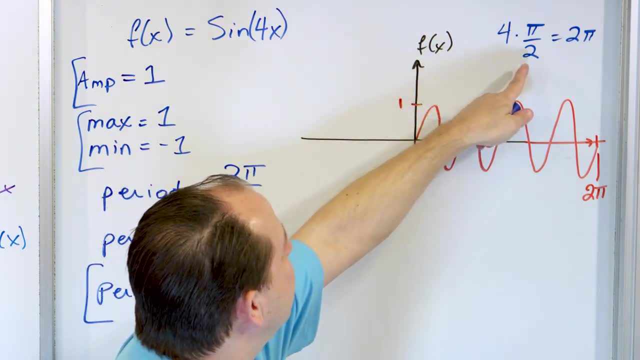 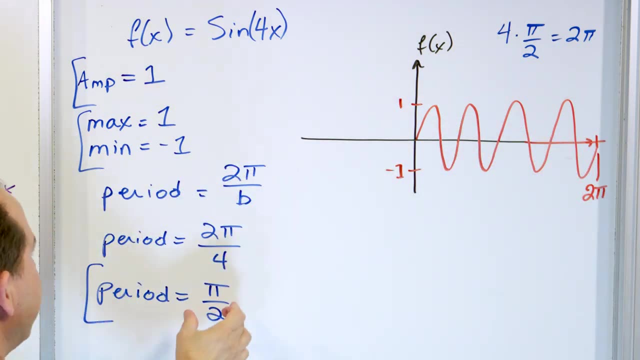 and completed one cycle of that sine function When my input only went to pi over two, which means it's a very small number and there's four sets of them in here. So I have four complete cycles there. So the period is pi over two. 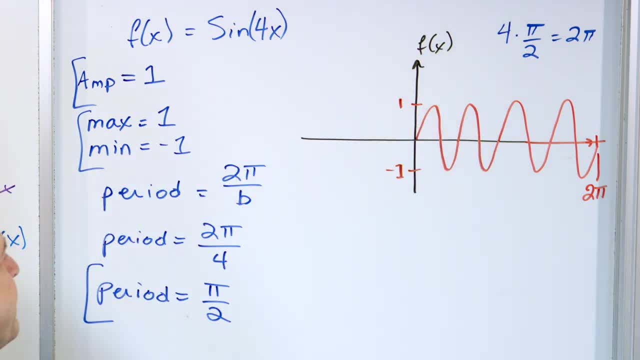 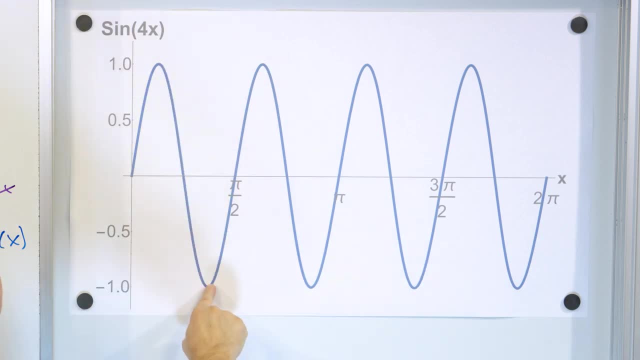 which means it begins to repeat after a much smaller time period. Now the very pretty graph here to show you sine of four times X would look like this: one sine of four times X. Again, it goes up to positive and negative one. 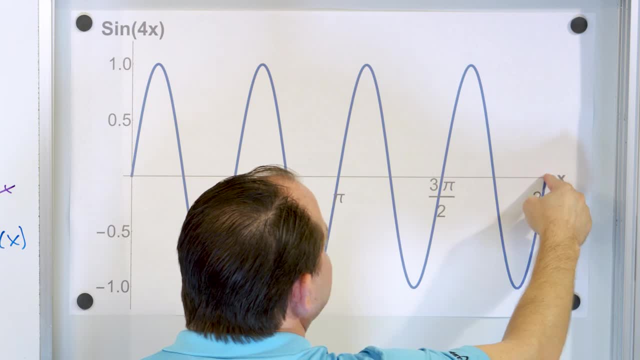 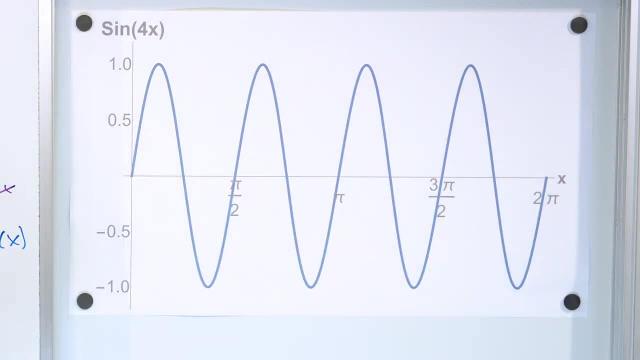 And the normal sine would just take one cycle all the way into pi. but here we have one, then we have two, then we have three and then we have four cycles existing in the same region of time. All right, let's take this down and solve our last problem. 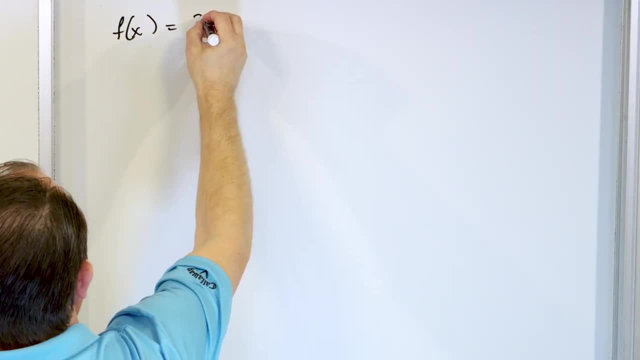 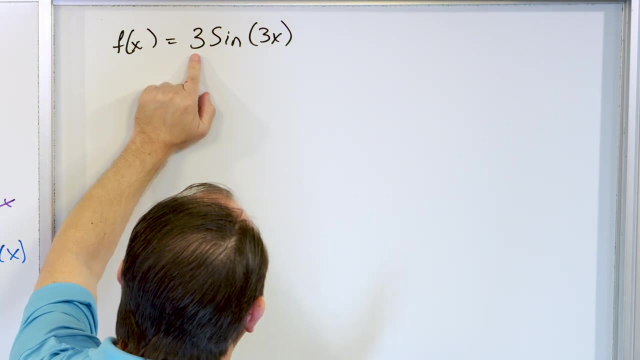 All right, let's take a look at our very last problem. F of X is three multiplied by the sine of three X. So here we have two things going on. The first thing is the amplitude is triple, which means it goes up to positive three. 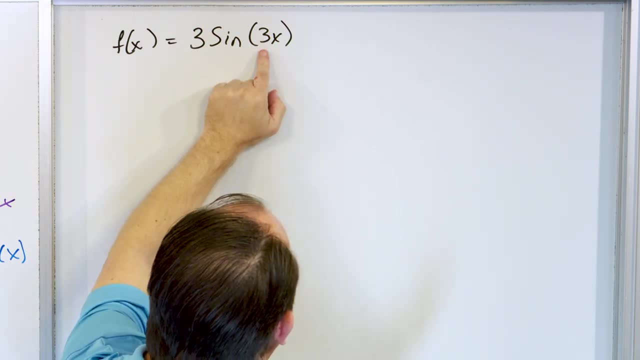 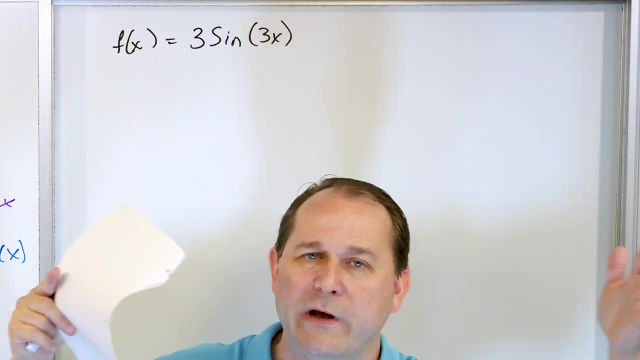 and down to negative three, And then, secondarily, the frequency is three times bigger, which means the period is three times smaller, which means there's three times the wiggles in a normal window for sine. So before we answer any questions, 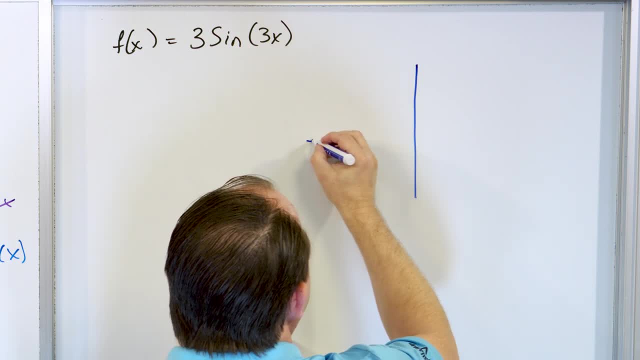 it's just gonna be easier to just draw a little sketch And you don't have to put all the angles down. Now a lot of people don't wanna do the sketch because they don't want to draw the angles, but that's okay. 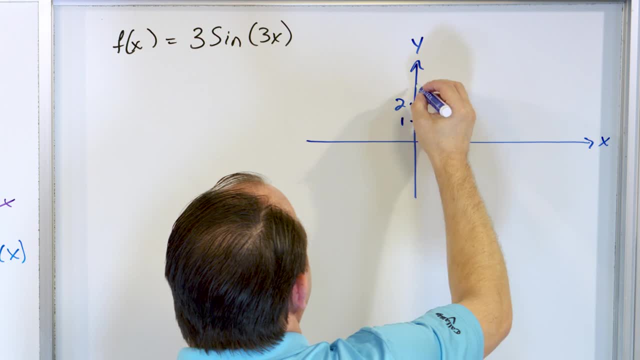 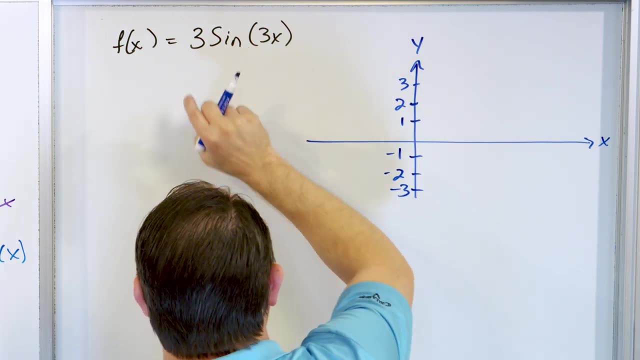 Just put: here's a. we could say this is one, two and this is three, and this is negative one, negative two, negative three right here, Because what we know is this thing has a three in front, So we know it's gonna go and it's a sine. 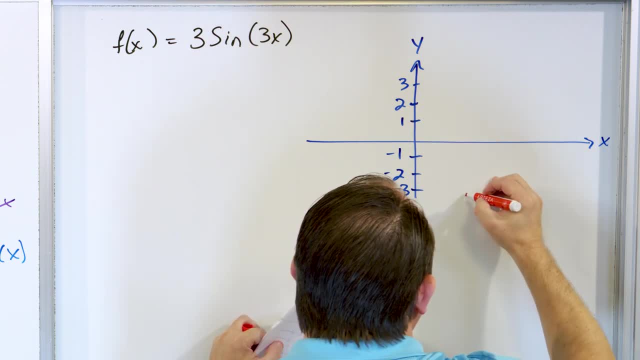 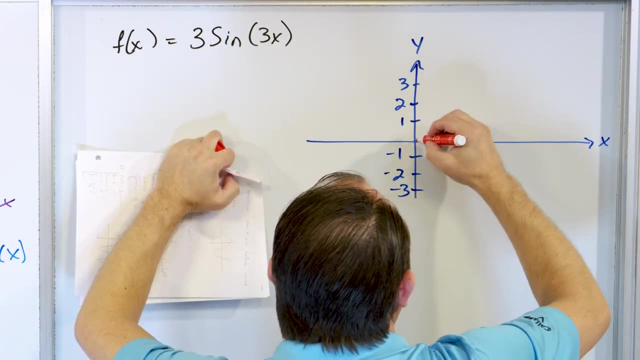 which means it starts from here, it's gonna go up and then it's gonna go down to a negative three and then up. But there's gonna be three of these cycles in a two pi region of x here. So it's gonna go up here, then down here. 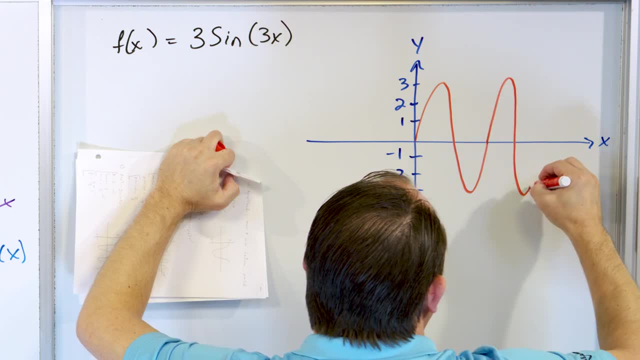 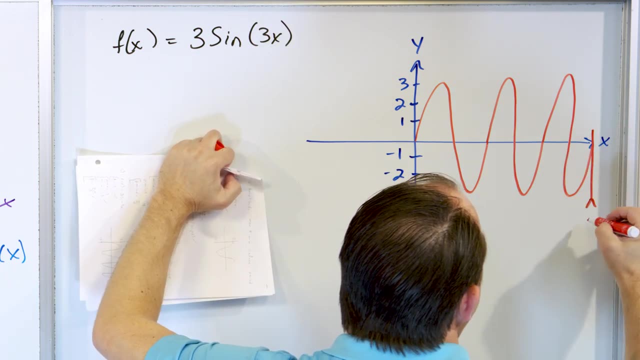 That's one cycle, Then it's gonna go up and then down and then up. That's another cycle, Then it's gonna go up and then down and then up another cycle. And this angle right here is two pi. 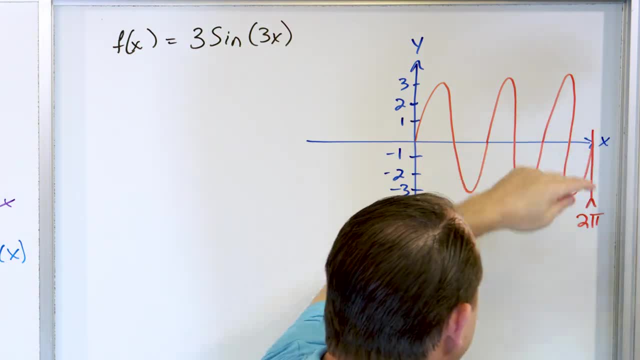 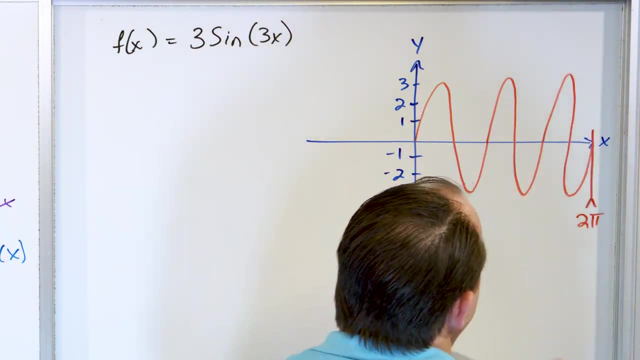 Sorry about the. the end of it here is just not great the way I ran out of space. But you get the idea. There's one cycle, then there's another cycle, then there's another cycle. There's three cycles in a normal baseline window. 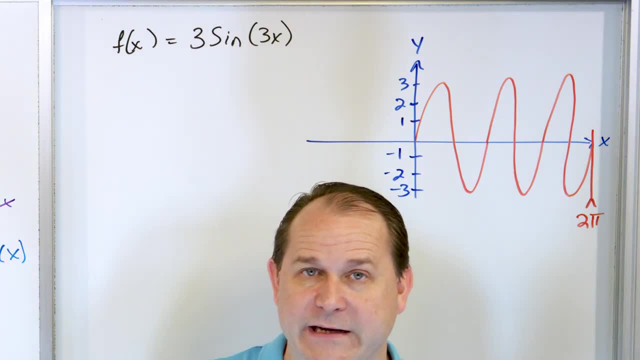 That's why, again, I was telling you, for all these trig functions, you have to have a baseline in your mind. Two pi is the period. okay Any modification to that, we can easily draw it and we don't have to mark all these angles. 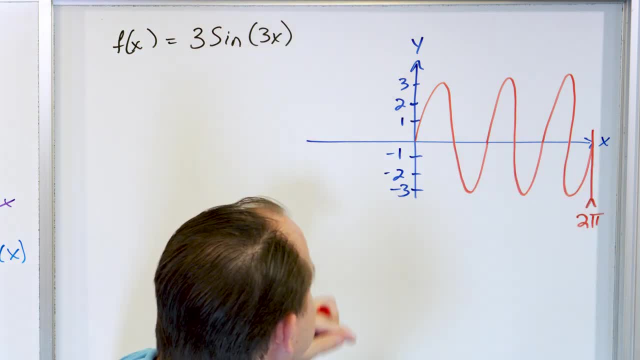 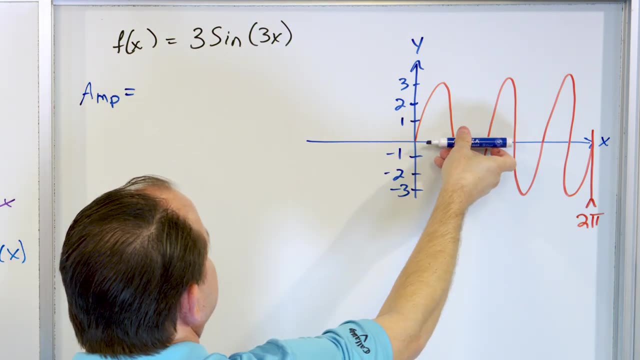 That's okay. All we know is three cycles fit into this window and it goes up to plus three, down to minus three. And assuming all of this is true, what is the amplitude? Well, the amplitude is the distance here up to there. 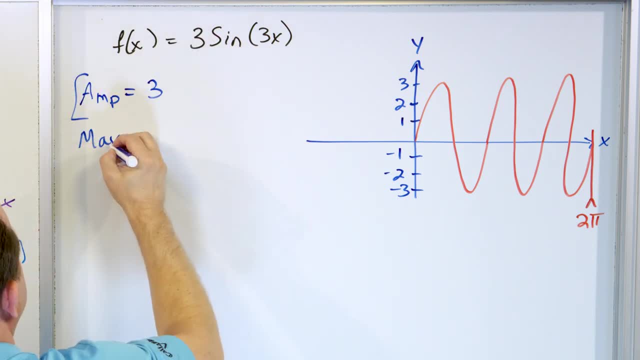 So the amplitude is three. What is the maximum? The maximum again goes to three. What is the minimum? The minimum goes down to minus three. okay, So that's an answer there. What is the period? Well, the period is two pi. 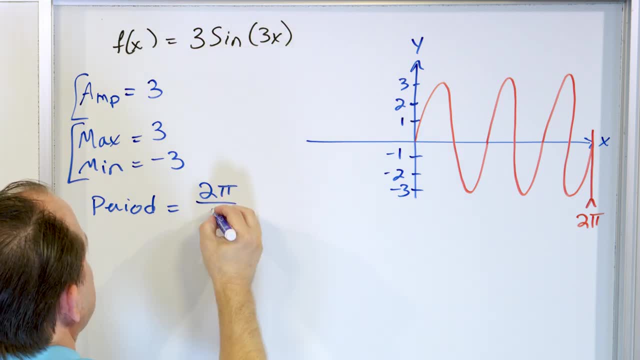 which is the original period of assigned function divided by the scaling factor three. It has to be smaller because this three means we're doing more wiggles, So we're cutting the period down. We're saying that in a normal two pi period window. 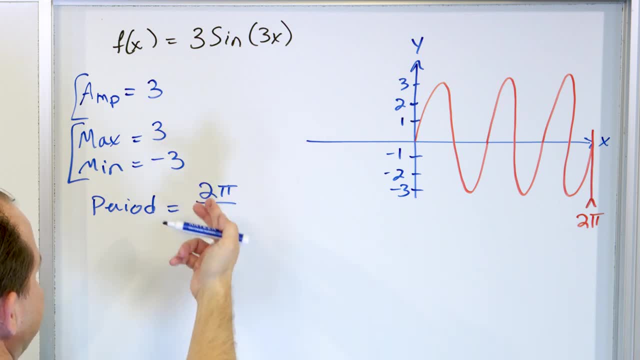 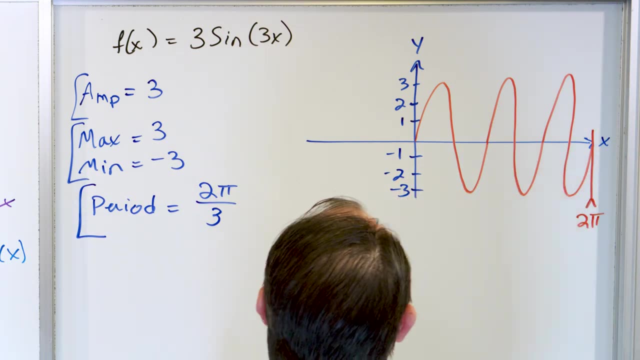 is cut into three equal pieces. That's what we're doing. We don't have anything to simplify. The period is just two pi over three. Now, this is my sketch. It's terrible, but this is the kind of thing you would do on your sheet of paper. 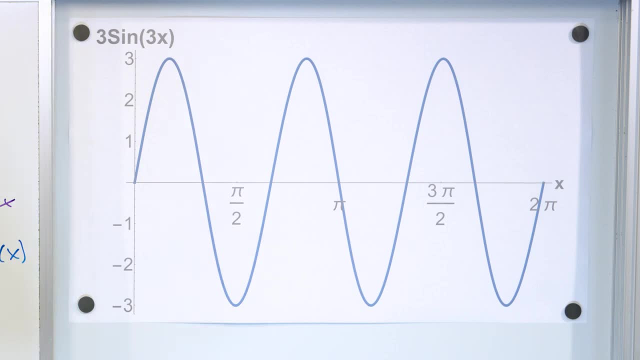 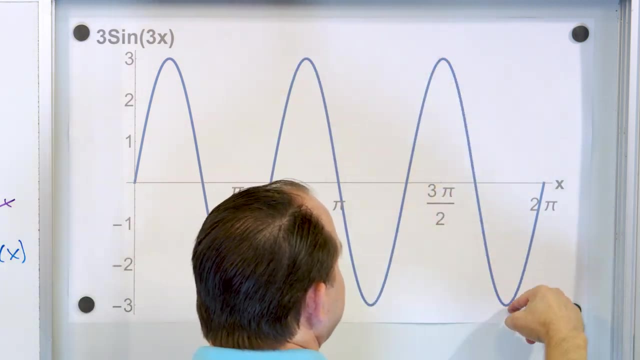 Let's see what the real sketch would look like, And it would look like something like this: It would go up to three, down to minus three. Here's one cycle, Up then down, then up. There's two, Up, then down, then up. 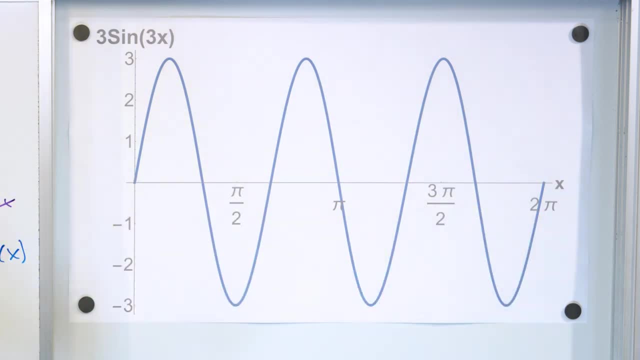 There's three. There's three complete cycles in a two pi window of a normal sine function That takes care of this, and then it goes up to three and down to minus three. So that's what we're doing here, That's all correct. 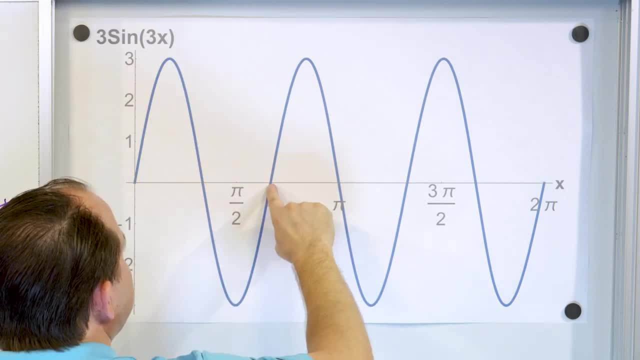 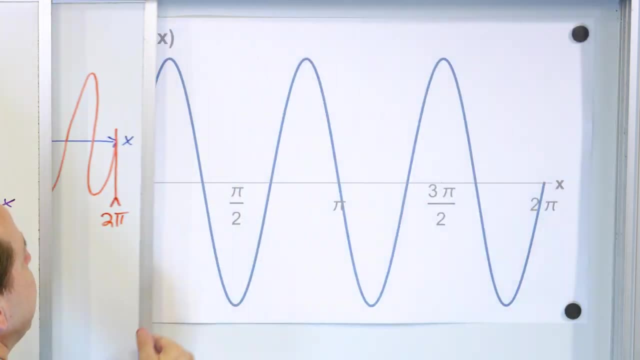 Now, what is the period of this thing? Notice that here is two pi and the period it begins to start over here. The period that we calculated was two pi over three, So I just didn't put the granularity in the graph here. 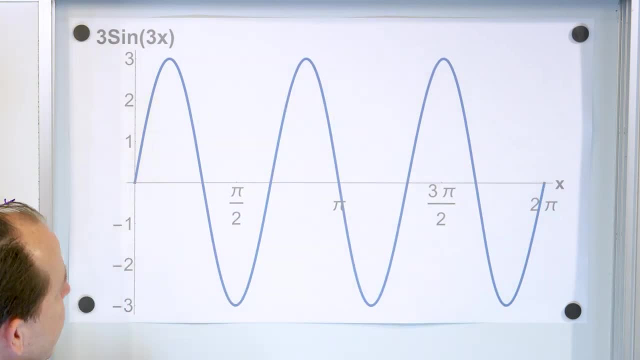 the labels, the tick marks, but this is two pi over three, And we know mathematically that's what it is, And so I guess, if you were gonna graph it perfectly, you would just put that on there. In fact, you could. 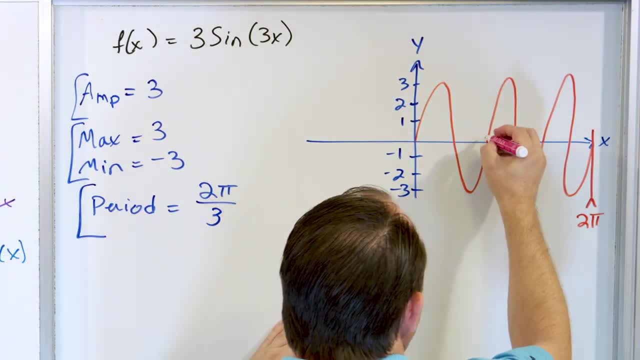 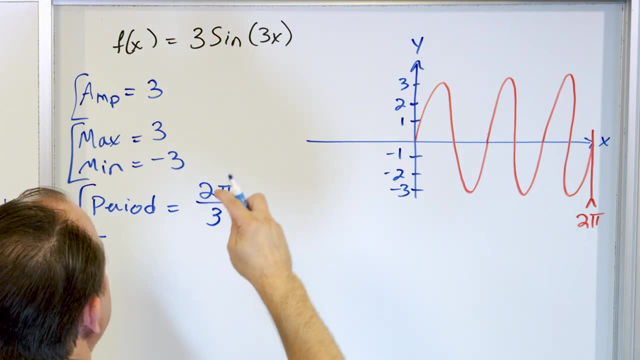 since you know the period is two pi over three, you could just mark it right here. Just put a little tick mark and put two pi over three, and that's what it has to be. And why. why is the period two pi over three? 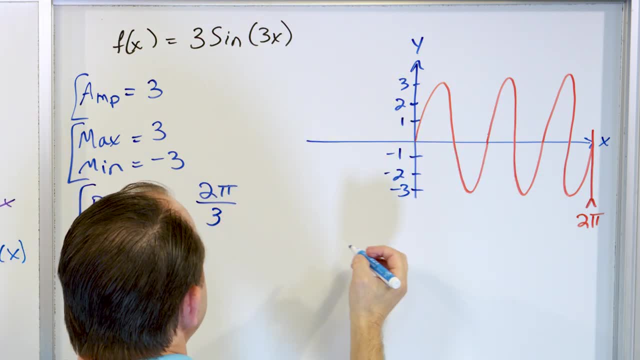 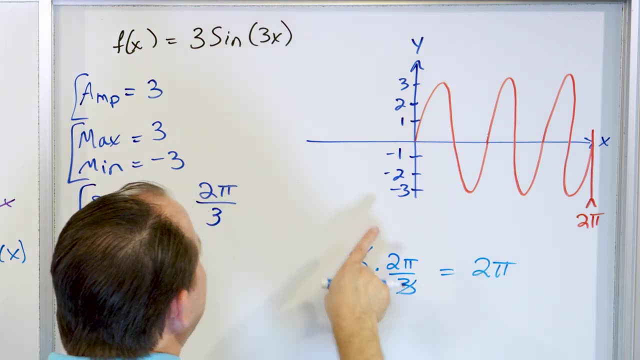 Because if I put an input value for x of two pi over three, then it's gonna be three times two pi over three, But the threes will cancel and then that'll be two pi. So when I stick an input value of two pi over three, 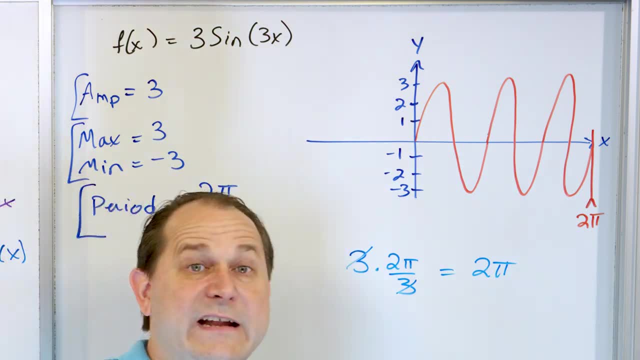 what I'm really taking the sine of is actually two pi, which means that it's gone around one time and has just completed one cycle at that moment. That's why the period is what it is. So I do want you to remember. 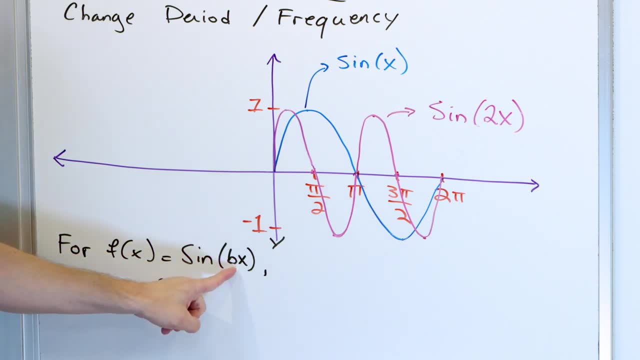 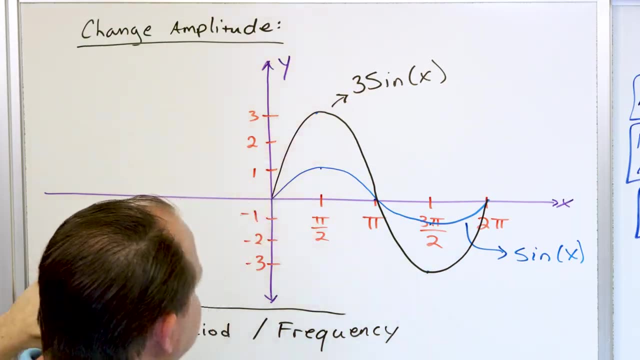 that the period of a sine function is two pi divided by b, where b is whatever is in front of here. I do want you to remember that changing the number in the front of the sine changes the amplitude. And I do want you to remember 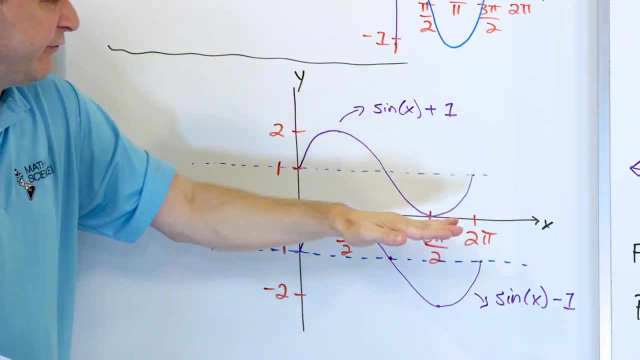 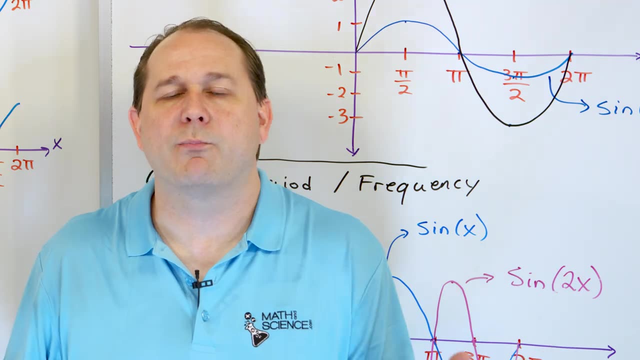 that adding or subtracting a number on the outside of a sine function just shifts the whole thing up and down. What we're gonna do in the next two or three lessons is just more of the same. We're just gonna get more practice with it. 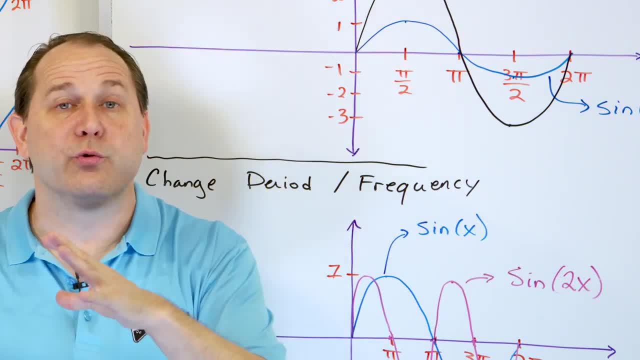 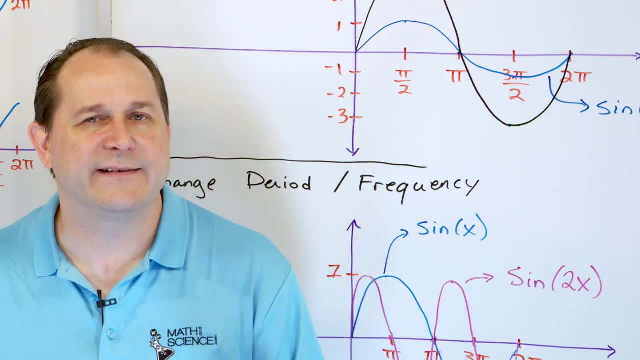 We're gonna do sometimes doing one thing at a time. sometimes we'll do two or three things at a time And after a while you will get comfortable with what these different things do, because I couldn't really break this lesson into three lessons. 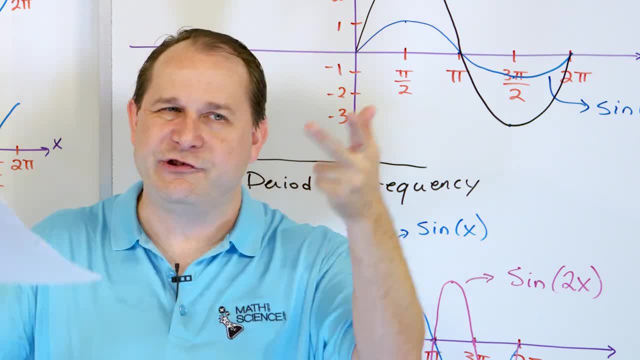 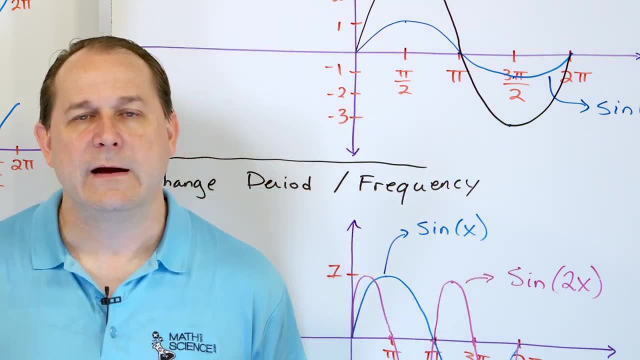 one on amplitude, one on frequency period and the other one on shifting. I mean, I could have, but it wouldn't have really done much, because you really have to see them together to know how they differ from each other, And so it's a long lesson. 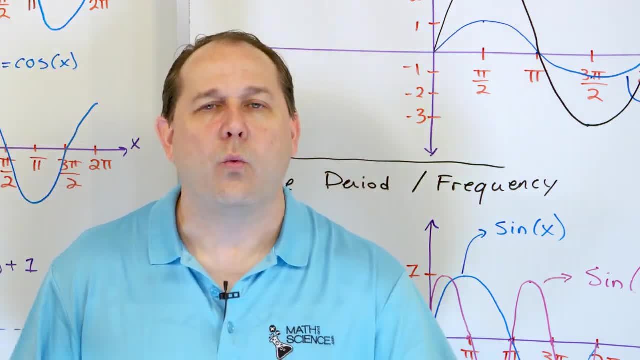 I apologize, but that's just the way it is. I also encourage you to sketch. Watch this lesson again. I've done lots of sketching, even in the lecture. I didn't have to. I'm doing it for a reason.